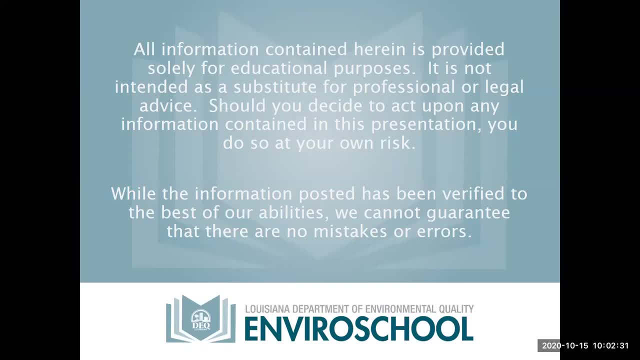 Slides and a recording of this webinar will be available on the EnviroSchool website. There will be a poll at the end of this webinar to provide your feedback so we can improve our sessions. so please complete before logging off. If you have any comments, questions or concerns, please email me at enviroschool. 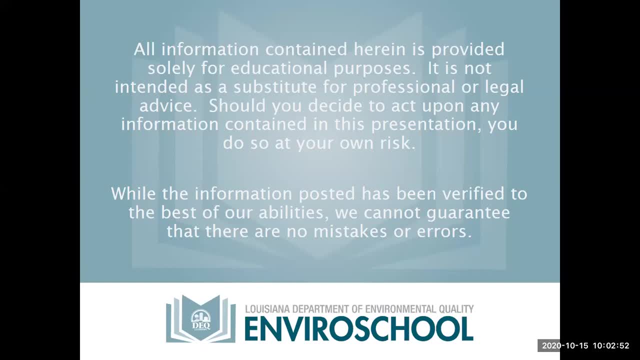 at lagov. Also, there's a note in the chat that if you would like a certificate of participation afterwards, please email me at enviroschool as well. Our speaker today is Keith Horn. Keith has a bachelor's and master's degree in conservation and biology from Southeastern Oklahoma State University and the University of Louisiana Monroe. 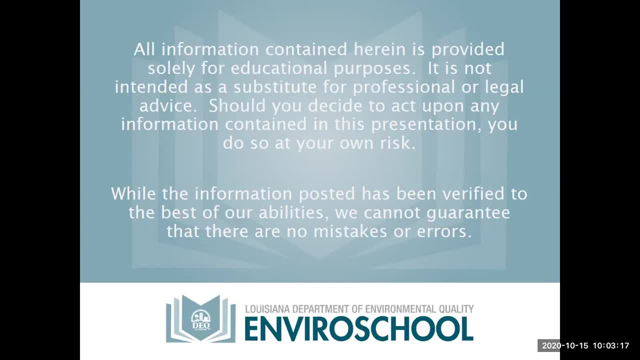 Keith is currently serving as a senior environmental scientist in the Remedio District. Keith is currently serving as a senior environmental scientist in the Remedio District. Keith is currently serving as a senior environmental scientist in the Remedio District Mediation Division here at LDEQ, Following a period of working for the United States Fish and 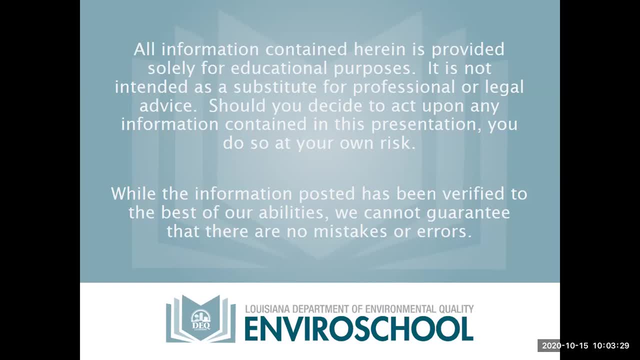 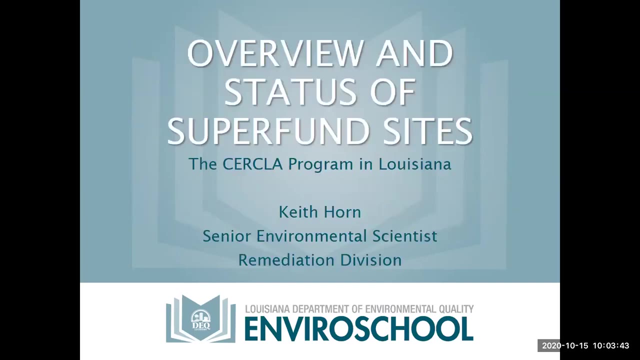 Wildlife Service. he began his career here in 1992.. Keith has 28 years of experience in site investigation and assessment, remediation and related areas. Keith, please begin. Thank you, Tamika. Like Tamika said, I'm Keith Horn and I've been around for a long time As. 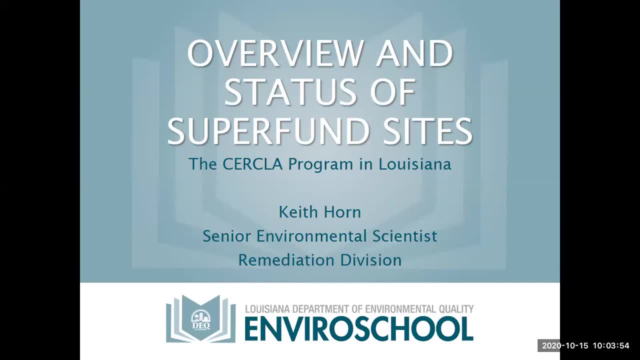 you can see I like to joke that Edwin Edwards and I started the same day and that's just that is true, but it is a coincidence. nothing to do with Mr Edwards, But anyway I am. one of my roles at DEQ is to be coordinator for our Superfund program in Louisiana. 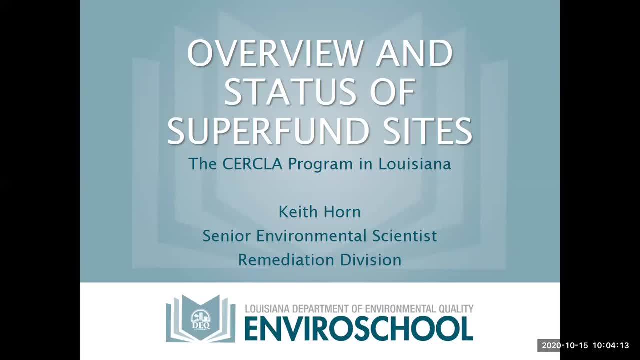 and for those of you that are unaware of the Superfund program, it is properly known as CERCLA, and we'll talk about what that means. It's a federal program and here in Louisiana the Remediation Division of DEQ interfaces with 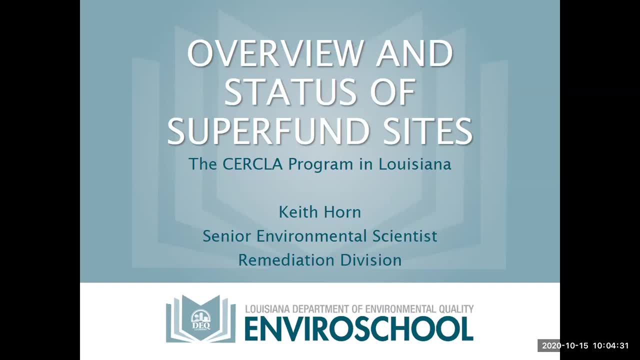 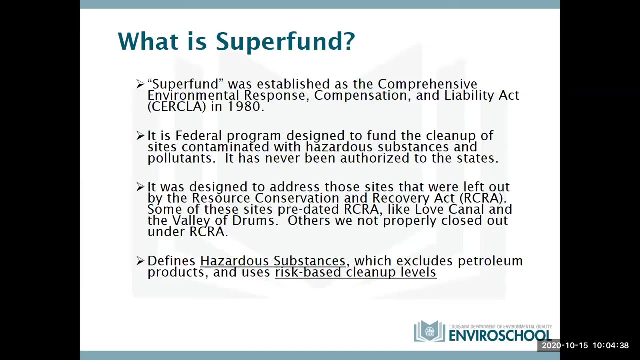 the US EPA, to you know, administer the CERCLA program and to deal with it. So all right, next slide, All right. so I guess we need to first talk about what is Superfund or CERCLA. and, as we said, it is was established by the federal law, which is known as the Comprehensive. 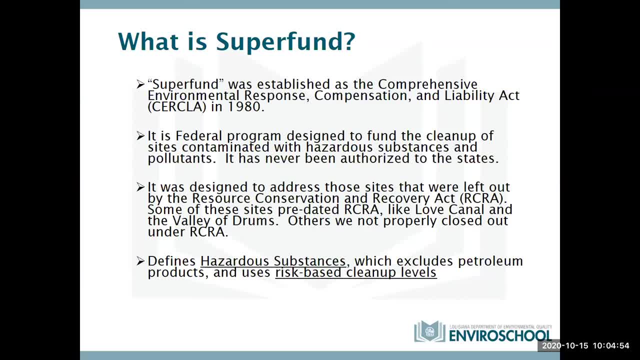 Environmental Response Compensation and Liability Act, and this was passed in 1980. So CERCLA is the acronym for that. Now important terms to get out of this legislation. it's supposed to be Comprehensive Environmental Response, and that's good. It is a very comprehensive environmental. 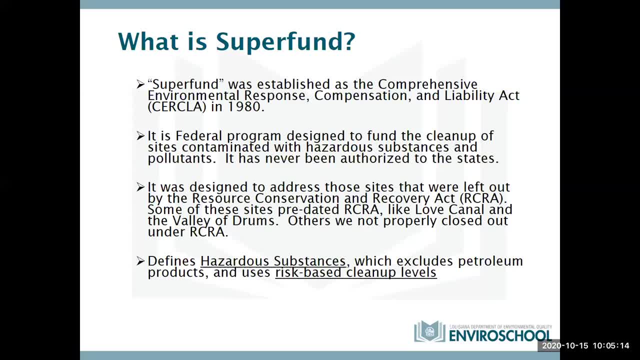 program, but two of the things that we're going to talk about today are the CERCLA program and the one of the key things that makes CERCLA, or Superfund, work are the last parts, which is the compensation and liability. The C and L in CERCLA are very important and have driven a great deal. 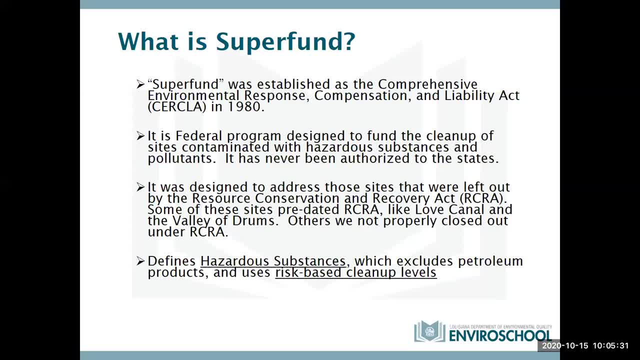 of environmental action in Louisiana and throughout the country, really. So let's look at this a little more. We'll move on to the next point. It is a oh no, sorry, Tamika, go back. Okay, the next bullet point. It is: 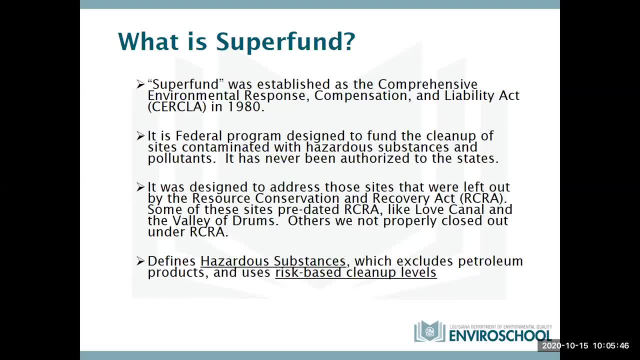 a federal program which is designed to fund the cleanup of sites contaminated with hazardous substances and pollutants, and it has never been authorized to the state. Now that term hazardous substance is important and pollutants is included in CERCLA and it's as I mentioned. 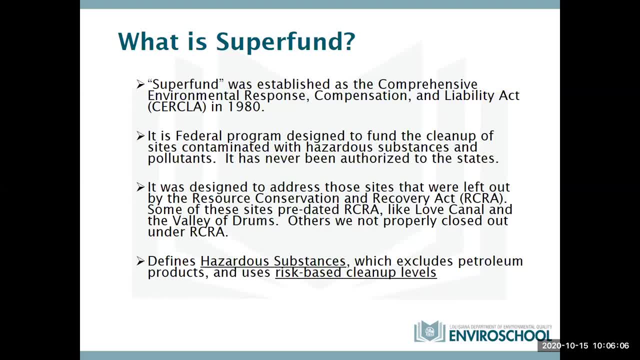 a federal program. You know, RCRA is authorized by the state. the DEQ administers RCRA because we have an authorized program. There is no such thing for CERCLA. We are the only EPA administer CERCLA Now. we are certainly partners with EPA, but it's their program. 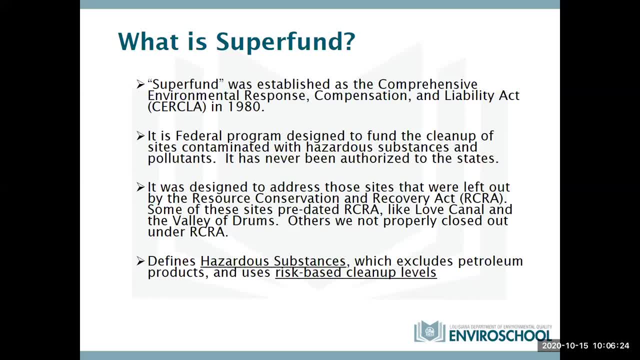 They make the final decisions, and they do so in consultation with us, but we don't run this show, So all right. So what was CERCLA for? Well, it was designed to address those sites that were left out by the Resource Conservation Recovery Act, That's RCRA. You may know it as the Hazardous. 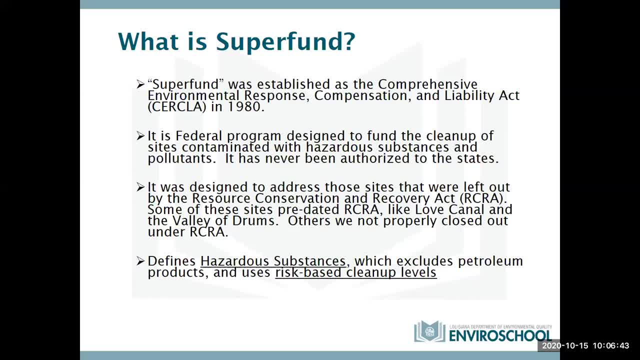 Waste Law and Hazardous Waste Regulations. Some of the sites that CERCLA was intended to address predated RCRA, So they were already there before RCRA defined hazardous waste and how you could dispose of it. Some of the most famous ones: 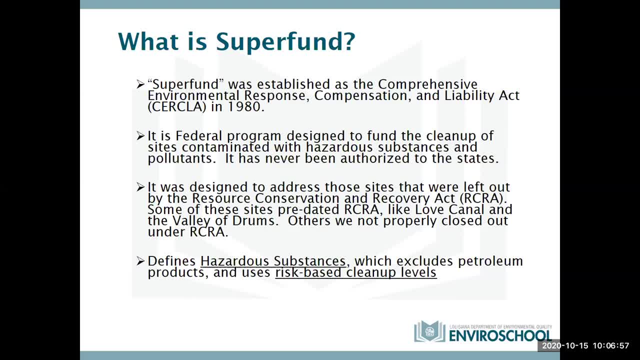 of course are Love Canal and then the Valley of the Drums. Then others were not properly closed out under RCRA. We have a number of sites in Louisiana where in theory RCRA was the law of land but in practice these sites did not achieve a program. So we have a number of sites that are 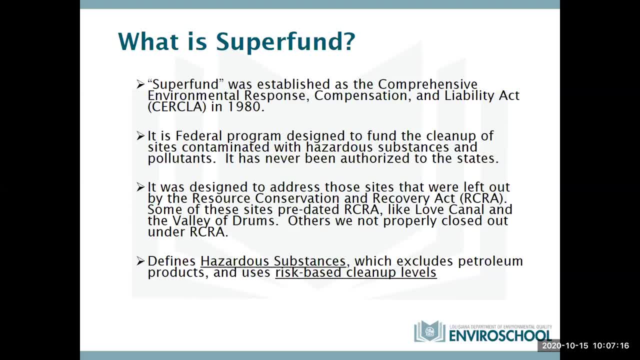 under proper RCRA closure and they ended up becoming CERCLA or Superfund sites. What Superfund does? at least as far as the law you know? RCRA defines hazardous waste. It tells you what is hazardous waste and where you can dispose of it and where you can't dispose of it. 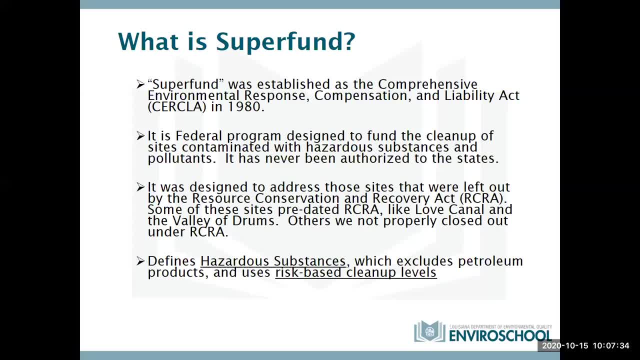 CERCLA defines hazardous substances and that's an important definition. Now, hazardous substances under CERCLA excludes petroleum, So hydrocarbons are not hazardous substances in the eyes of EPA and of CERCLA. Now in the state regulation that's not exactly true because our definition is different, but under CERCLA, CERCLA 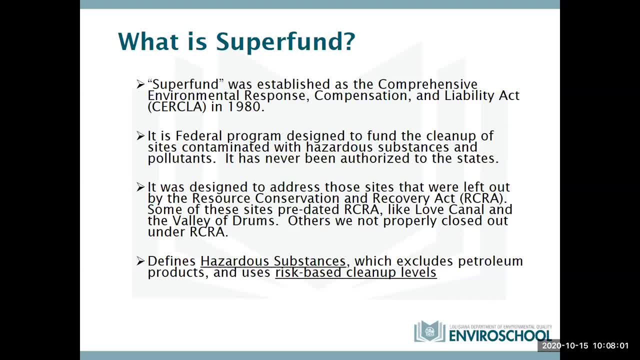 does not see or clean up hydrocarbons. They're just not part of the law. They were excluded from law specifically. Now, the other thing that CERCLA or Superfund did is it uses risk-based corrective action programs. Now, this is another critically important point about CERCLA, because we 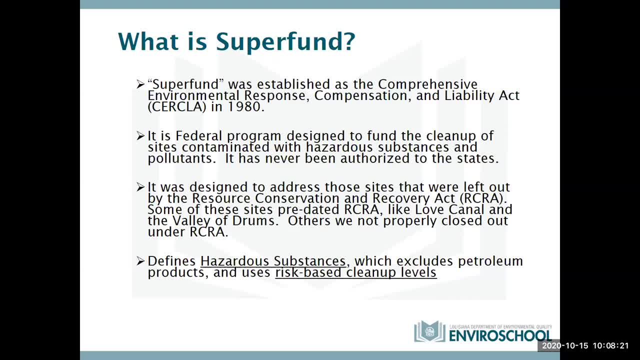 all have our risk-based corrective action programs. or here in Louisiana, we have the RECAP, which is the- you know, Risk Evaluation Corrective Action Program. Texas has its program, Arkansas has a program, Everybody has a program. Well, all these probabilistic risk assessment programs. 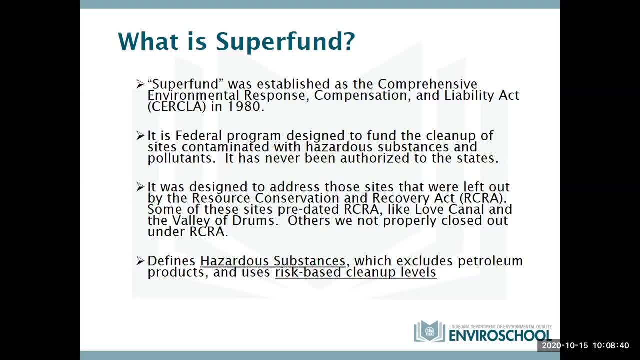 came from CERCLA because the question was, you know, Superfund program had all these sites that contaminated with hazardous substances and the question was, when cleaning them up, how clean is clean? That was the question. That's a big concept, So probabilistic risk assessment that we all use. 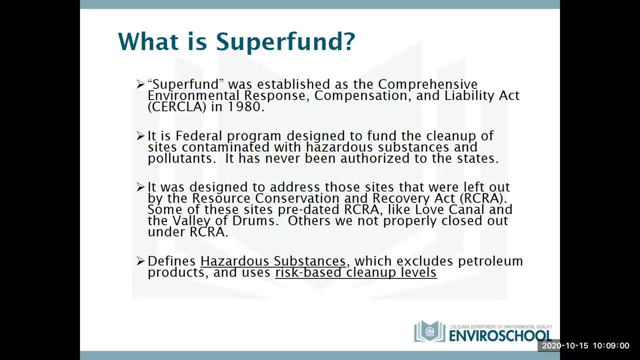 today came from the Superfund program. It came from CERCLA. It originally started in what was called RAGS, which is Risk Assessment Guidance for Superfund, and then RAGS evolved and then from RAGS and the various calculations, it became CERCLA. So it's a big concept. It's a big concept. 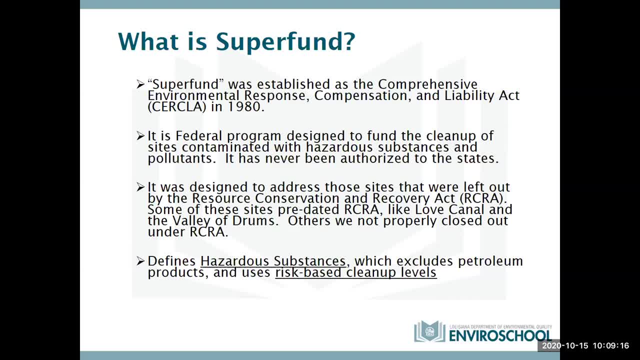 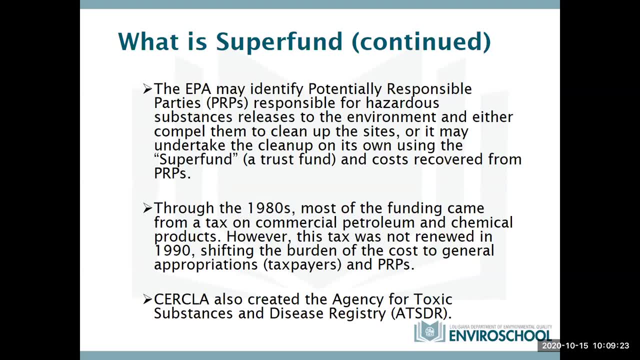 We all developed our various state programs, So risk-based cleanups came from Superfund. Okay to me, All right. So let's talk about Superfund a little more and how it works Under Superfund, the EPA. you know that compensation liability part- this is where it's very important The EPA may identify. 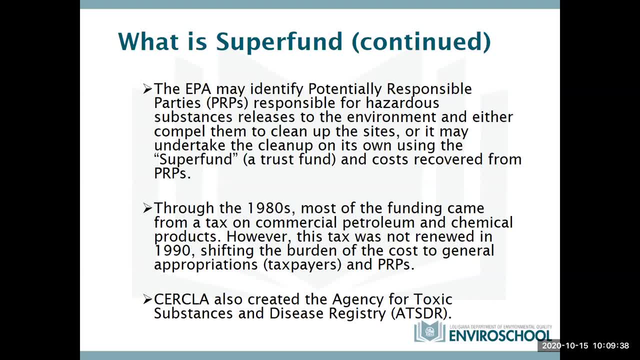 potentially responsible parties. These are PRPs. They are responsible for hazardous substances released to the industry. They are responsible for the production of hazardous substances. The EPA may take the program at the site out of the environment and they may compel them to clean up. 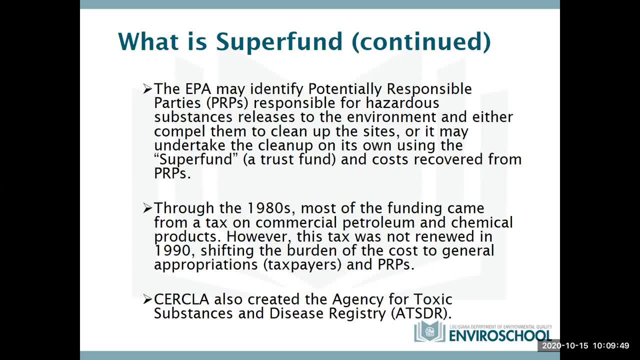 sites or may undertake the clean-up on its own using the Superfund, which is a trust fund- That's where the term Superfund came from- and costs recovered from the PRPs. Another scary thing about that liability, and early on in the program, is if the PRPs refused to clean up a site and then 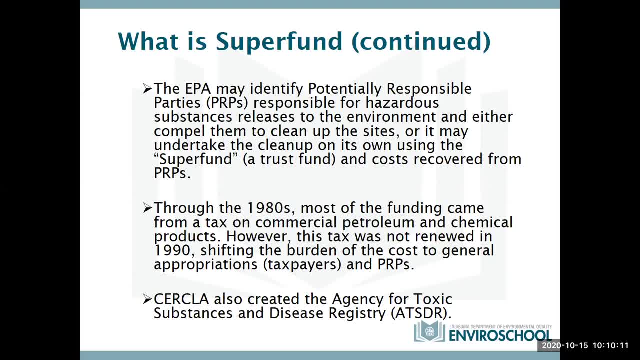 EPA used the trust fund or, you know, federal monies to clean up the site the EPA would have. they could then sue the PRPs in federal court and recover what's called triple damages, That is, from each PRP they would recover three times what the PRP should have paid to clean up the. 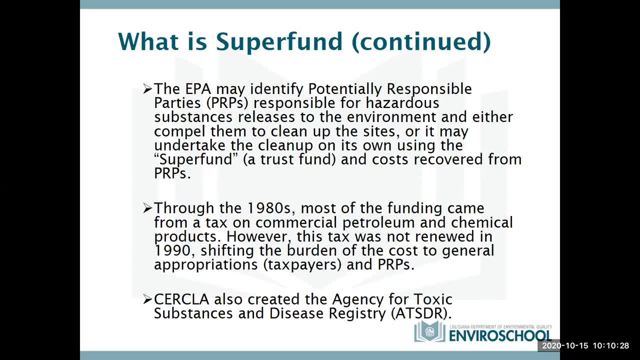 site in the eyes of the court. So that was a powerful motivational tool. They could always threaten to: hey, PRPs, if you don't play ball, we're going to go in and take care of the problem and then we're going to go and get your money. So that compensation liability part. 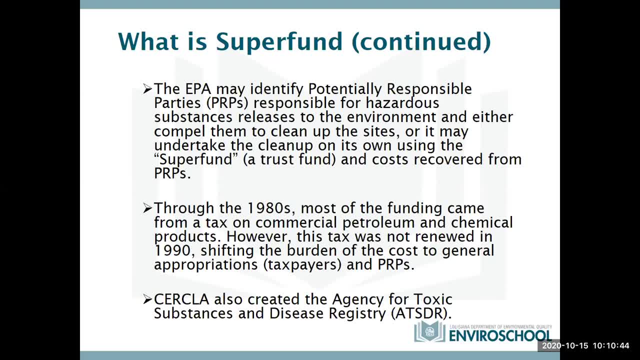 I told you is very important. Okay, so the second point on this page is: throughout the 1980s, most of the funding from Superfund came from a tax on commercial petroleum and chemical products. However, this tax was not renewed in 1990.. So the tax was originally passed with the Superfund. 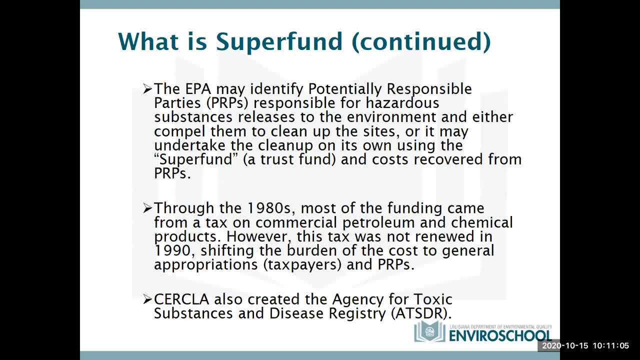 regulation in the 1980s- 1980, when the law became, you know, the law of the land, and then it had renewables, So the tax was not renewed in 1990.. So the idea of the Superfund tax was that the polluters paid. 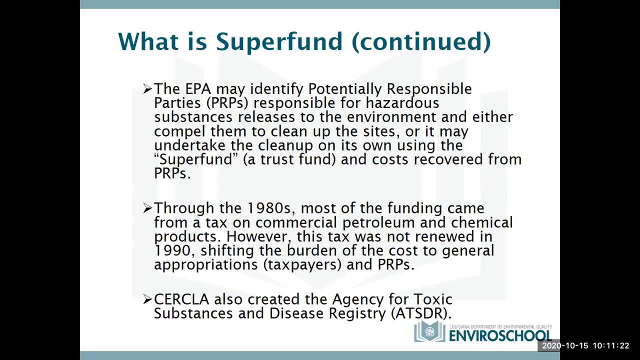 Well, that was, I guess, true, you know, although it was a tax on all chemical industries, you know, not just the ones that were responsible for certain sites, although many of them were responsible for some sites. So, but after 1990, the tax was not renewed, So the tax was not renewed. 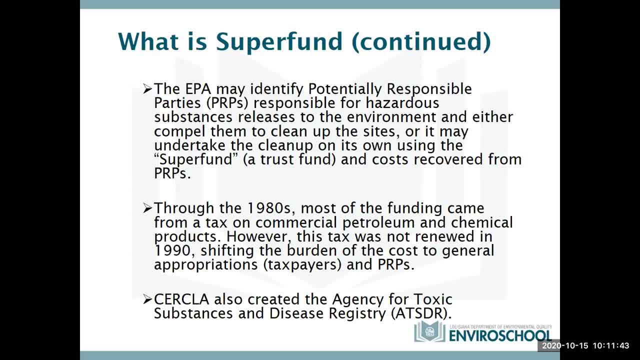 So the tax was not renewed. So the Superfund went on budget. So we went from the polluters paying to the taxpayers paying. So it comes from the general fund, Although- keep in mind the PRPs- the liability provisions still exist. So wherever possible, you know, EPA tries to identify those PRPs and make the polluters clean. 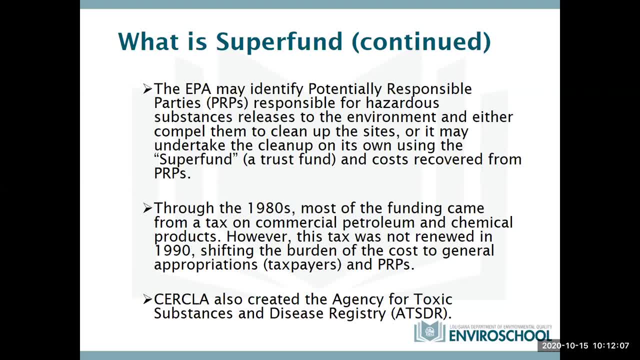 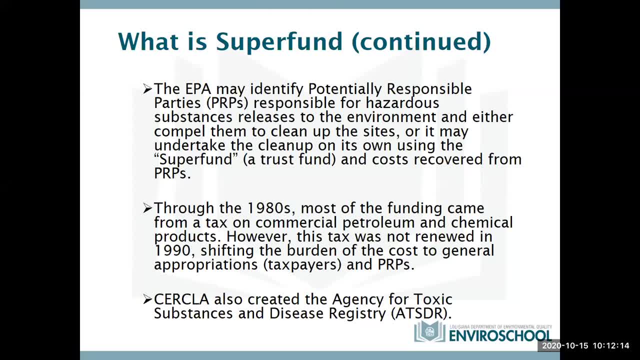 to be able to do that. We're not going to be able to do that. We're not going to be able to do that. Everyone has either went bankrupt long ago or whatever. So the federal government and the state government have to, you know, cover the cost of the remediation of the orphan sites, if you 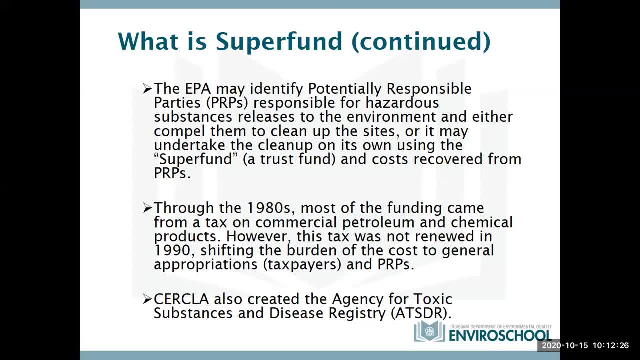 will So. and another little thing that CERCLA did- it was written into the CERCLA regulation- was to create the Agency for Toxic Substances and Disease Registry, or the ATSDR, who are also involved in environmental risk assessment And they're, you know that, probabilistic, you know. 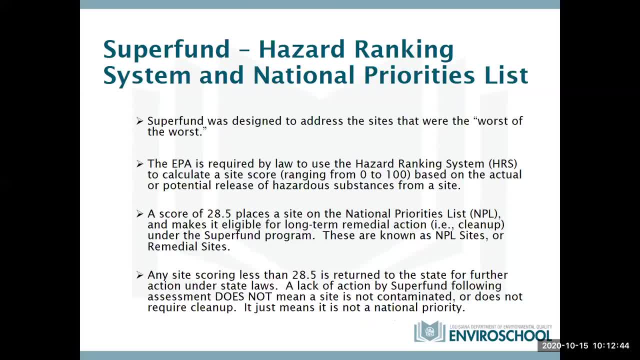 probabilistic risk assessment stuff we talked about. So that's important to our creation. All right, So the next thing we're talking about under Superfund is what sites qualify for Superfund. Does the gas station on the corner qualify? Well, no, because one, the gas station on 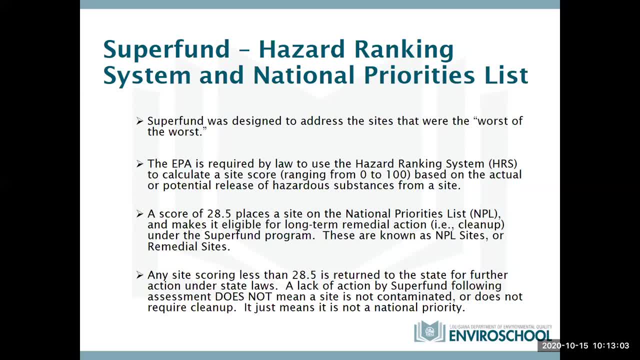 the corner would be exempt because of parole and exemption And secondly, it wouldn't score high enough. So what Superfund was designed to address was the sites that were not qualified for Superfund, The sites that were the worst of the worst. that's another term. you'll hear a lot. 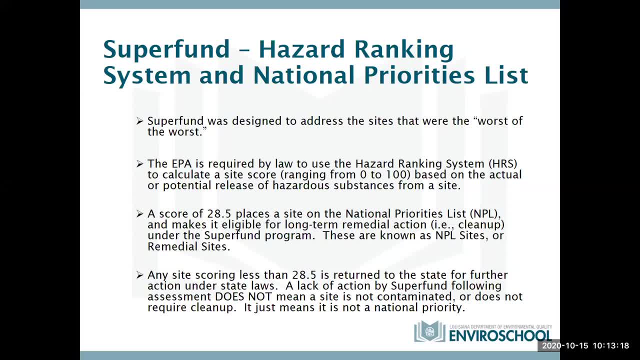 whenever you talk about Superfund. It was designed to handle the sites that are called a national priority And that's where we get the term NPL or national priorities list. So EPA is required by the law to use the hazard ranking system or HRS, which is to count. we have lots of acronyms in 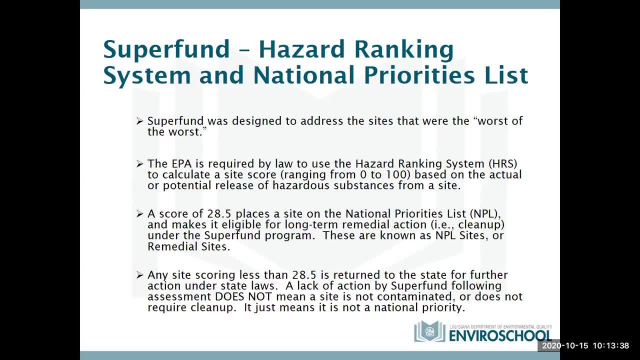 the environmental field, don't we? But anyway, the HRS is used to calculate a site score ranging from zero to 100, based on the actual or potential release of hazardous substances from a site. So they have various pathways. We just recently added a pathway, which is the vapor. 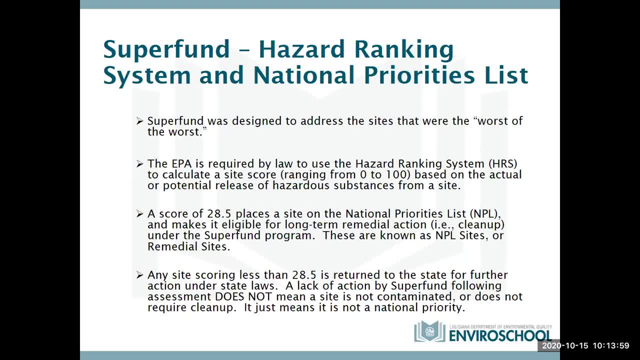 intrusion pathway, But you have groundwater pathway, you have surface water pathway, you have surface soil exposure pathway, the new subsurface of vapor intrusion pathway, And each pathway gets a score and then they're summed. they get a score Now to be on the national priorities list and be eligible for a Superfund. 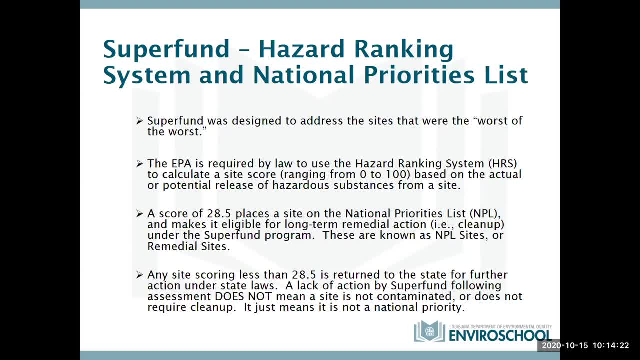 cleanup, the score has to be 28.5 or above. So, and where did that number come from? That's an interesting story. Well, EPA, in developing the HRS, had a list of sites that they felt like should be Superfund, that these sites, you know, should be Superfund. And so, when the HRS was, 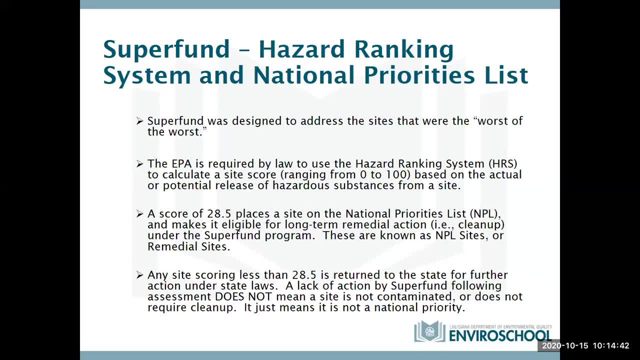 developed. they looked at this. they said, well, what number would cause these sites that we feel like should be Superfund to all be Superfund? And then that was 28.5.. So there we have it. That's what it was, So it's kind of arbitrary. 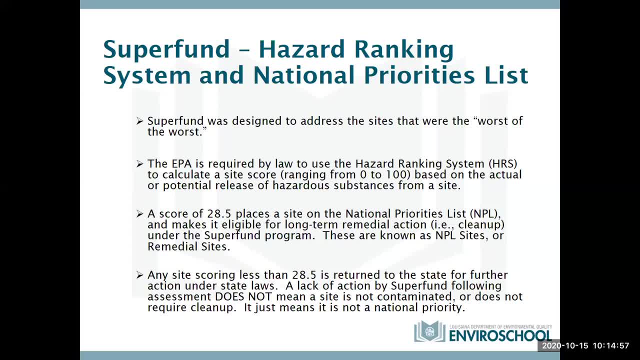 but it was based on the actual site inventory at the time HRS was developed. So once you score 28.5,, like my friend, Mark at EPA says hallelujah. we now have a Superfund site. Now we can clean it. 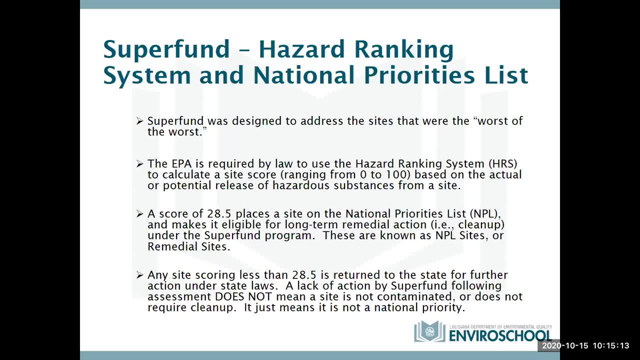 up. You know we have the money. The federal government has the ability to use the Superfund program to address the site on long-term remedial action. so cleanup. So those are the NPL sites, or we sometimes call them remedial sites, because they're eligible for long-term remedial action. Now let's talk about 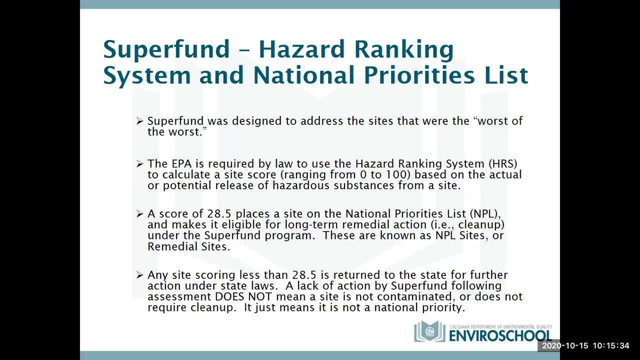 the other possibility though: a site that scores less than 28.5. So if it scores 28.0, that's not good enough. It does not go on the NPL site. It does not go on the NPL site. It does not go on the. 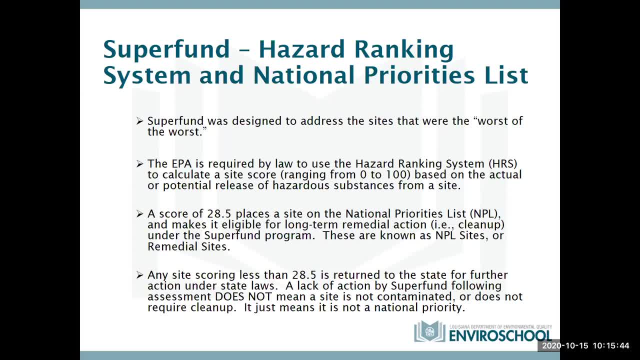 NPL. They cannot be proposed. It is returned to the state for further action under state laws. So a lack of action by the Superfund program following a site assessment does not mean that a site is not contaminated. It can be heavily contaminated. It does not mean that 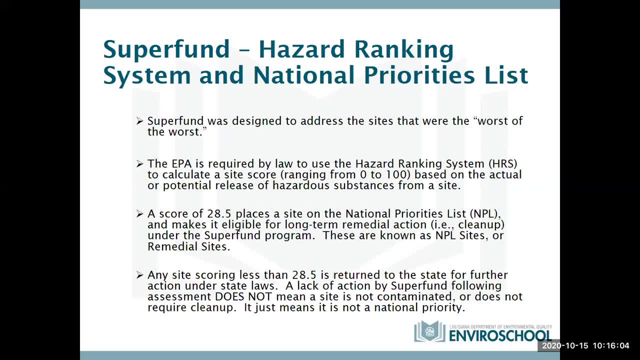 site does not require cleanup. It very well could. It just means that that site is not a national priority for cleanup, So it does not get that long-term cleanup. It is not one of the worst of the worst, as we said, So it's, you know, a lot of people. 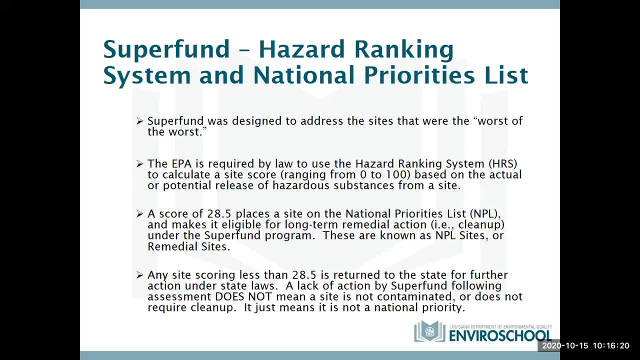 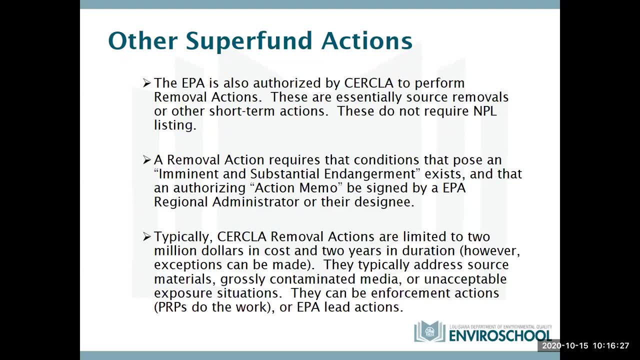 misunderstand that concept, because Superfund assesses a site and finds that it is not a national priority does not mean that there's not a problem there. Okay, All right. So let's talk about other actions under Superfund, though. We talked about the remedial program or the NPL. 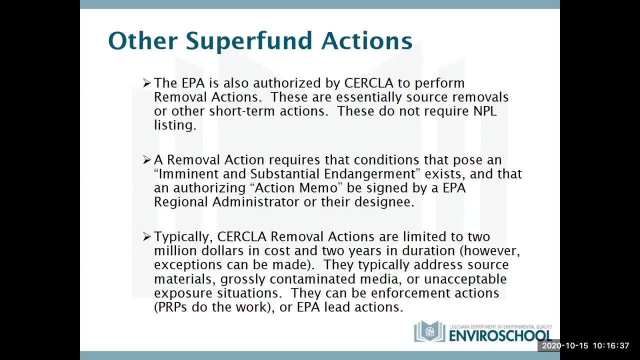 but there is another branch to the Superfund program that we need to address, and this is the removal actions, or the emergency response actions. EPA is authorized under the CERCLA program to perform these removal actions. What they essentially are- simplest thing. 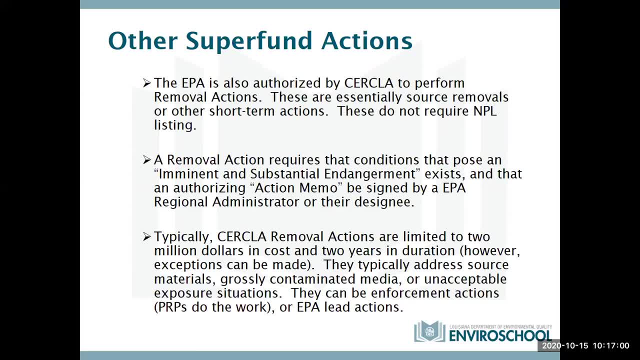 I can say is that they're a source removal or a short-term action. They do not require NPL listing, So sometimes these could occur before the Superfund assessment. It's better if it occurs during the Superfund assessment, because you can count them. 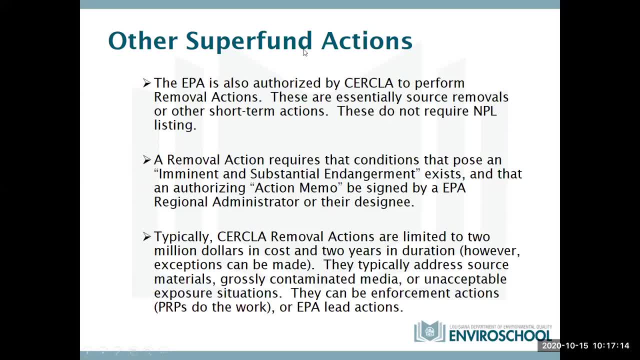 You can remove stuff toward the site score, but they you do not have to have a 28.5 score to do a removal action. Now, what does a removal action require? Well, now, this is a great term. It requires that the site 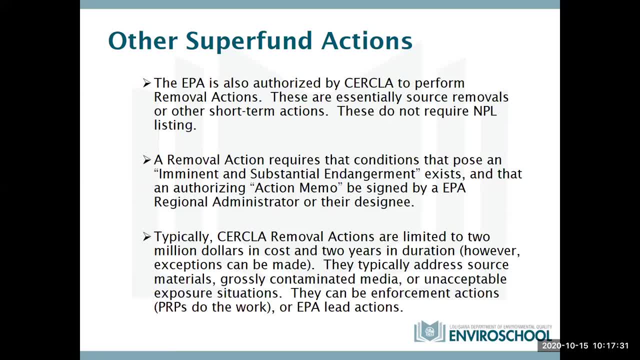 exhibit conditions that pose an imminent and substantial endangerment to human health and the environment. And then if you have an imminent and substantial endangerment condition, then an action memo has to be prepared and signed by EPA regional administrator or their designee, And then, once that occurs, you can move forward with a removal action. So this is a funny thing. 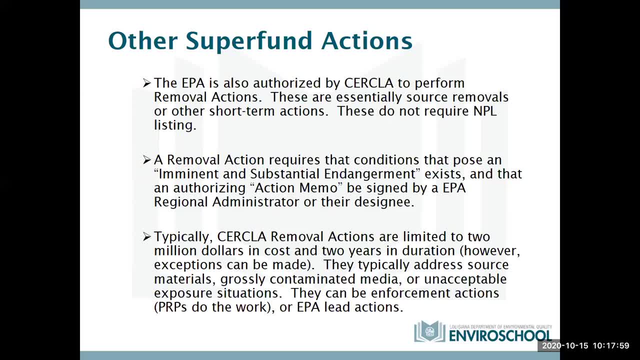 I remember, me and my boss, back in the 90s, we were talking to an EPA on-scene coordinator and we said: you know, can you tell us what this imminent and substantial endangerment means? Can you give us examples of conditions? And then we will, you know. 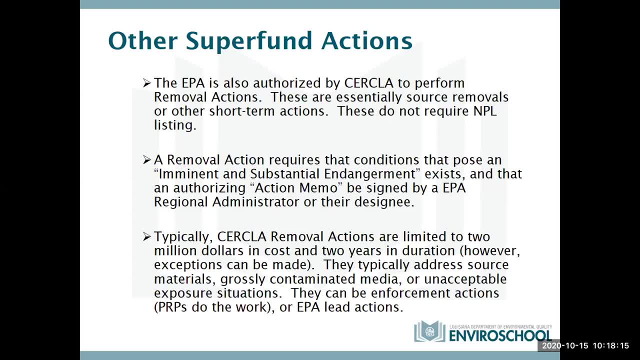 we will not try to refer to anything that you know wouldn't be appropriate. You know what is the definition of this? and he kind of laughed as you guys. Well, there is no definition, Isn't that an undefined regulatory term? 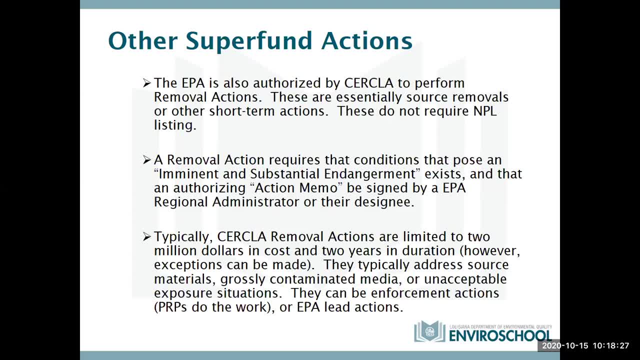 So it is, whatever a EPA regional administrator will sign off on in an action memo. So you know one person's imminent and substantial endangerment may not be to another, but it's you know. it's like that old saying, I know it while I see it. huh. So the EPA, when they freue you and they say you know that that's not an independent administration. 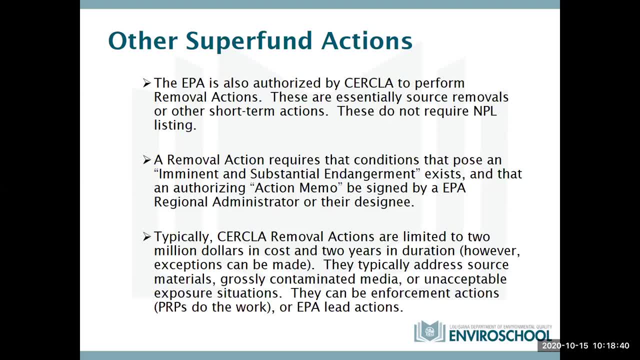 They're not able to say the different things that you want them to say in that particular application. So the EPA, when they see an imminent substantial endangerment and they convince the regional administrator that one exists, then you can do a removal action. 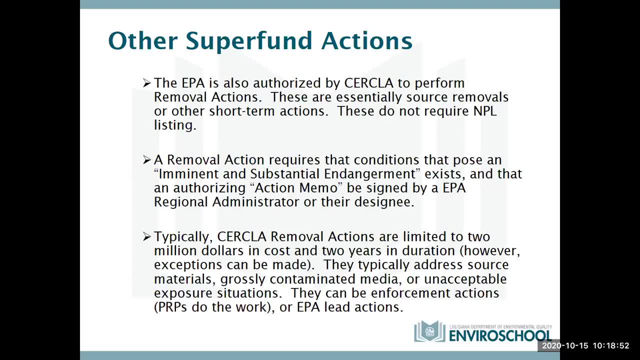 So now, what are these removal actions like? Well, they're limited typically to $2 million in cost and two years in duration. You know, it's not a long-term cleanup, It's a source removal action. So that's the usual rule of thumb: $2 million and two years in duration. 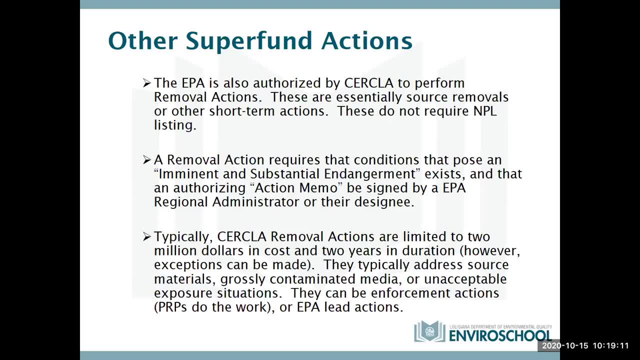 Now, exceptions to this can be made. You can have larger costs and you can have longer duration, given exception in these cases. So some of the examples of ones that we've had in Louisiana. we've had removal actions like West Bank asbestos, where the asbestos came in Cherokee and Johns Manville scattered all over West Bank. 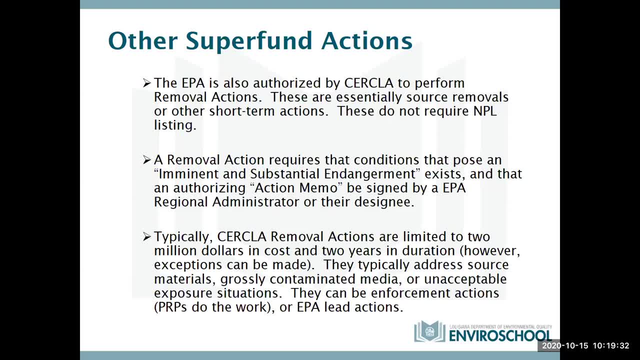 That was an exceptional one- It went over two years and $2 million- And another one was New Orleans methylparathion, which was where parathion- That methylparathion- was illegally distributed in New Orleans area and used by people as roach spray, and EPA had to do a lot of removal actions because that stuff is not, you know, of course, appropriate for use in that manner. 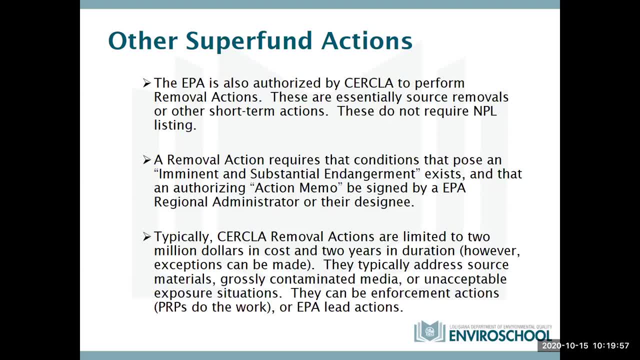 So there was a black market in it, as it turns out Now. so what are removal actions typically supposed to do? They're address the source materials. So we've got some waste in tanks. They're deteriorating. We've got some waste in tanks. 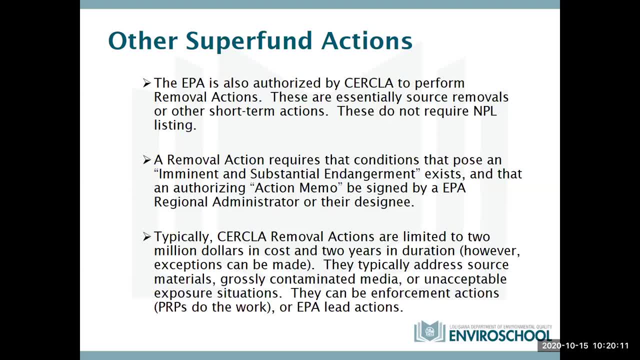 We've got some waste in tanks. They take away the tanks and the waste Grossly contaminated media, So you've got, you know, soil that's saturated with this contaminants. You remove the contaminated soil And or unacceptable exposure situations. 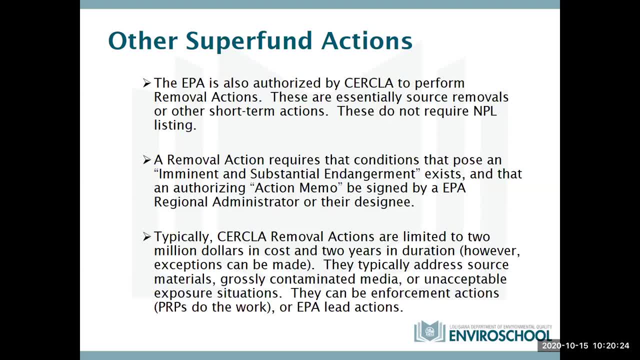 Now, in this case, here's one example of an unacceptable exposure situation. You have some people drinking from a well that has hazardous substances in the groundwater, So that is unacceptable. So what they do is they connect them to the rural water district. 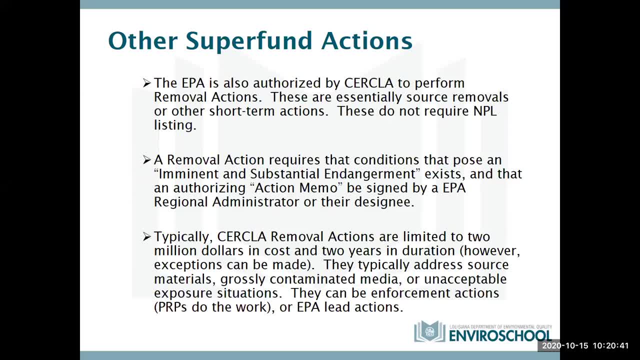 You know. so that takes away the exposure situation. It doesn't clean up the groundwater but solves the exposure. So now another thing about removal actions is they can be enforcement actions. If there are PRPs identified, EPA can order them to do the removal action to address the 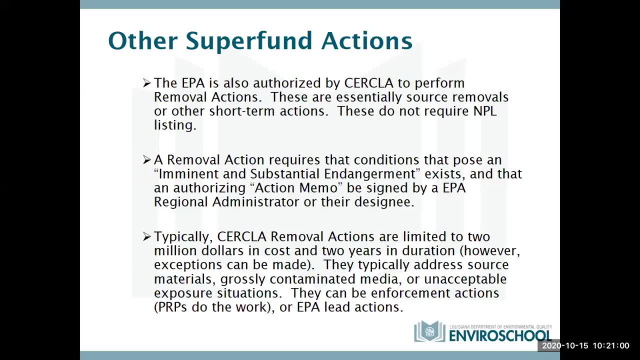 intimate substantial endangerment. Now, in other cases, where either PRPs are unable or unwilling to do the action, then EPA can lead on these actions. So, Tamika, Yeah, All right. So let's talk about a recent removal action here in Louisiana. 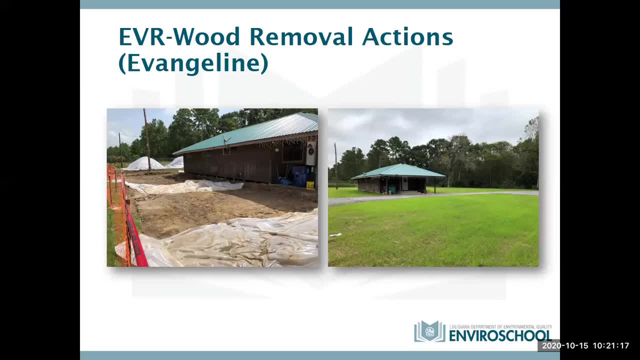 This one's over in the community of Evangeline, which is near Jennings, And this is at the Everwood Wood Treatment Superfund site. This building you see on your screen was the plant office for the Everwood Treating Company, And later it was converted by the Land. 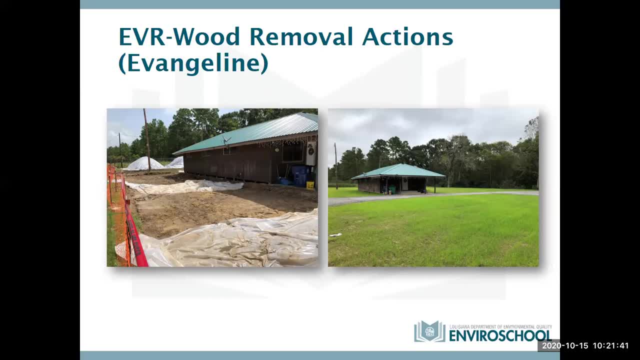 owner into. as far as I know, it's always been a house since Everwood closed, but people began living in this former office building, you know, before I got involved in the site, and that was in the 90s. So I don't know why, but this seems to be a strange thing in Louisiana. 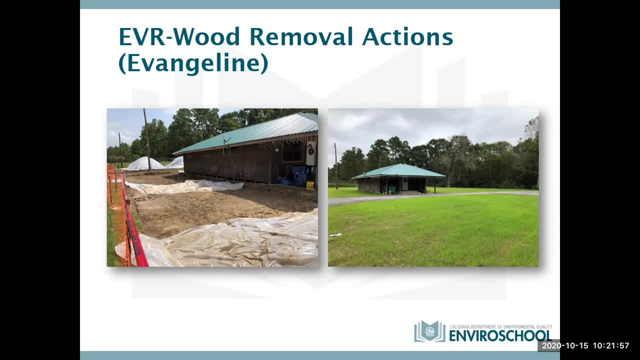 At wood preserving sites, which are generally- almost always- heavily contaminated, people always want to live in the office building that the wood treating site had. This is the case for this one Also, Union Creosote, which is small. The Creosote are up in Union Parish. 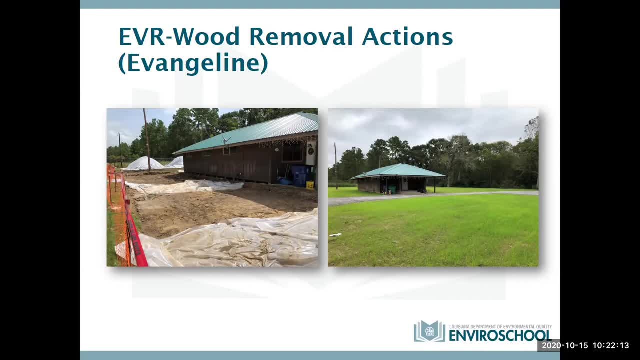 The other unfortunate thing. it seems that there often is either children or pregnant women living in these structures when we come across it, So that was the case here. There were two young children and a lady that lived here with the son of the landowner. 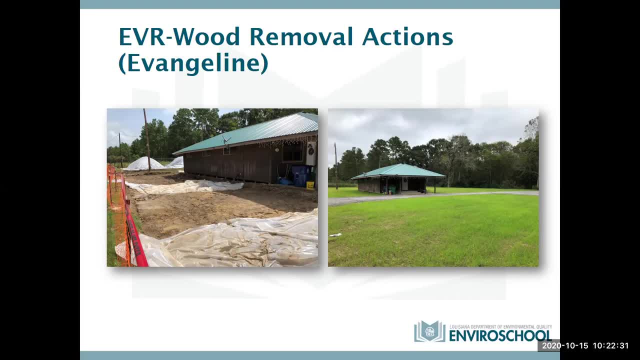 And so you know, when EPA began to do the assessment of the Everwood Treating Company site, they took some samples in the yard of this house to see if there was a potential exposure for the these on-site residents, And indeed there was. 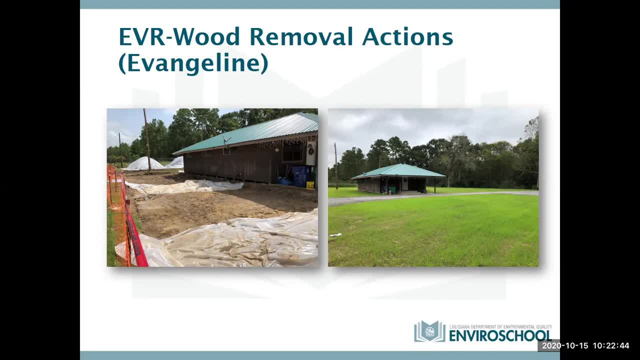 There was arsenic and dioxin from the treating compounds that were used at Everwood. Everwood used- we call it the triple threat. They used both Creosote pentachlorophenol, which breaks down into dioxin, and copper chromium arsenate. 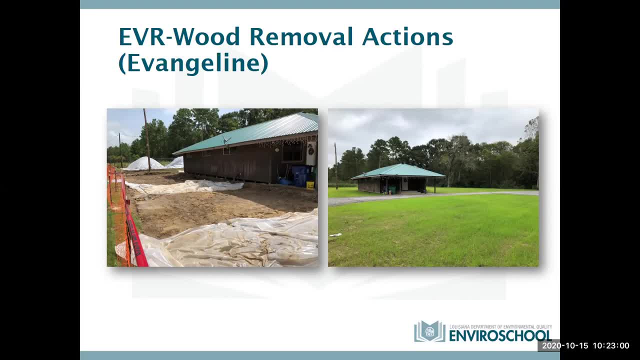 or womanized, which is called CCA, And so they have all kinds of exposure issues. So what was done as a removal action to Address this exposure scenario was to remove one to two foot, depending on the depth of contamination, from the yard of this former office. 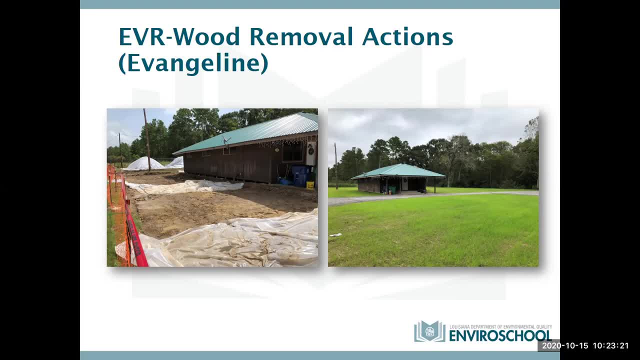 which is, as you see in this picture, now a home, So on the left side you see it. during the removal action, This is on the left side of the house. They only had to remove one foot on the other side. 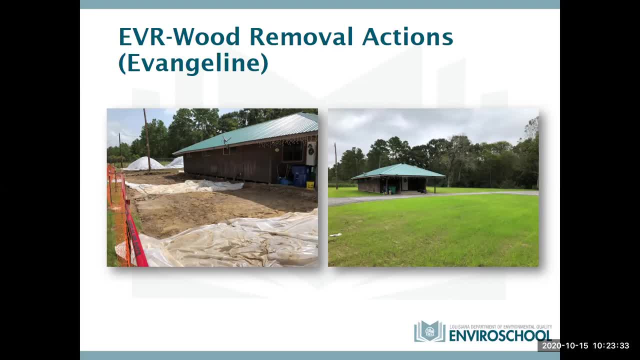 It got deeper into two foot. It was based on, you know, sample results. And then the soil in the back is staged under those tarps And then the right is. after the removal action, they removed one to two foot of soil. they backfilled it with. 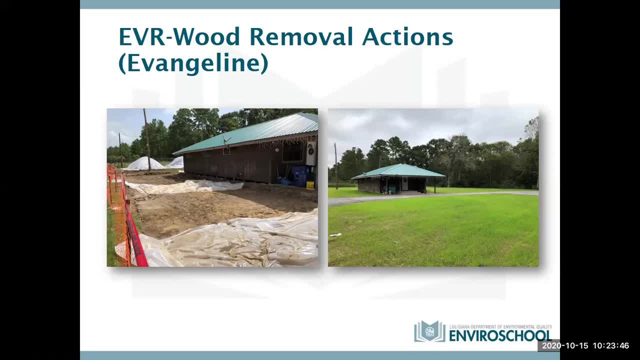 clean soil and they planted nice grass. it's really a nice yard now, but anyway, after that, the lady that lived there convinced her husband, the son of the landowner, that you know, it might not be best if we have our kids living on a Superfund site. and so you know, hey, I applaud that decision and 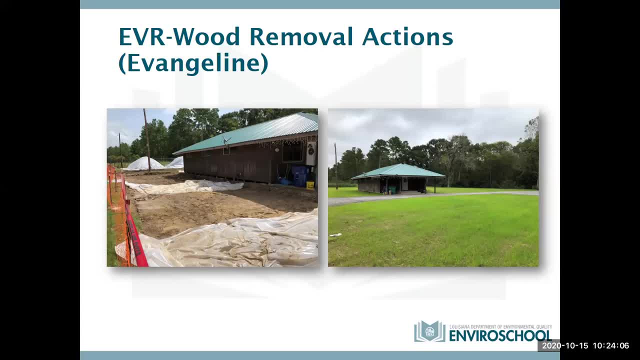 so after they moved out to the removal, they never moved back in. however, the landowner's other son, I understand, lives there now, but at least he doesn't have wife and children there. so you know a little bit, a little bit less exposure, I guess. all right, Tamika, all right now, also at Everwood, now that 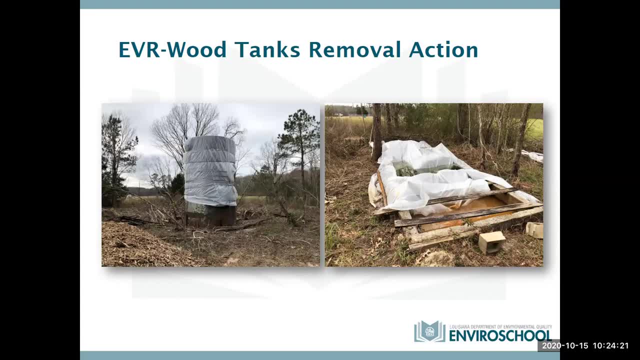 first removal. I told you about the house. that was one removal action. it was limited: two years and two million dollars. now another removal action was performed at Everwood. this was called the Everwood tanks removal action. this was to address- and this is more a- this is a classic removal action. uh, you know that yard removal action. we talked about that. 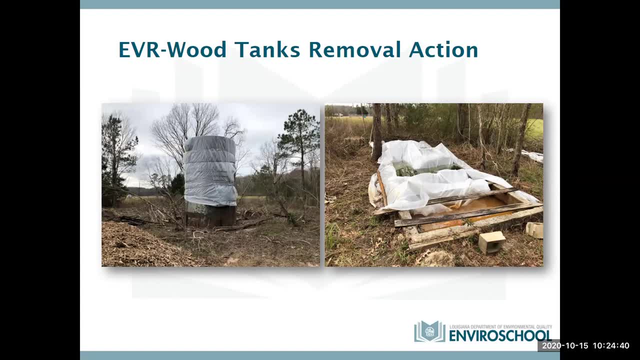 addressed an unacceptable exposure situation. right now, the Everwood tanks is more of a classic removal action. it was intended to deal with the last remaining waste on the facility, the source material. so on the left you see the penta chlorophenol tank that was uh left at the facility. 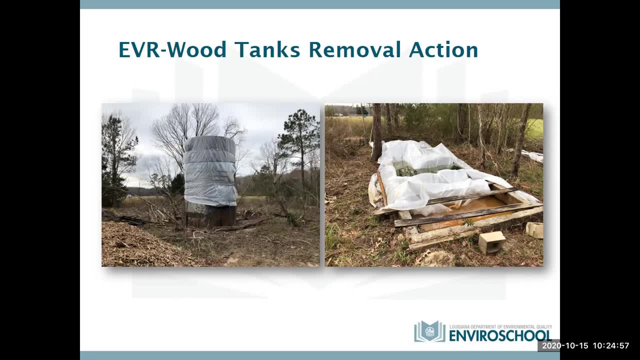 and it's covered in some, um, you know, sheeting and and some uh tape, because they've removed all the trees from around it and they've removed all the trees from around it and they've removed all the it that had grown up around it, and you see that those trees are now mulched on. 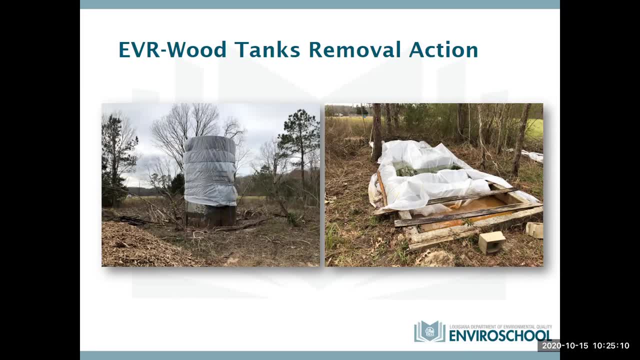 the left there and they're preparing to actually remove the tank and its content. So this was when it was being, you know, addressed. Now, on the right hand side of the phase, we have a in-ground. they call it a separator. it's a concrete structure. 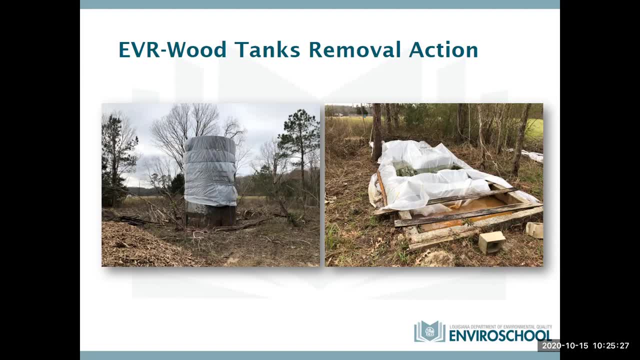 that would catch the penta chlorophenol solution. that would come out the treatment cylinders when they were opened and then the penta chlorophenol would be recovered and any water would be treated. I'm doing air quotes, you can't see that, but anyway would be treated and then discharged under 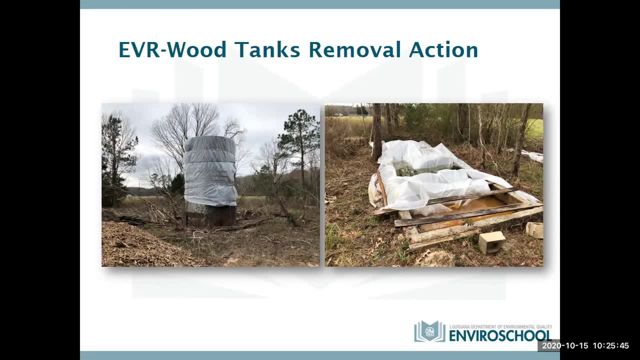 whatever rules existed back in the 70s and 80s. So that is actually that brown stuff in. there is a penta chlorophenol water mixture that's very high in contamination levels, So that was removed and there was also an underground. 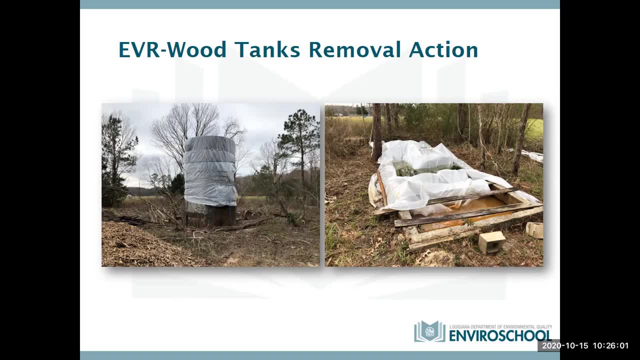 storage tank that contained penta chlorophenol from the water separator and that was removed. So this was more of a classic source removal action. Again, this is a separate action. you got a separate budget of two million dollars and two years duration. 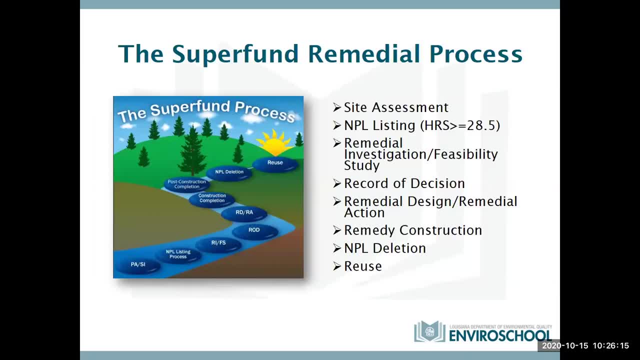 So sometimes you got to know how to play the game. So that's the removal program. We do short-term actions to remove source material and grossly contaminate media and to address unacceptable exposures. But let's look at the Superfund remedial. 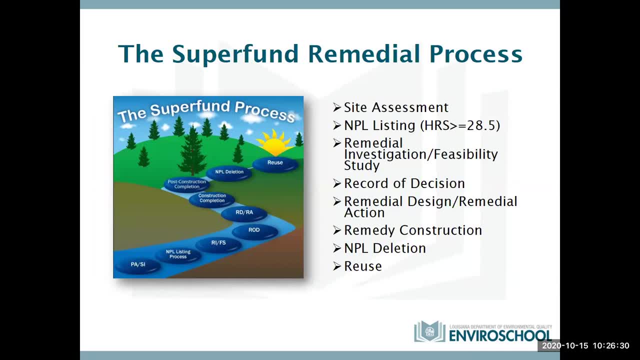 process, the NPL. NPL listing the long-term remediation process. Now this: I want to apologize for this diagram. this is EPA's diagram, not mine, but you know, hey, it's what is. But if we look at it on the left, we see a little diagram and it starts out with: 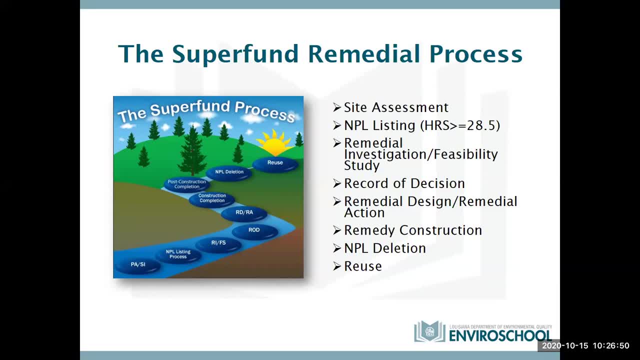 what it says, PASI. and you see, everything's brown and scary. and then we follow the pathway of blue dots all the way up till everything's green and happy and we finish and we're done. So that's the NPL. So that's the NPL. 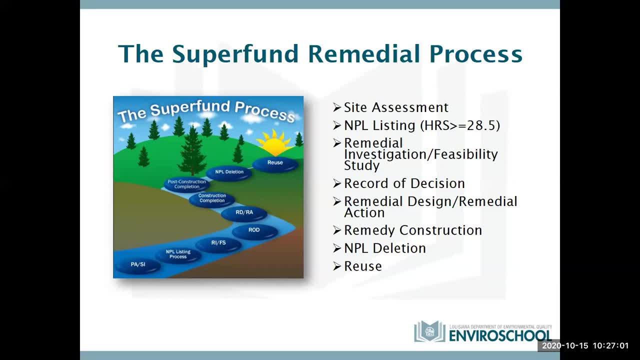 Then we reuse the site. So hey, it's okay, I guess. But we start the Superfund remedial process at the site assessment phase. You know, either the state or EPA identifies a site that might have NPL potential, and so a site discovery is. 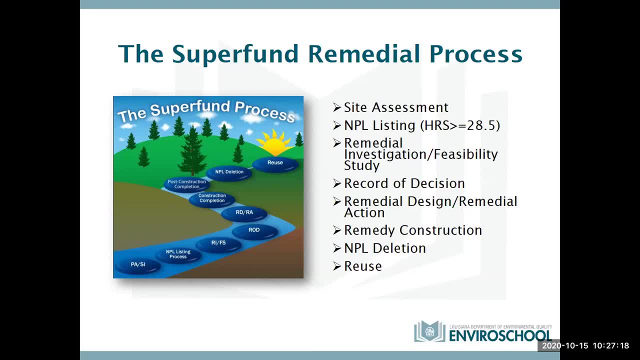 done and then to determine if it's going to score 28.5, we have to do a site assessment. The site assessment done by EPA under the Superfund program is a two-step process. The first is called the PA, our preliminary assessment, And that is 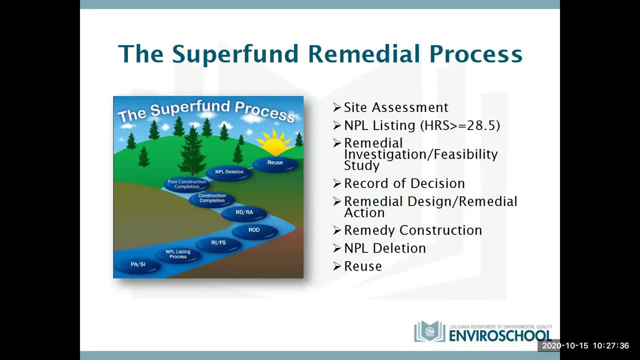 generally a study of the site that does not involve sampling. You look at the history of the site, the records, you look at potentials, pathways and so forth, And if all that indicates that, yes, it could be a NPL candidate, then you go on. 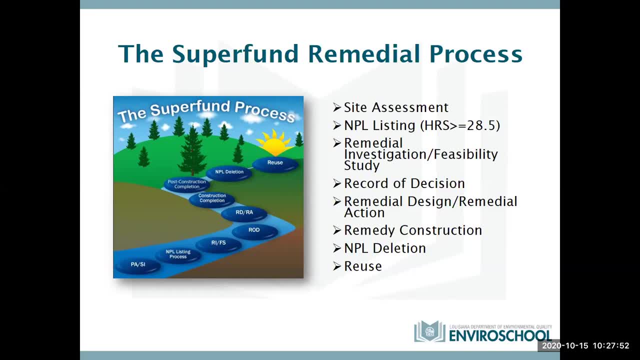 to the SI, which is the site inspections phase, and that's where EPA or their contractors, or sometimes the states, take samples, samples to determine if those NPL pathways are contaminated, to determine if the targets are affected. And what you're looking for under the site assessment is what we call an observed release. 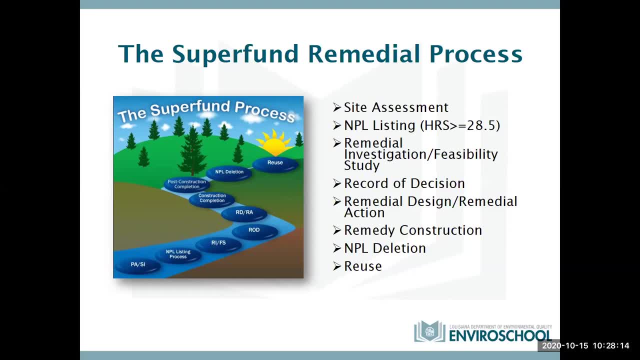 That is, to determine if hazardous substances have been released to the environment And an observed release is different than a cleanup level. An observed release is either three times background or three times the sample quantitation limit if there is no background. So if you have a release, 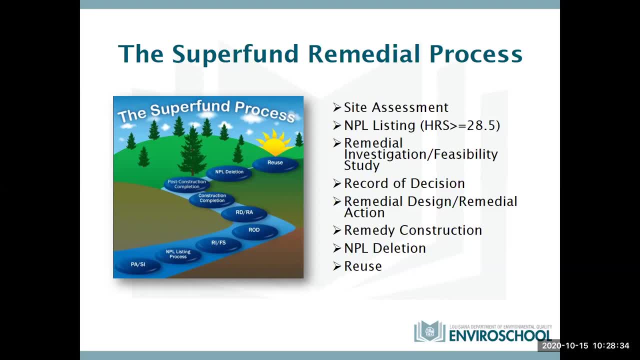 in the site. it could be a release that doesn't require cleanup, but it does show that the site is, you know, releasing contaminants to the environment. So we do the PA and we do the SI, And if you know the pathways, give us a score that could be over 28.5, then EPA goes into the. 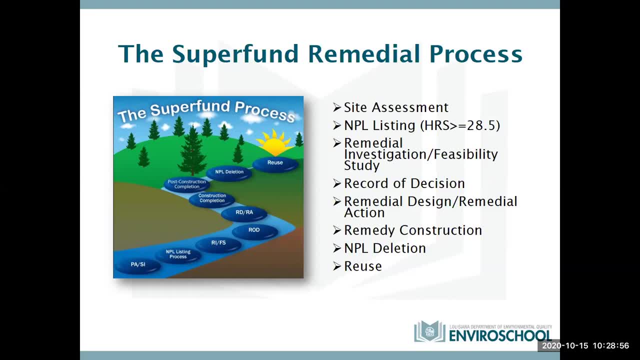 NPL And they do that through an NPL listing process And they have to publish it in the federal register as a proposed site And then if there's, you know, opportunity to comment in other stuff, and if that goes forward, then we have it in the federal register again as a final listing And it's on the 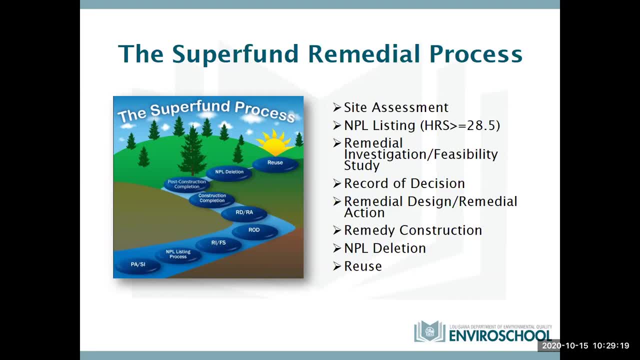 national priority list. Hallelujah, as Bart says, we have- now it can clean it up. So the next phase. you say: wait, we already did an assessment. Why do we have to do a remedial investigation? Well, 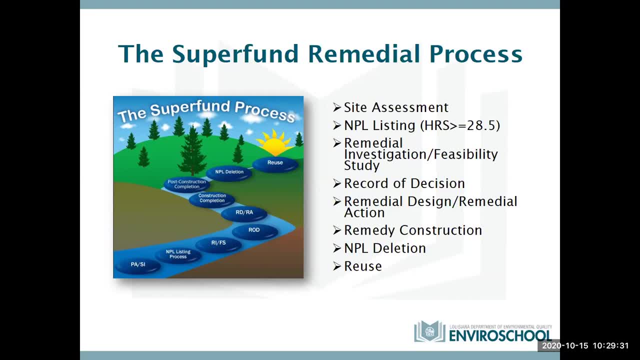 it serves a different purpose. The remedial investigation is designed to determine the extent of contamination. We're going to look at the horizontal and the vertical extent. We're going to look at those pathways in more detail. We're going to try to determine exactly. 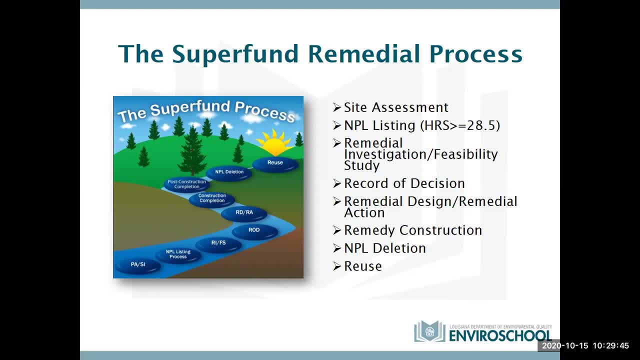 how much cleanup we have to do. And then that's the remedial investigation. The feasibility study portion of this RIFS is to determine what are our options for cleaning up. What potential options could we utilize? Could we dig it all up? Could we bio-remediate it? Could we? 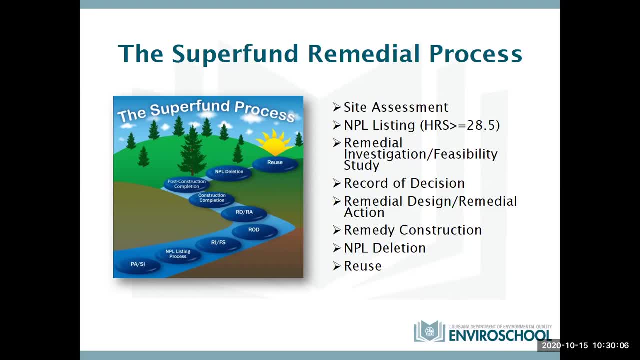 use capping and fencing? Could we do a combination of these things? So these are all looked at and the various feasibilities of these options are investigated and, in conversation with the RIFS, Cost estimates are developed so we can see what the various different options would cost. 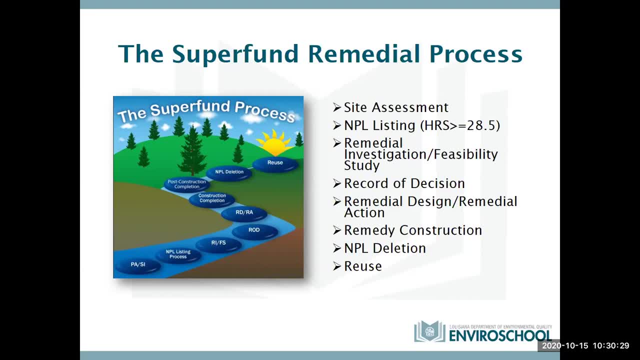 After the feasibility study has been completed, the EPA and the DQ and other partners, like the Department of Health and EPA's ATSDR partners, look at the results and a proposed plan is developed. And the proposed plan is then taken before the public. 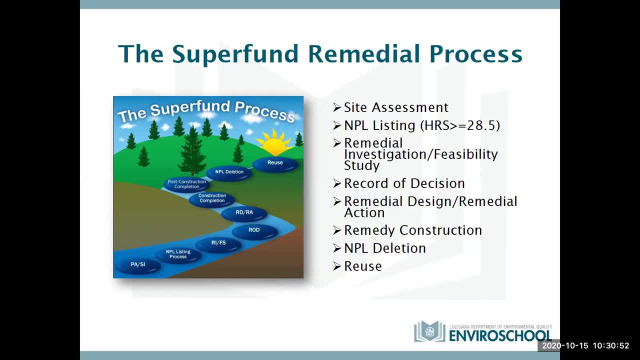 We can say we have this site area, we have public outreach and involvement. We say we think the best way to address the site is option three, whatever that is, And if the public agrees, then we go into what's called the record of decision. And again, that's a very formal step. It has to be signed off on by 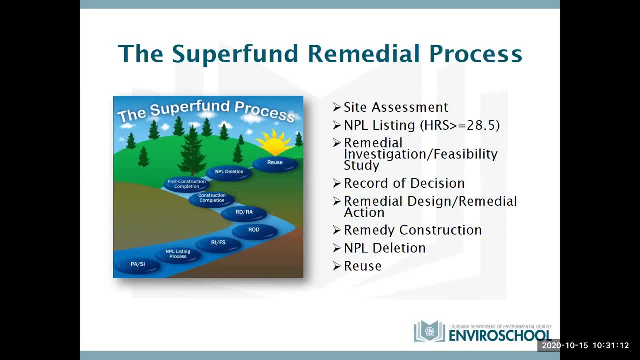 the EPA regional administrator, And this is what we looked at, why we made the decision. We did the and this is what we're going to do. These are the cleanup levels we're going to achieve, and then this is the operation maintenance we're going to do after the. 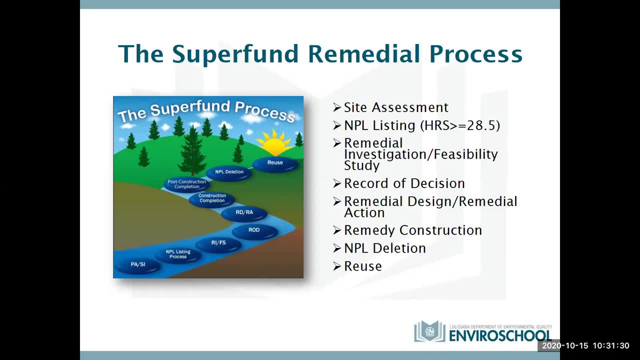 cleanup. So this is really a very formal and important step in the site process: the rod, if we will. Now, after that, we do remedial design. That's how we try to design the cleanup, We do the engineering of it, We figure out how we can dispose. 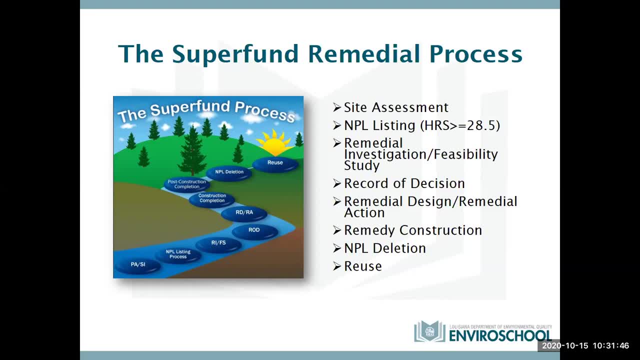 of the stuff we're going to dig up. We do our waste profiles, etc. You get all the ducts in a row so that the actual work can occur. Contracts are written and let, and then we do the remedial action. That is, we do whatever the rod says. we're. 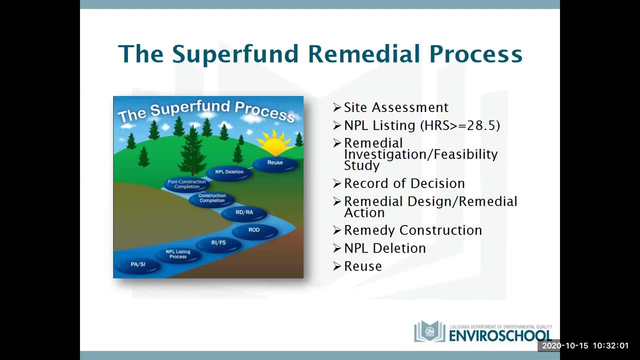 going to do, And so we implement that Now. the remedy: construction. sometimes this involves constructing a cap of fence. It could involve constructing a groundwork treatment system and operating it for a number of years to make sure it works properly, and so forth. So it just 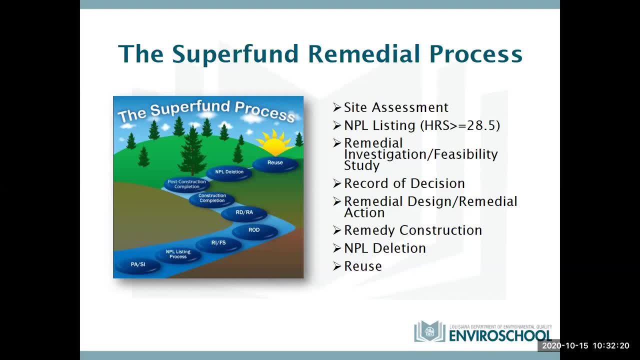 depends on the project, What the particular remedy is. Historic remedies involve constructing on-site incinerators and burning waste until you know reach through meal goals and land filling ash. So really depends on what the site is and what the remedy is. as to what that entails Now, after the remedy, construction, you have the construction. 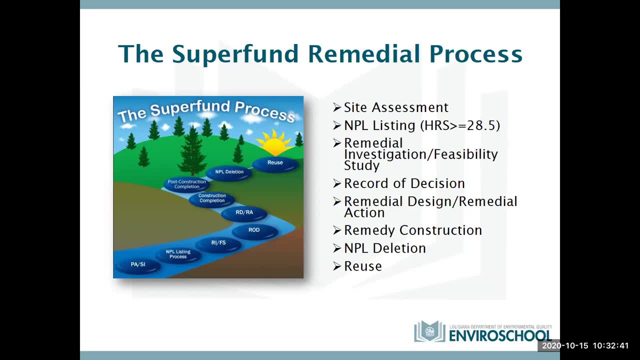 completion and post construction. Please see our little steps on left. We're up to the green area. now We have pine trees in our biographie, in our little diagram. So at that point, once the remedy has been implemented and you know everything has worked out, then we can consider. 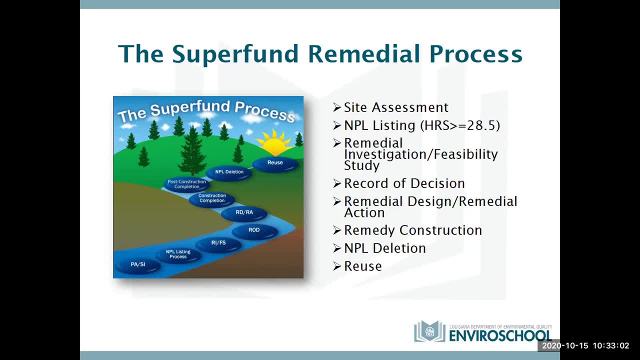 deleting the site from the NPL, The cleanup is complete. then we go into operation and maintenance phase, if that's warranted, depending on site conditions. So and then, lastly, after we've cleaned up the site, we can reuse the site. Now my friend over at EPA who does the ENF cleaning and 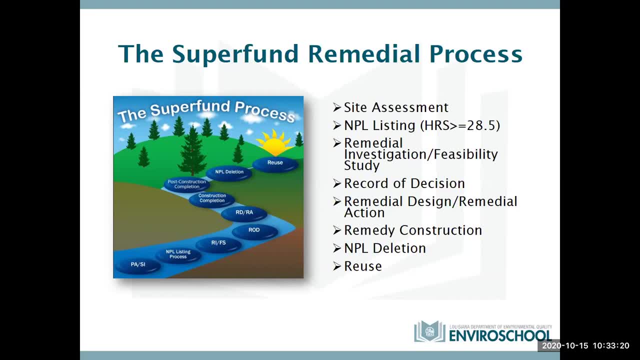 site reuse could point out. some portions of site might be able to be deleted and reused before this end of the process. but this is a simplified diagram, So we always want to bring things back into commerce if we can. So if portions of the site are found not to be contaminated, we might cut them. 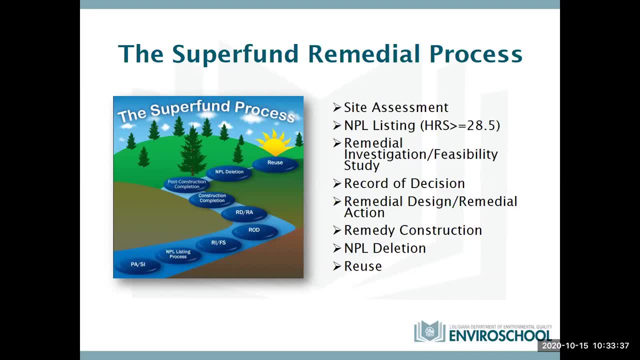 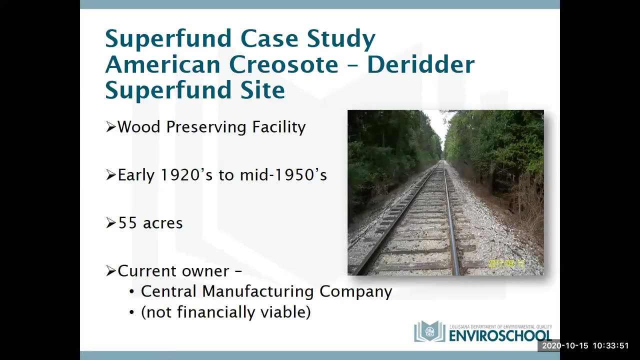 out of the site and delete them earlier. So it just depends. All right, Tamika. Okay, that was it. I can hear you Next slide, please. Okay, great, That was tough. Okay, well, you know, technology is wonderful. 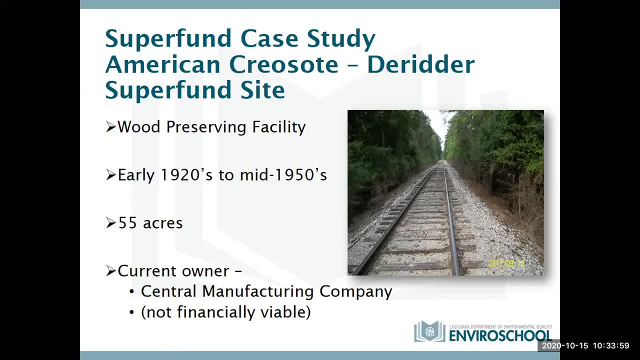 All right. so we talked about the process in general and I thought what we should do in order to really kind of hone down on how this works is: look at our newest Superfund site. let's looks at our newest Superfund site. let's do a case study. 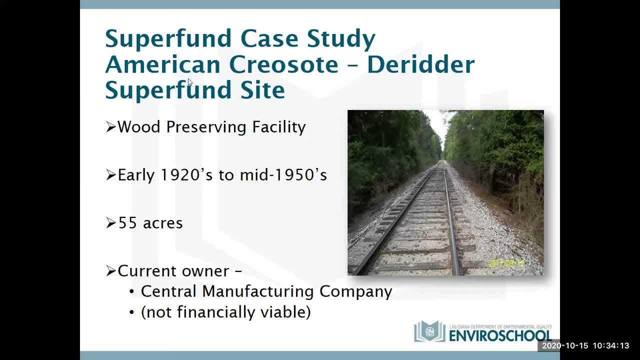 let's look at our newest Superfund database, and if people want to access a Superfund site in Louisiana, This is the American Creosote and DeRitter Superfund site, And so we'll go through an actual example. We're not done with. 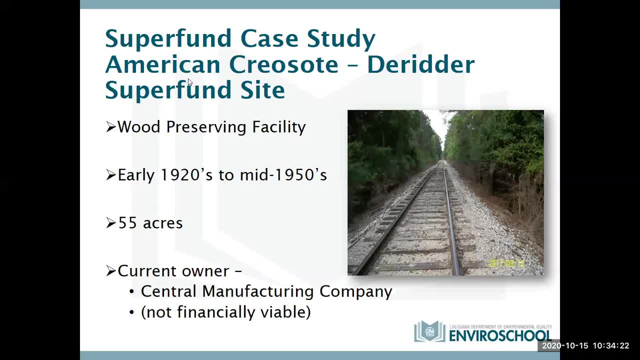 this one, but we're in it, Of course, as the name, American Creosote, might suggest, it is a wood preserving facility and it is in DeRitter, So it operated using Creosote as wood preserving, you know, compound from the 1920s to the mid 1950s. 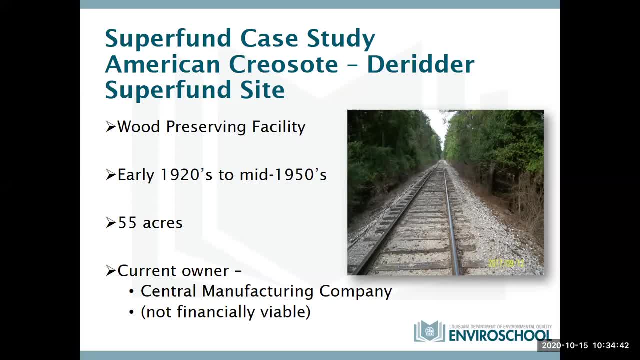 when it went out of business, And the picture on the right shows the way we used to access the site. The best way again was the railroad track that ran through the thick woods that had grown up on the site since it went out of business in the 50s. It was nothing but a big patch of thick. 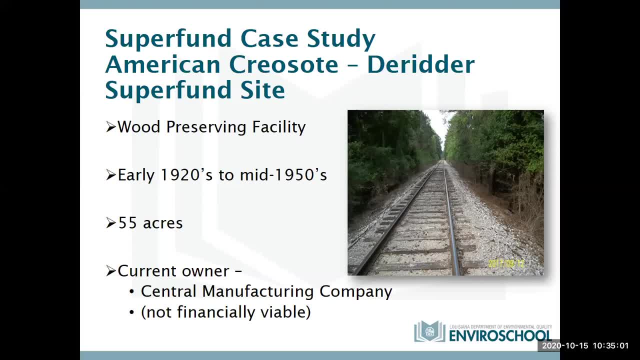 pine and yaupon and other things. I'm a biologist so you know trees get to me All right. so the site itself was 55 acres in size and it was owned by a company called the Central Manufacturing Company that had bought it with the idea that they could possibly redevelop it, but they quickly. 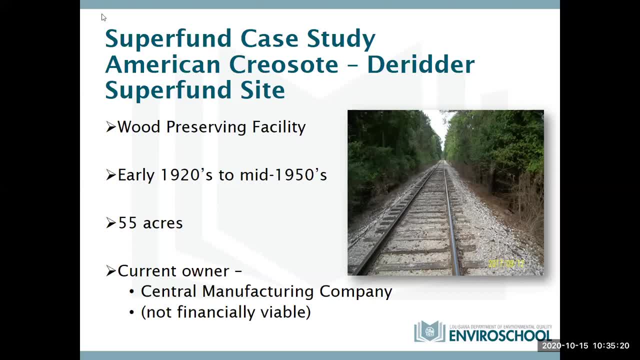 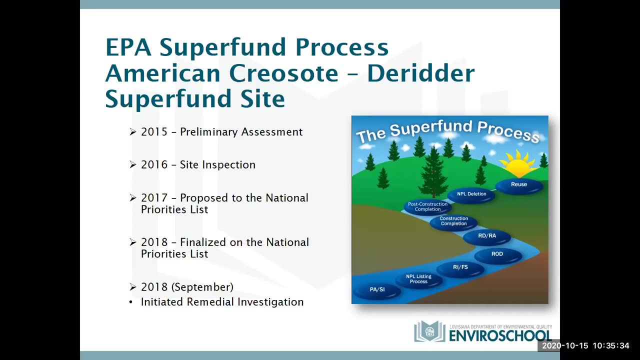 learned that the financial cost of doing that exceeded their ability. They were not financially able to take on the cleanup of the site of this magnitude. So let's apply our little diagram to the American Cruise Set site. So we began to do the preliminary assessment of the site in. 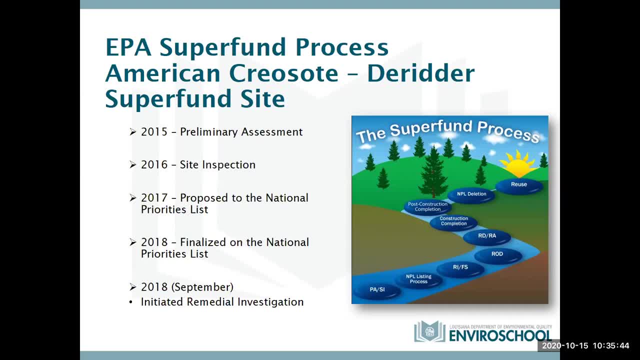 2015.. EPA and their contractors and DEQ all went out there and began to look at the pathways and the targets and so forth and did our paperwork and it looked like, hey, this is a potentially good candidate. 2016 was the site inspection. EPA got access agreements and began to take samples to 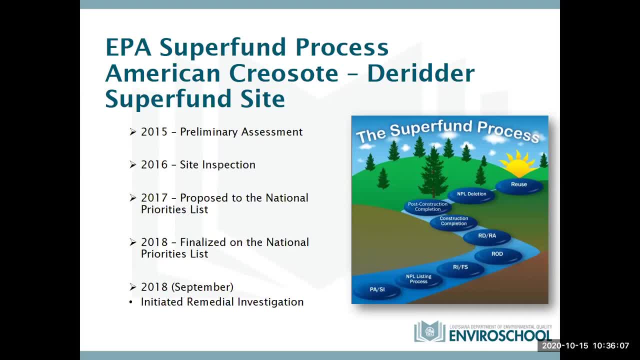 determine the Background extent of the contamination in regard to the pathways. did it have npl potential? well, sure enough it did. it was uh proposed to the national priorities list in 2017 and in 2018 it was finalized. so you know, that's that two-step. you have to publish it in the federal register. 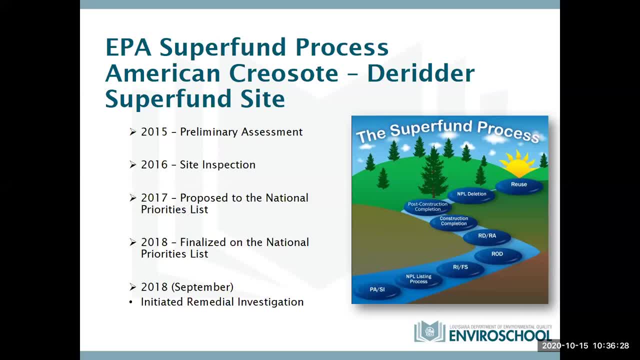 and you know, have a period when there could be comments etc. and then we have to go back to the federal register to finalize it. so it was finalized, uh, and in 2018- in fact september 2018- we initiated the remedial investigation and we are uh still there. um, we're still working on that. 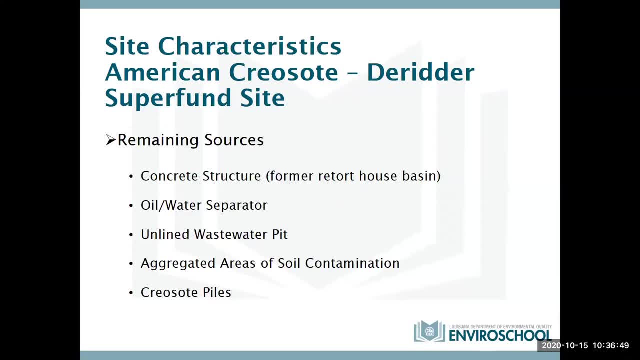 remedial investigation. so to make up all right. so the uh site characterization, uh, excuse me, characteristics of the american criticism deriver superfund site. the remaining sources are a concrete structure which was the former pressure-resistant site, and the remaining sources are a concrete structure which was the 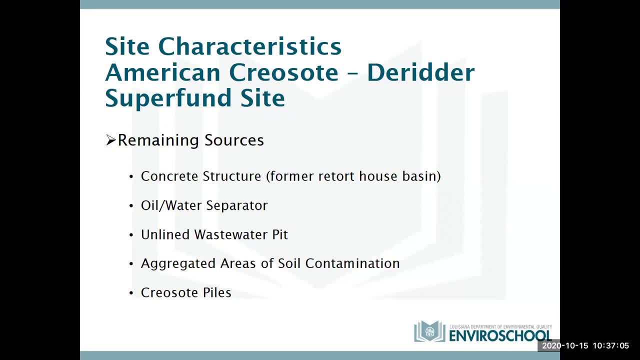 former pressure cylinder or retort. that's a word you don't see too much anymore, but those pressure cylinders that they use to pressure treat wood are called retorts and that was the retort house basin. there was an old water separator that had creosote waste. there was an unlined wastewater pit that. 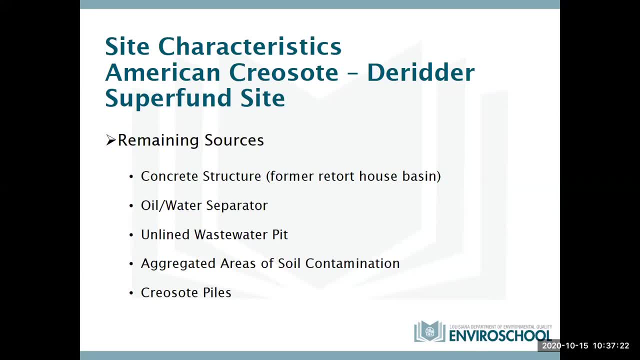 was heavily contaminated with creosote and waste. there are various areas of soil contamination and there were piles of creosote waste in the woods that apparently had been disposed of there. when, when the plant was dismantled and salvaged- I guess they salvaged what they- 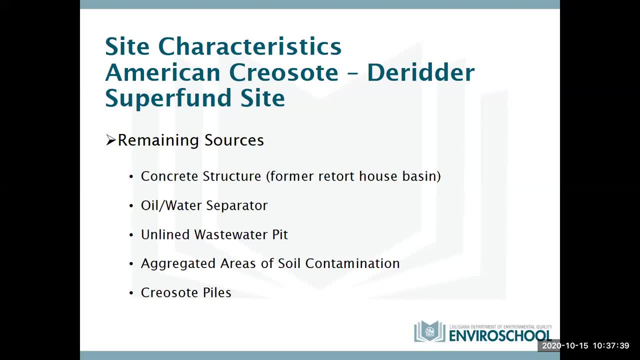 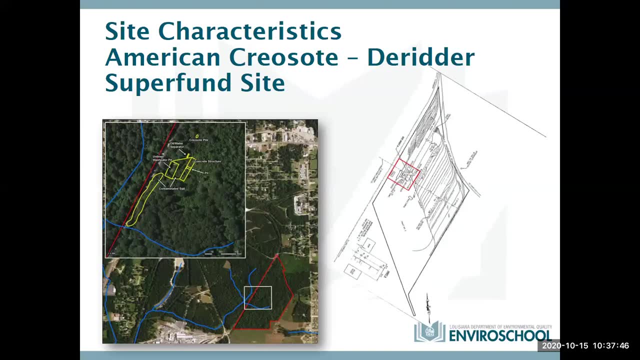 could, and the waste was all left on site. So next slide, please. Okay, this kind of is a multi-step overview here. If we look on the left, we see a big map that has a little white square in it. The red outline shows the 55 acre property and 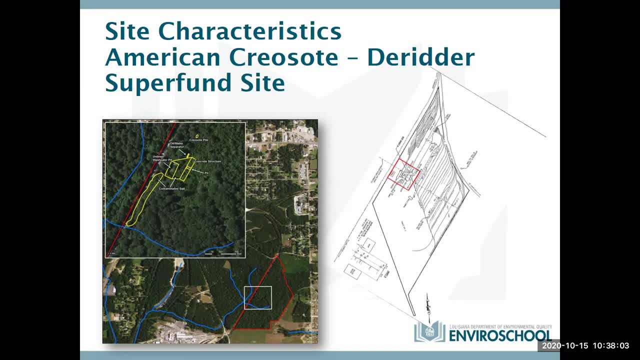 then the blue lines show the surface water drainage pathways from that property. And then when we look at that little white square that gets expanded to be up on the upper left, That shows a zoomed in version with the process area and its contaminants: The concrete structure, the contaminated soil areas. 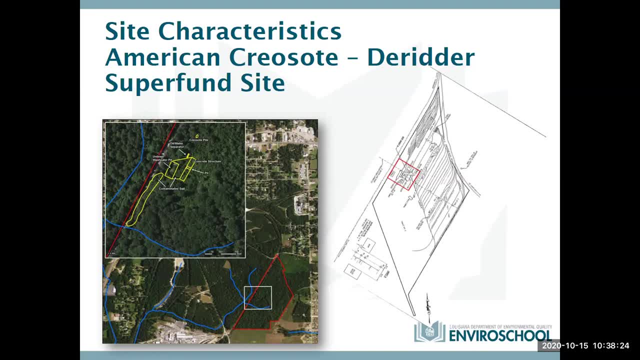 the wastewater pit, the drainage path that had creosote, all the way down creosote pile, etc. So if we look on the right, what we're gonna see there is a historic map of the facility that shows what used to be. There used to have a number of various little railroad tracks. 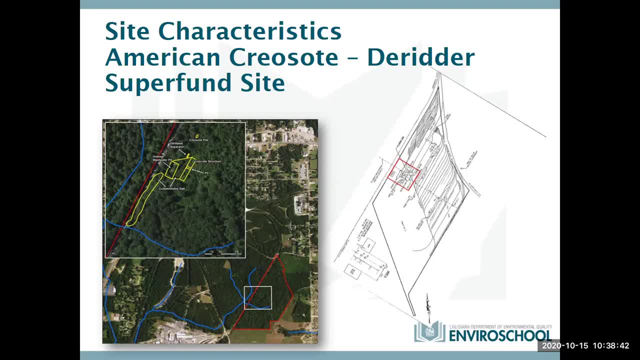 that were used- Narrow-gauge railroad to move logs around so that they could be treated, and wooden structures like ties. creosote was used in railroad ties for a long time. That was a very big use of the creosote material- still is. And then that little red square there shows the area that's. 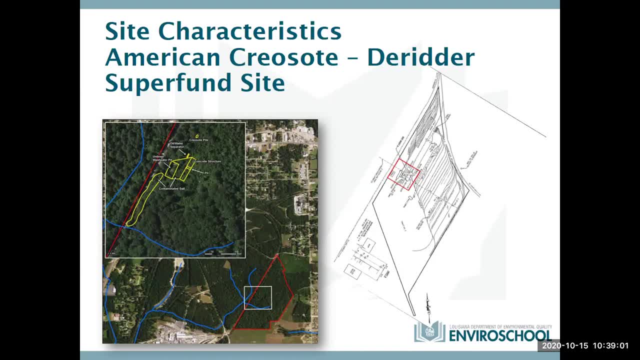 in the white square on the left. So that shows the land that has the, the process area, if you will. So of course you're concerned about the process area because that's where the creosote was at. You're also concerned about some of those outer areas because they could be what we call drip. 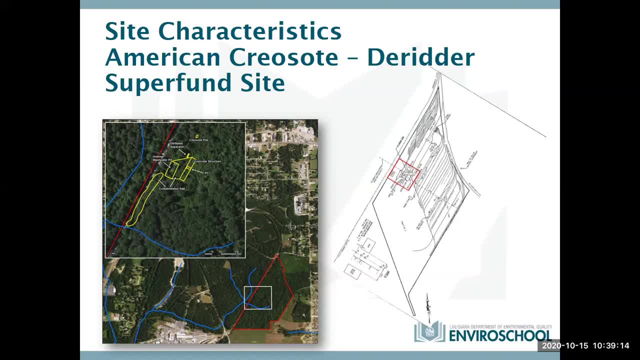 areas when creosote was pressure treated into that wood and then it was pulled out of that retort or pressure vessel. A lot of times they'd roll it out somewhere so all the excess creosote could drip off and then that would result in soil. 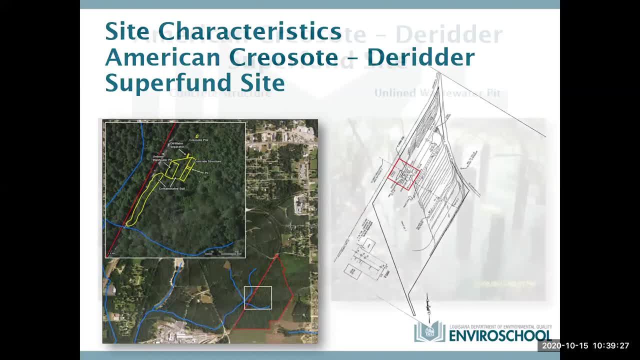 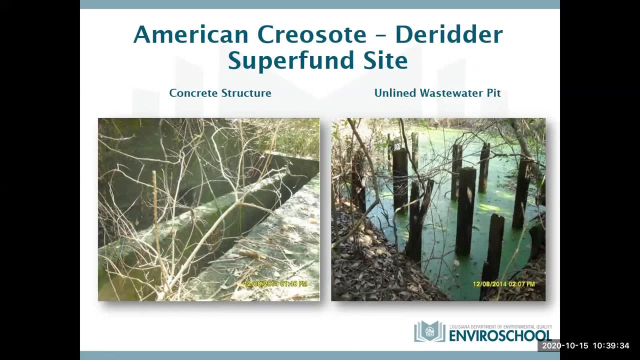 contamination. Here's just a couple of pictures of the conditions we found at the site, and this shows 2014.. So this was during the pre-PA phase and site discovery phase, I guess. But at the left we see one of those concrete structures that could be an oil water separator. I think that was. 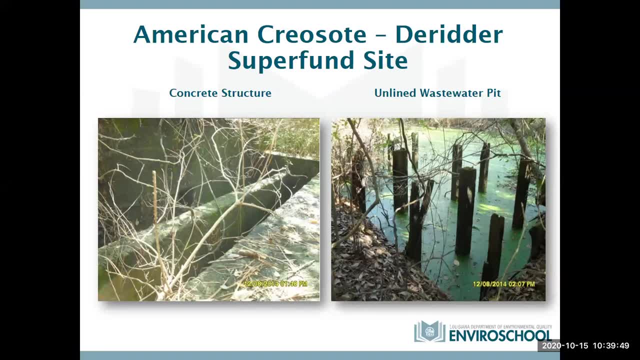 assumed and you see the black stuff and that's creosote. Creosote is listed hazardous waste. by the way, It's an FO hazardous waste. Now on the right we see that open surface water body. that was sort of we. 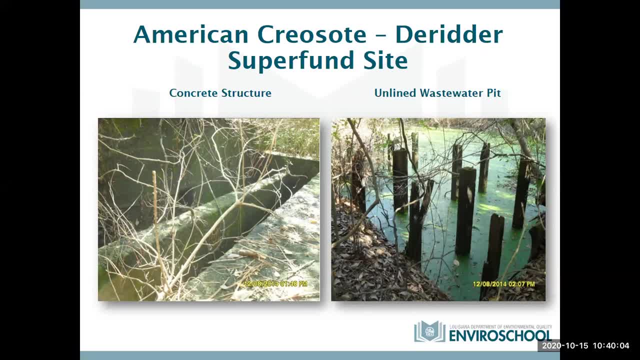 thought a water treatment pond or something like that and that has some duckweed growing on it, but it's heavily contaminated with creosote all across its bottom And of course, creosote, in addition to having hydrocarbons and nastiness, is loaded with polyaromatic hydrocarbons, or PAHs, which are 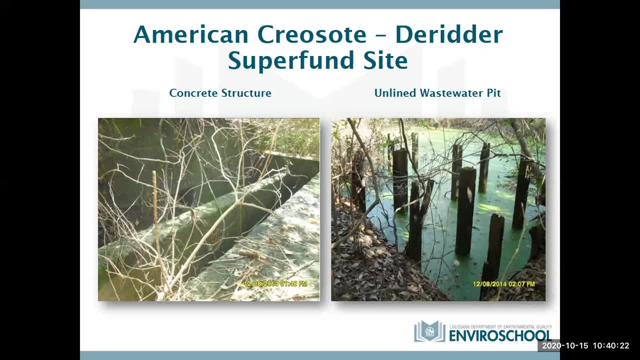 powerful carcinogens. So that's one of the primary concerns. So you notice that these pictures were taken in December. they're 12-8, 2014.. That's because this thing was so grown up with woods and you know vegetation. 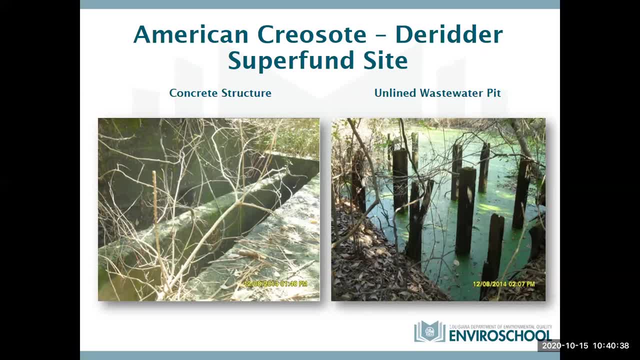 from the 50s that you know that was the best time to really get in there. that you know. still, you had to chop away through the brush. When we were doing the PA and SI, they actually rented a bulldozer so we could bulldoze a path to. 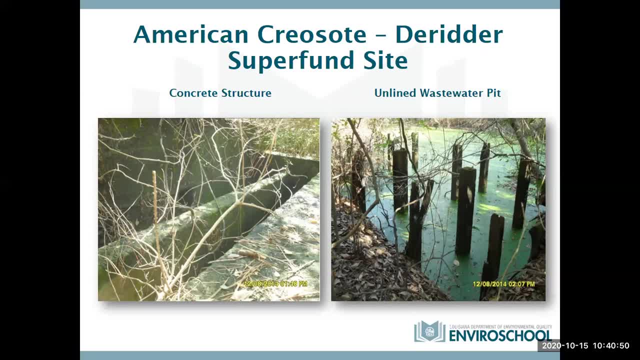 the areas where we had to take samples and, you know, do some drilling work. So yeah it was, it was a lot of work. So yeah it was, it was a lot of work. So yeah it was, it was a lot of work. 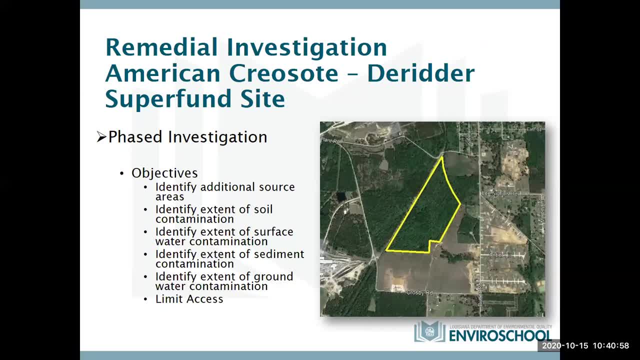 Okay, All right. So, having done the PA SI again on the MPL, then we had the remedial investigation. We were looking at a phased investigation because EPA's budget, you know, isn't what it used to be. You know we don't have 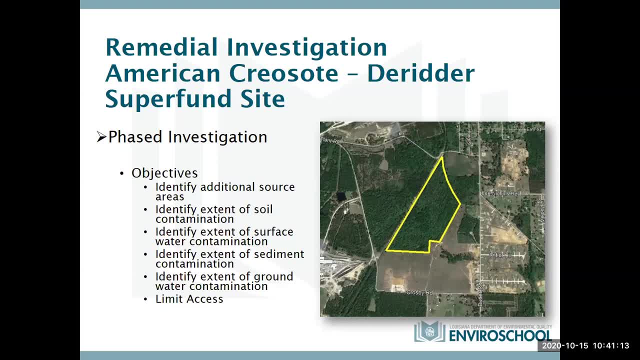 that Superfund tax anymore. So they're on budget and you know the federal budget. you know there's all these sequester cuts and everything else from time to time And you know so EPA has been doing our eyes as a phased investigation. So you do a portion of it, then you do. 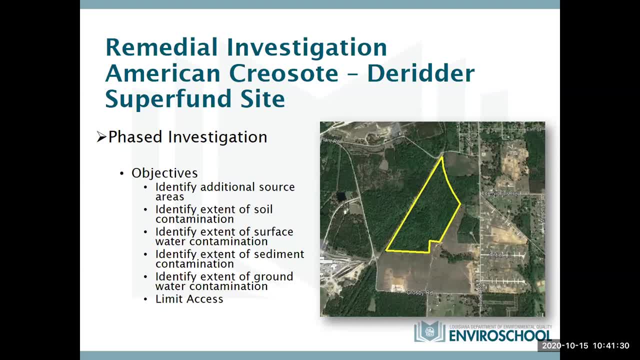 some more when you have some more money and more time- And this isn't necessarily a terrible thing. I mean, instead of going out all in one year and spending, you know, millions of dollars to do all the sampling- sometimes you do some sampling. you look at those results and you say 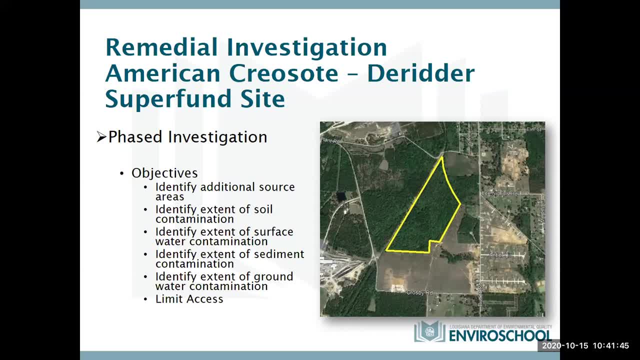 hey, based on that, I think I need to answer some more questions. So you go and do your next phase of sampling. So, although it takes longer, sometimes it gives you better results. But it's really a practical reason. It's, you know, it's what it is. So in the objectives of a remedial 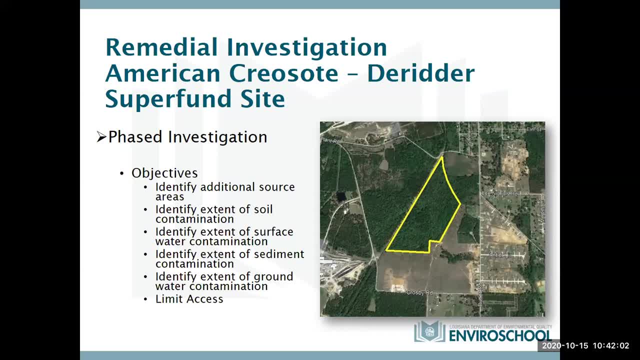 investigation are to identify any additional source areas that we did not find during the PA and SI, you know, during our initial thing, because, gosh, you know, this thing was just grown up so thick We have no idea what might be out there really at the beginning. 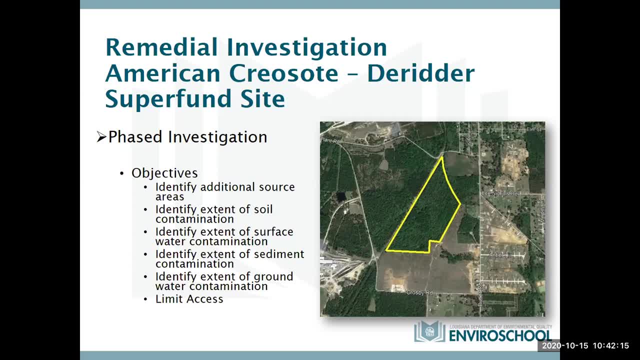 We just went to the areas that we knew were likely. We went to identify the extent of soil contamination. you know where were those drip areas at, where you know might there be other areas that would have to address? We wanted to identify extent of surface water contamination. 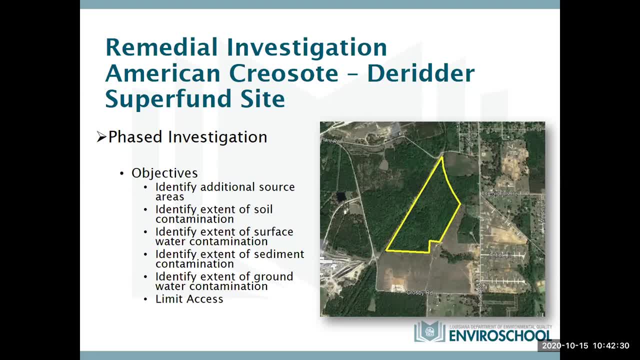 There's really two drainage paths in the site. We find out during the RI. there's one to the southeast and one to the southwest. So we, during the PA and the SI, we only knew about the one to the west, You know. 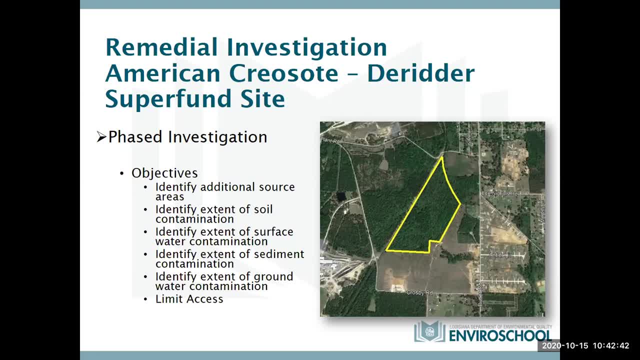 during the RI we were able to determine: yeah, there's another drainage path and, yeah, it's contaminated. So that was important. Identify the extent of sediment contamination in those drainage paths. How far does it go? Where might we have to address it? 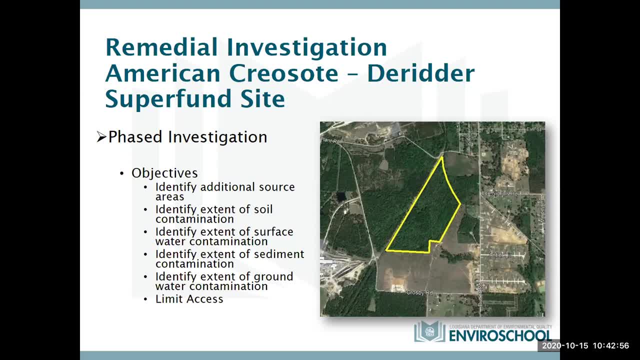 And the ground level. you know the ground level. you know where is the extent of that groundwater contamination. We knew that there were some in the process area but we don't know how far it extends And does it affect anybody's wells around there? Because all those people around 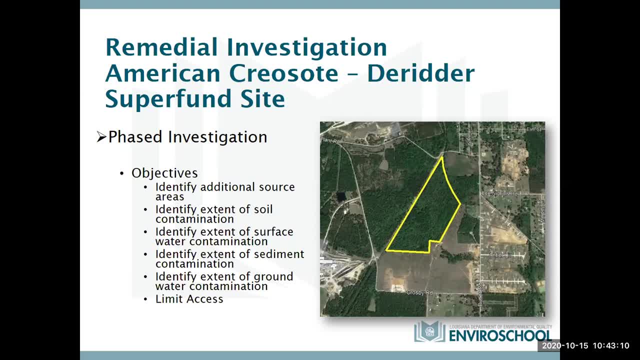 there drink water from wells, And another thing we wanted to do is limit access because you know we have, you know, creosote on the surface of the ground. It could be, you know, hunters or trespassers, or you know. 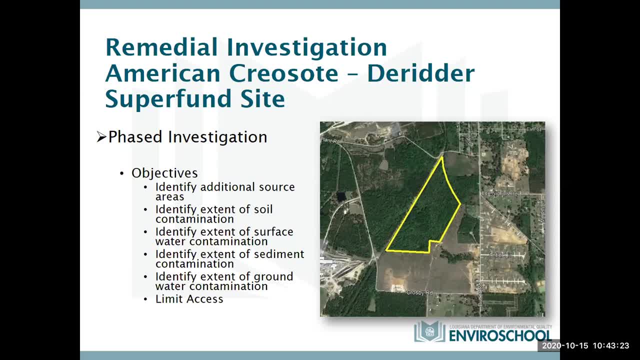 kids playing in the woods could come in contact with it, So we didn't want that to happen. The only limit to access prior to the RI was the very thick vegetation I was telling you about. it's just difficult to get in there. Well, during the RI, we had to open up pathways. 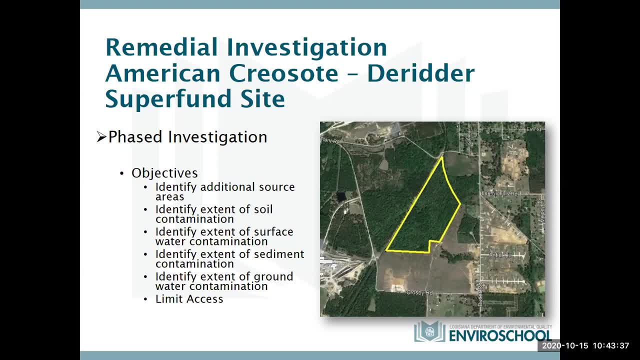 We bulldozed and made roads on the site to access these areas so we could do the sampling, But that also opens it up so kids or hunters or other people could get into it. So one of the goals that we did was fence the site. It cost a lot of money but it was necessary to prevent, you know. access And unfortunately we got a lot of trees damaged our fence in the recent hurricane, so we've got some fence repair upcoming. It's a shame, because it was all so pretty and shiny and new and now it's pine trees damage it, fall all over it. 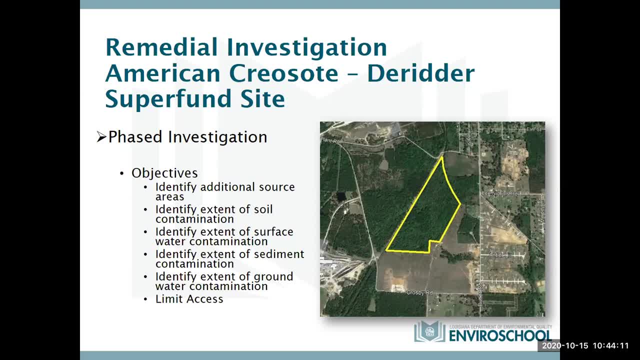 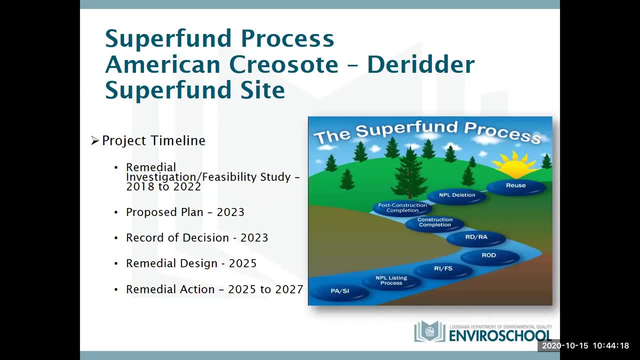 But part of the thing will get fixed. All right, Tamika. Okay, so back to the Superfund process timeline, The remedial investigation and feasibility study. we're planning that to run from 2018 to 2022.. Now, I told you, it takes a while. 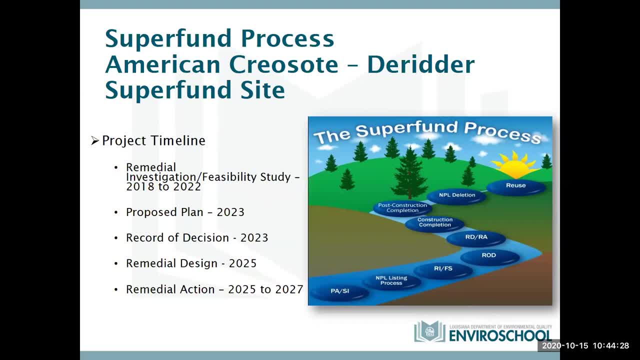 It's in phases. We are currently in the investigation phase and then we're going to finish that up and go into a feasibility study phase. So we're right on schedule. We're in 2020.. You know we were able to continue. EPA contractors were. 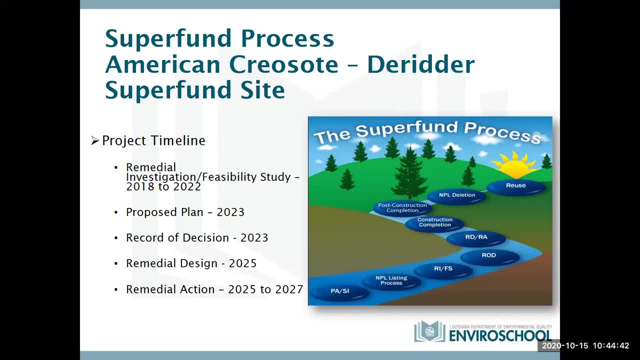 able to continue working through. you know the global pandemic, which is good because they were able to work in that remote area. you know practicing social distancing and and using safety. You know they said that they felt safer they would in you. 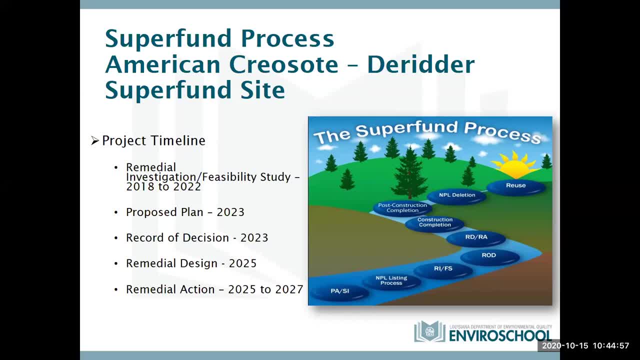 know some of the big cities that they normally work in. so, hey, The proposed plan. we expect to have that ready for you know, consumption by the public and comment in 2023.. We hope to get to a record of decision at that year too. and 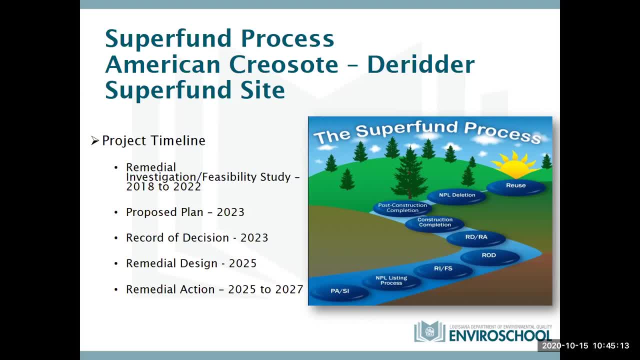 then we can begin the remedial design and the remedial action. This may move a little bit faster, because one thing that happened on this particular site is there was a safety couple up near a high-dose lawn and what we found there was it was a. 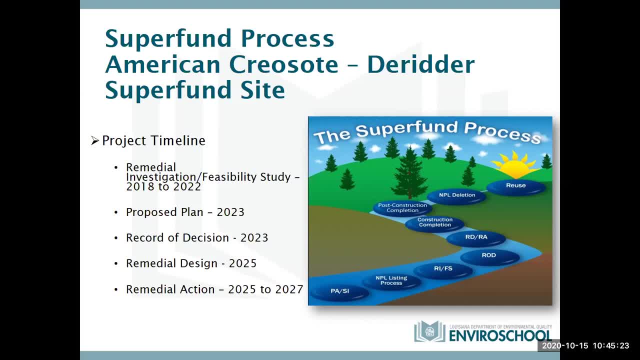 a bankruptcy of a company that was a successor of one of the PRPs here. It was called Tronox and EPA, the two sites in Louisiana that Tronox was a potentially responsible party successor for, And they recovered a good amount of money for each site from the bankruptcy of. 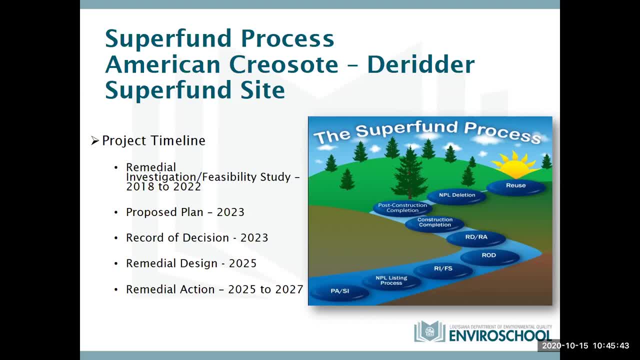 this company. So we have several million dollars for each site. So it will be partially funded by that bankruptcy. So now we can move faster because we have some PRP funding. We don't have to wait for budget monies to be available- Another thing that that bankruptcy made possible. 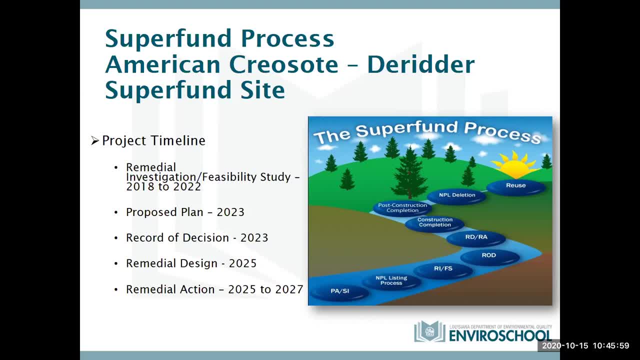 is. we are in the process of doing an EPA removal action on the site, One of those $2 million surface removals. We know we have to deal with creosote on the surface of the ground. There's no way to risk assess that away. It is waste. It is high concentration, So that will. 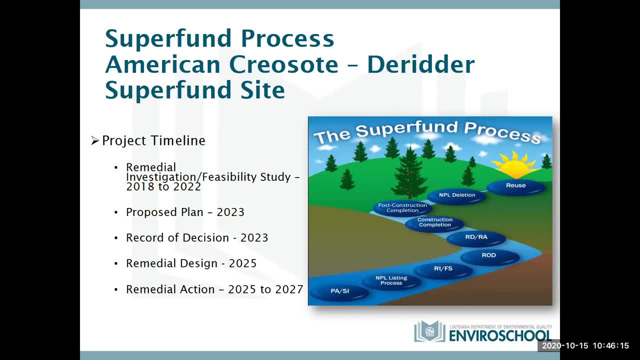 be removed and disposed of. That was ongoing Again. we're in the process of doing an EPA removal action on the site So that will be removed. when the COVID pandemic occurred and we had to stop. The material is still staged but we did not get to dispose of it before that happened. But we will continue that as soon as. 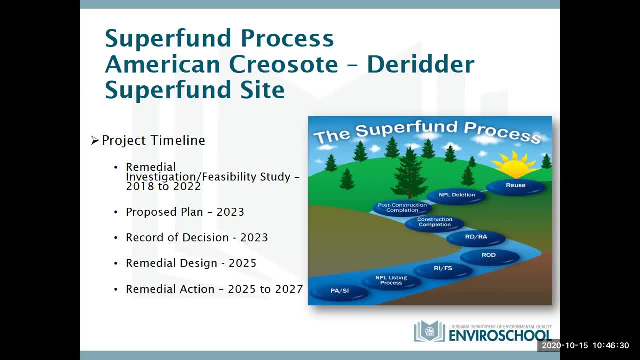 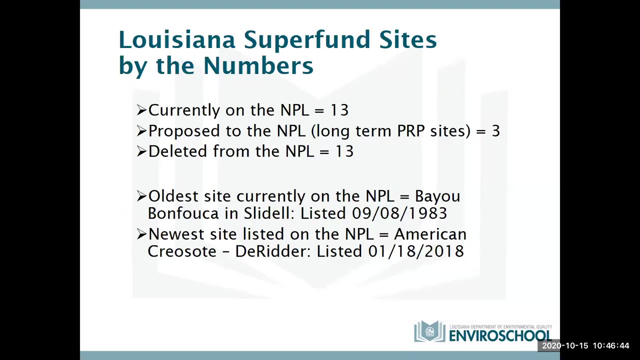 some of EPA's travel restrictions are lifted. They're beginning to get a little bit better over there in Dallas, So we're hoping that late this year, early next year, that we'll be able to resume that removal action. Okay, Tamika, All right, So that was our newest Superfund. 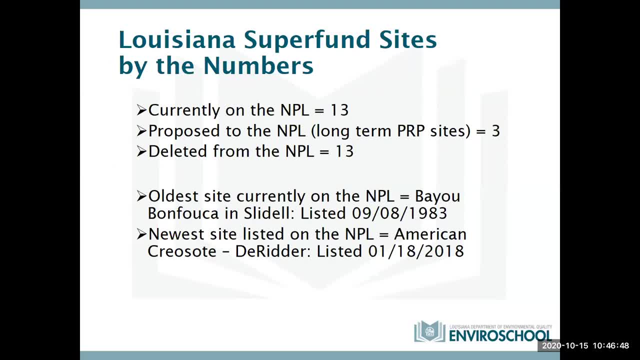 site in Louisiana, the American Creosote DeRitter site. But how many sites do we have in Louisiana? Where do they go? What kind of sites are they? I thought we'd talk about this in terms of the numbers. We'll play some Trivial Pursuit with Superfund sites here. So currently, 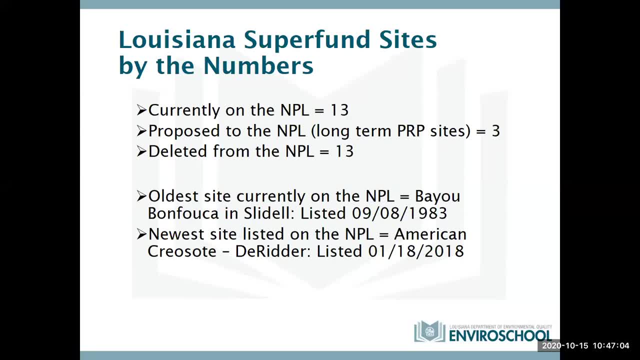 in Louisiana on the NPL, counting our American Creosote DeRitter, we have 13 sites that are listed on the NPL that we are in some stage of cleanup on. So this extends from the remedial investigation phase all the way through to a long-term remedial action. So we have 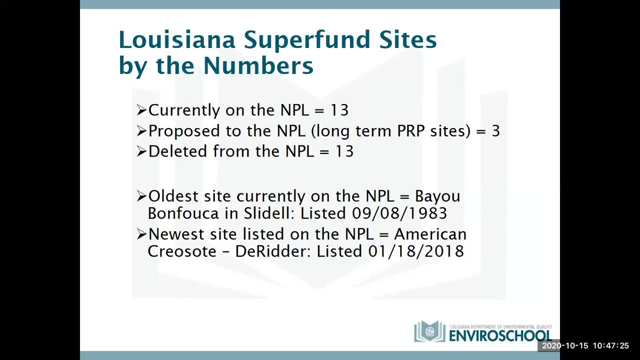 sites that are proposed to the NPL that are long-term PRP cleanup sites, but they were never listed on the NPL. So, if you remember, in the syllabus for this thing we said we'd discuss that concept and we will in a little bit. But we have three proposed to the NPL sites that are: 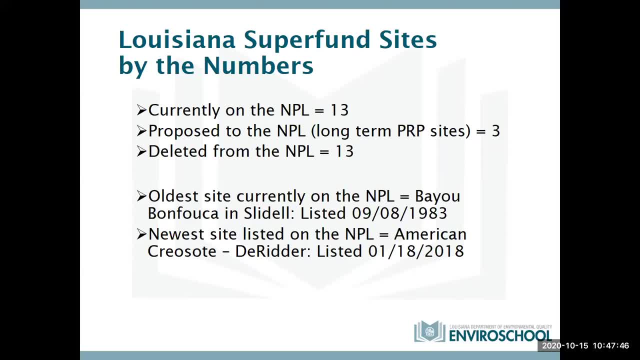 being addressed by the PRPs that are not listed on the NPL. So we have three sites that are being not listed Then deleted from the NPL. these are 13 sites that we have. See, this is CalBalance. We've got 13 going at 13 cleaned up, But anyway they're deleted from the NPL. They've been. 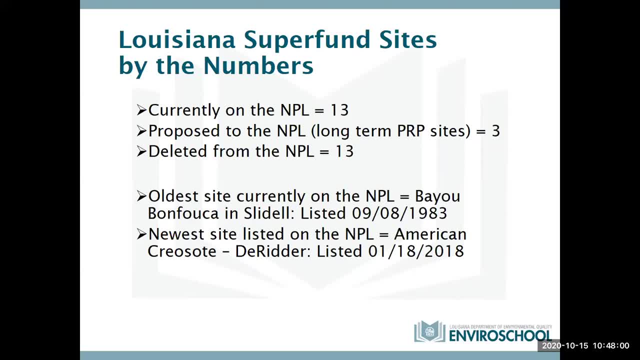 remediated. Two of them have been cleaned up completely and have unrestricted use, and then the rest of them are in some form of operation and maintenance of the remedy. So that can vary from active to passive. But let's talk about the oldest site currently on the NPL. 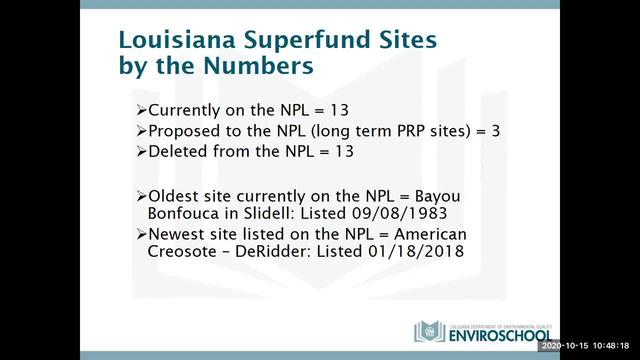 this is our famous site, Bayou Bonfuqua Superfund site in Slidell, Louisiana. It was one of the first hundred. It was listed on the NPL in 9-8 of 1983. It was one of those sites that the NPL was. 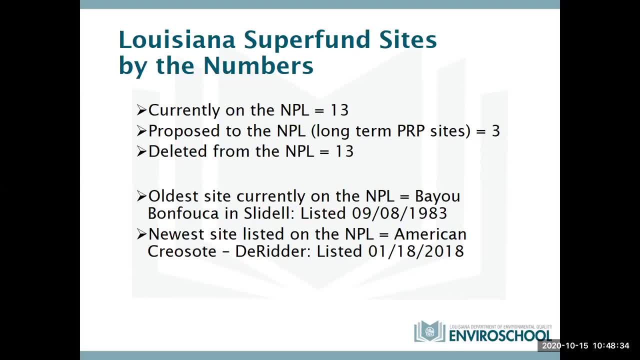 designed for, if you will. It was one of those that they said that needs to be on it And that was. it's a serious site. It was $160 million cleanup, So that is a big site. I still manage that one. We have a groundwater pump and treat operation going on. The newest site listed. 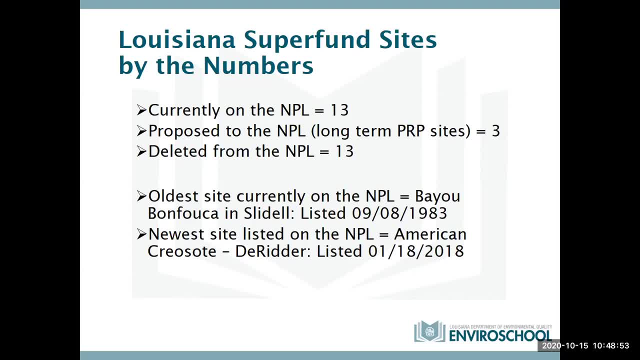 on the NPL, like I previously told you, that is the American Creosote DeRitter site and it was listed on 1-18 of 2018.. So that's where we range. So you know, I said in the syllabus that we would. 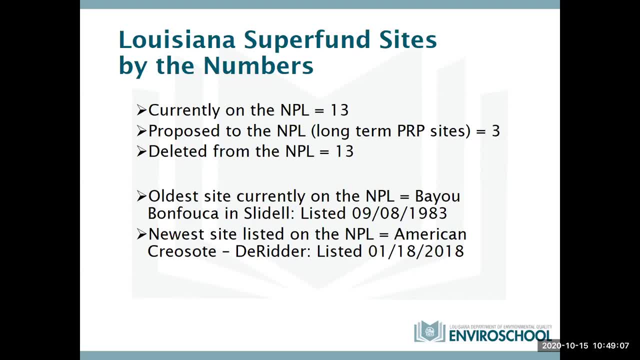 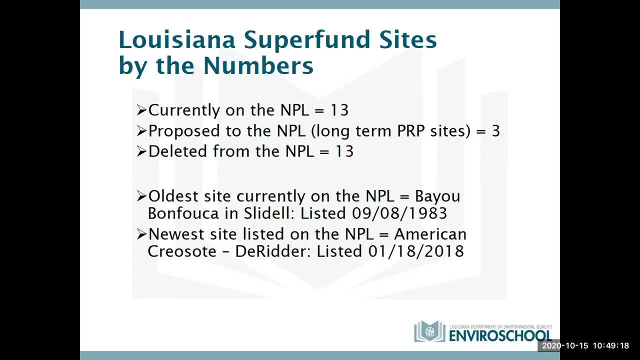 didn't qualify for the NPL for one reason or not, or maybe we didn't look at them closely enough before. Is it possible that we'll find a site out there that could be NPL caliber that we don't know about? Yeah, it's possible. You know, there's certain sites that didn't really get. 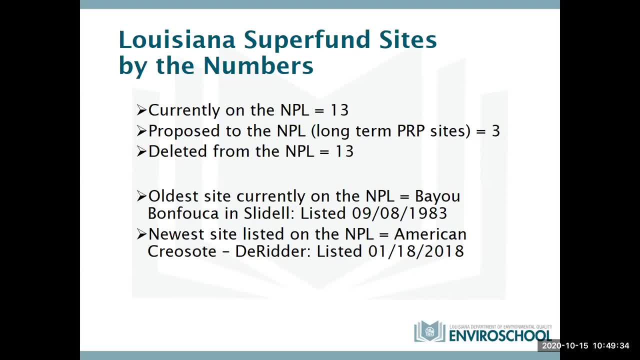 looked at much before. Our newest sites are like shipyards- Those kind of went under the radar before, but now we're looking at some of those historic shipyards that are closed. Our second newest site listed on the NPL is a shipyard- SBA shipyard. So 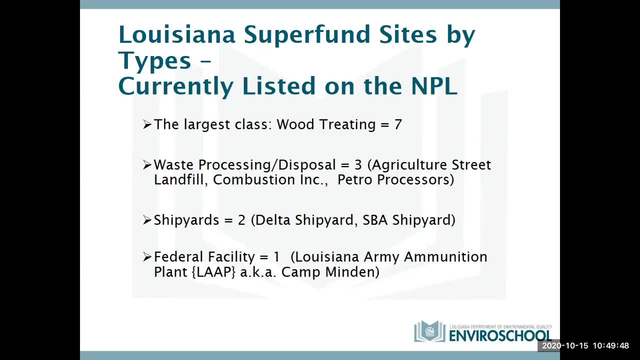 there may be more that we don't know about. All right, so let's look at the ones listed on the NPL, the 13 that we have currently listed. The largest class of sites in Louisiana that are currently listed are wood treating sites- Wood. 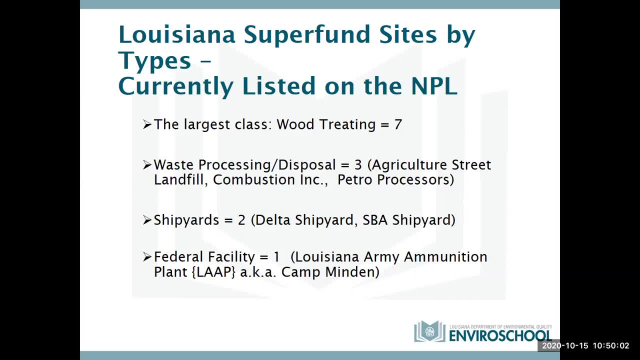 treating sites are always nasty and always a long-term cleanup. We have seven currently listed on the NPL, so that's where we're at Lots of them, and we talked about a couple. Next, most frequently listed on the NPL currently is the waste. 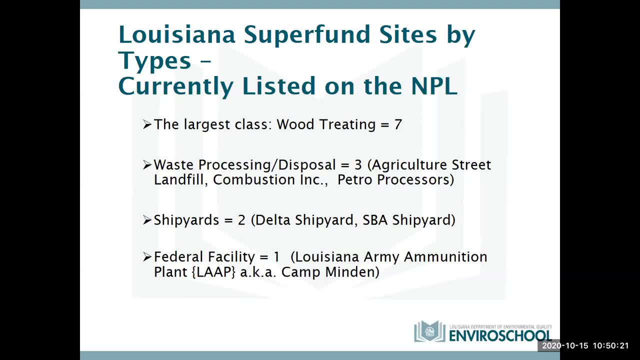 processing and disposal sites. There are three of those listed right now, all that were active on Agriculture Street, Landfill. Certain operable units are still listed. certain operable units have been deleted, but we have Combustion Inc, which is over in Livingston Parish, That one's currently in a phytoremediation. 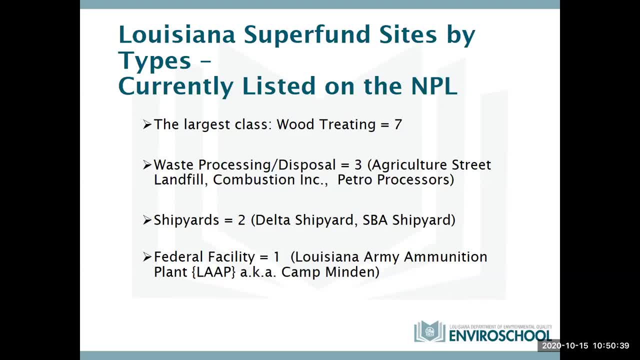 process. and then we have Petro Processors, which is north of Baton Rouge, in房s and canals, And that is in an enhanced natural attenuation and bioremediation process. So that's intermission. I like to say We have two shipyards. 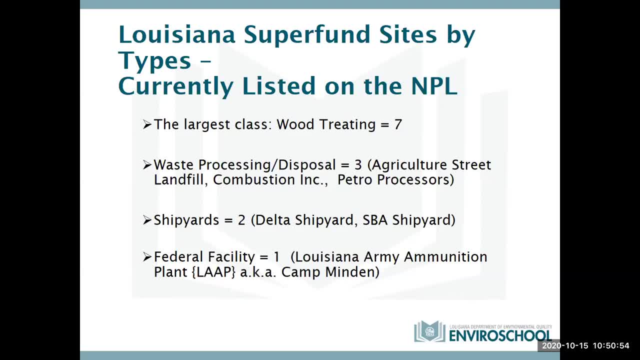 Shipyards are a growth area for EPA's food fund program. We've got Delta Shipyard and SBA Shipyard. These are both recently listed. They're the two that were listed most recently, except for the American Cree-South Territory. 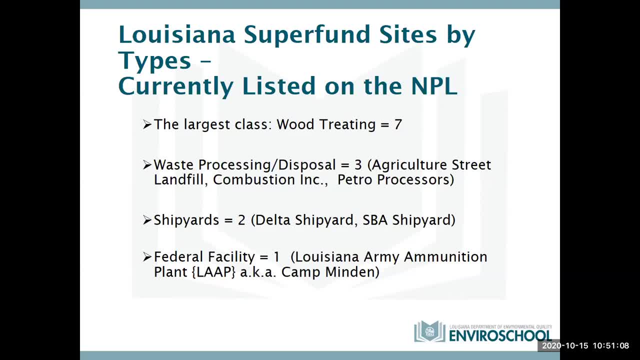 We have federal facility. We have one federal facility. Um, this is a site that the federal government is actually responsible for, And when we say federal facilities, it could be anything from NASA facility to- but you know, 90% of them, I'd say, could be a Department of Energy facility. 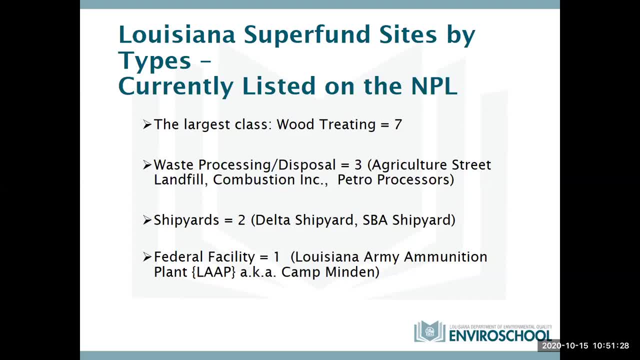 But 90% of them are probably military facilities nationwide. Nobody can mess up a site like the military, is what we say. I mean, you know, historically, before there were laws, you know the military used a lot of chemicals. They used a lot of explosives and other stuff. 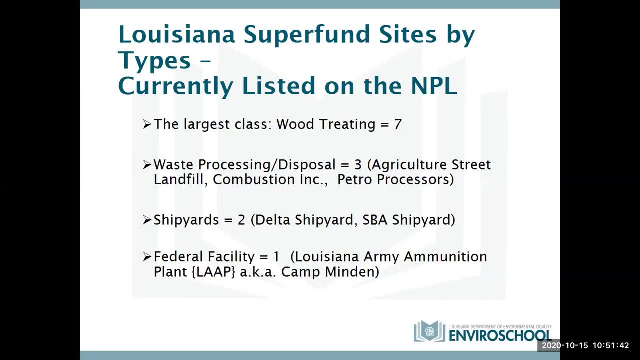 And you know, there were no laws against disposing of them on site, And often that's exactly what happens. So a lot of these have problems. The Louisiana Army Ammunition Plant has a number of AOIs that are under, you know. 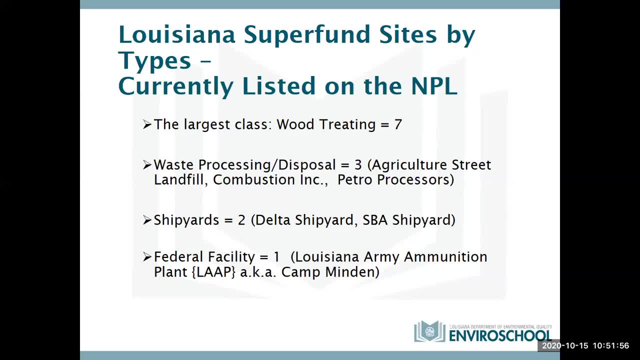 federal monitoring. Now we call this in Louisiana now Camp Minden. It's operated by the Louisiana National Guard, But the Army is still responsible for this. This was a big weapons plant for war And it's located up there around Doiling. 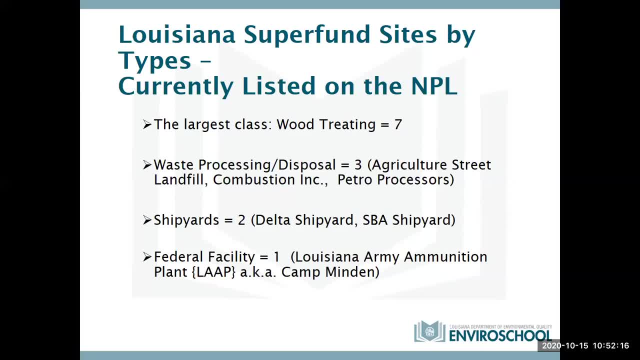 It's near Bossier. There was another one in Texas called Longhorn Army Ammunition Plant. That was a sister facility And these facilities made all the big bombs that were used in World War Two, you know, during the air war in Europe and Japan as well. 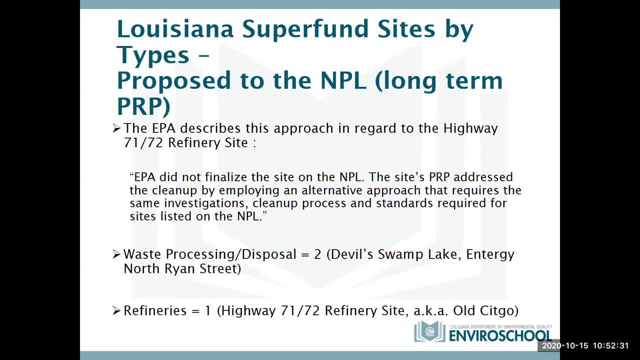 So they were explosives plants. So all right, Tomiko, Now let's look at what I told you. I'd tell you about the proposed to the NPL and why they don't get listed. So we have the one site up in Bossier that is proposed and it's never been listed. 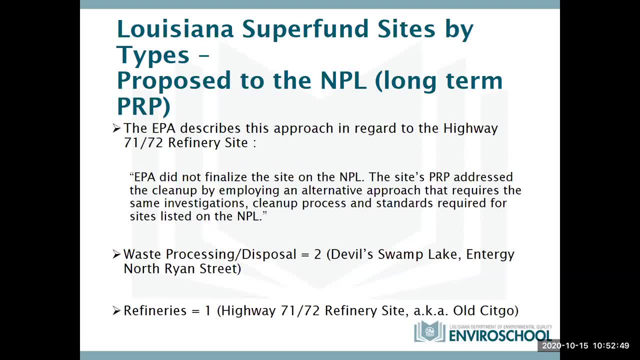 And it's called the Highway 71-72 Refinery Site. That's what EPA calls it. That's what's listed on the NPL and on the website says We call it Old Citgo. It's another name for it. It's in Bossier City. 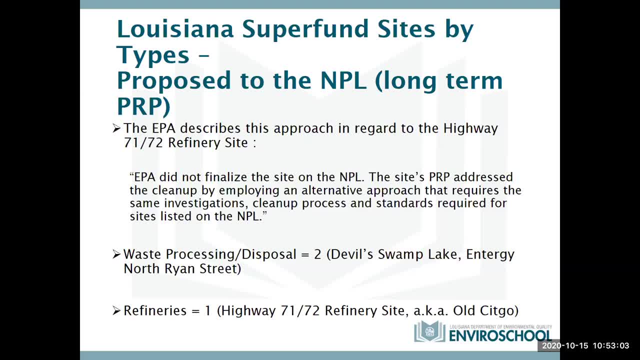 Well, it's really in Bossier City. It's under a lot of the downtown area there, So that that is The explanation of why it and the other sites are not finalized, And this is from a document that I cut and pasted. 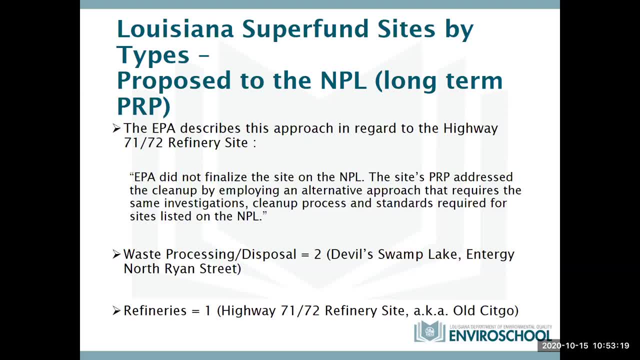 It says EPA did not finalize the site on the NPL. The site's PRP addressed the cleanup by employing an alternative approach that requires the same investigation cleanup process and standards that were required for sites listed on the NPL. So, as EPA proposes these sites to the NPL, 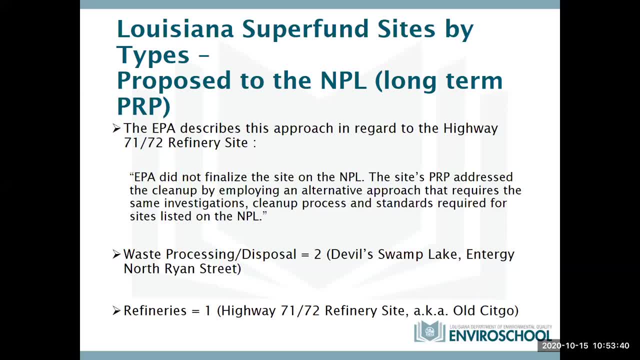 And then the PRPs enter into some type of cooperative agreement- or in EPA they call it administrative orders on consent- in order to clean up the site. So there is no need, in EPA's view, at that point to go ahead and list on the NPL. 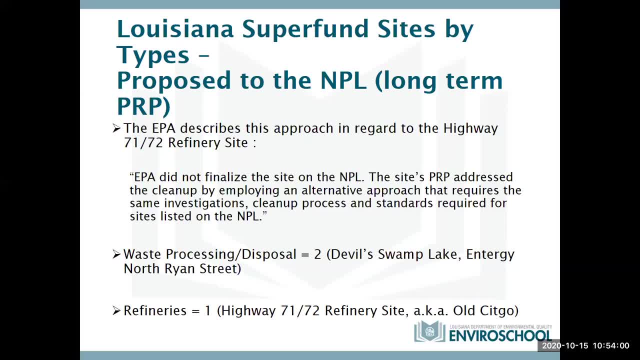 As long as the PRP enters into some kind of legally binding cleanup plan with EPA and everything continues to go Well, then there's no need to list it Now. had they failed to abide by the plan or whatever, then it could be listed on the NPL. 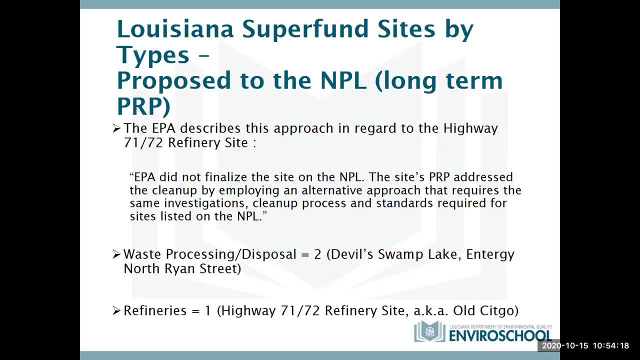 So all you have, it's proposed. All you have to do is: you know, step that up. It's kind of like drawing back your fist and saying: don't make me hit you anyway, All right. So then, other two sites that we have, and these are the Devil, Swamp Lake, Superfund. 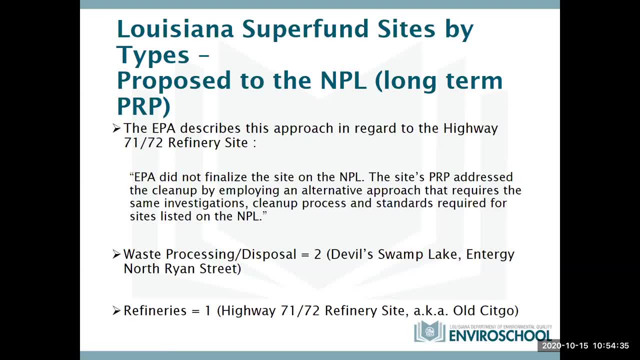 site North Baton Rouge, which is where PCBs were discharged in Devil Swamp Lake by Rollins Historically. and then we have Intergy North Ryan Street. That's a former coal gasification facility, an oil gasification facility on North Ryan Street. 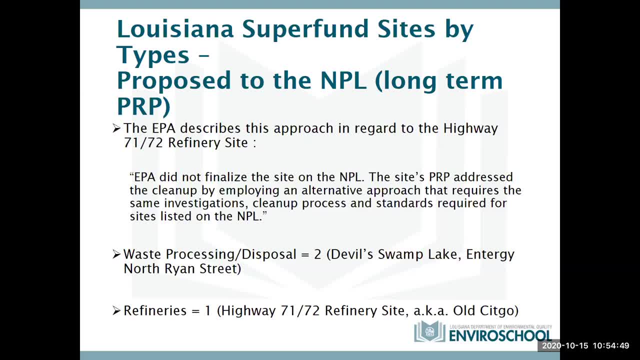 Also there was a lot of PCB disposal there. Intergy- it was run by GSU before Intergy and Intergy became the PRP when they absorbed GSU. So that is being addressed by Intergy and it's in operation maintenance at this point. 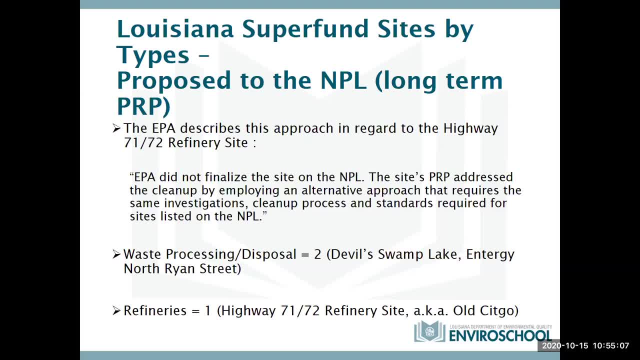 So it's proposed to the NPL, but never was necessary. It was not approved. So it's proposed to the NPL, but never was necessary. And of course we had the Highway 71,, 72, it was a refinery site and we discussed that. 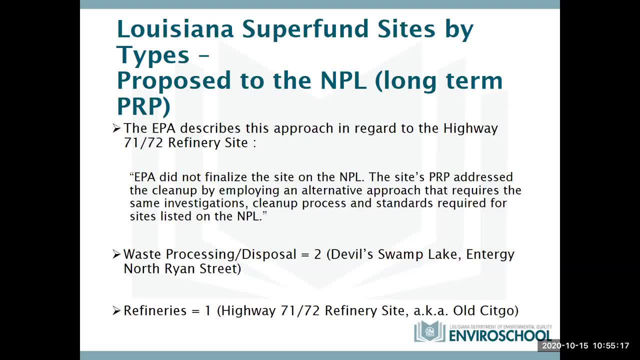 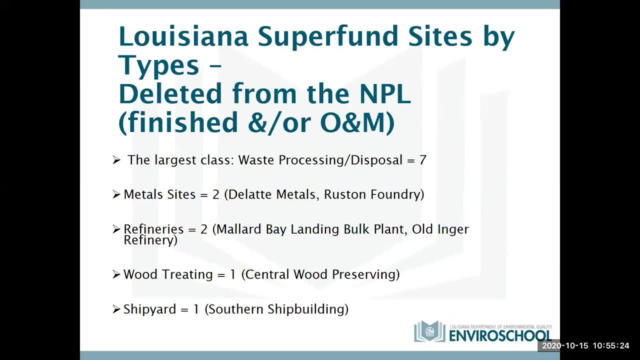 So that's our three, our three proposed to the NPL. Now we're thinking about deproposing the 7071 site because we're almost reaching all the remedial goals. So all right. So losing out Superfund sites by types. 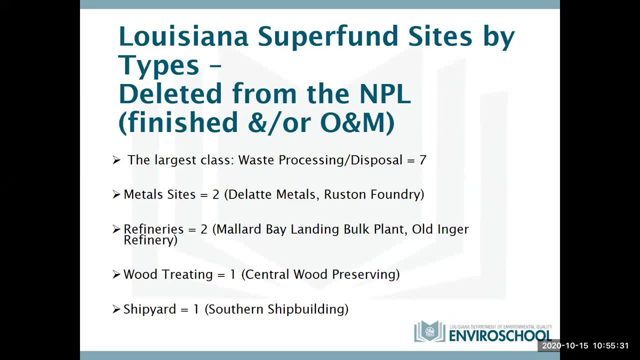 Now these are the deleted from the NPL. There are two that are finished and all the rest are an O&M. The largest class of site was the waste processing and disposal sites. There were six of them. There are seven of those, which is you know. there's a number of those that are scattered about. 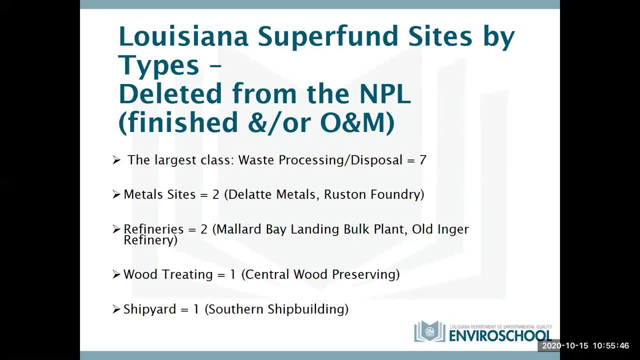 And then we have two metal sites. We have Dillat Metals on Ponchatoula and Ruston Foundry, which is not in Ruston, it's in Alexandria. I know the name is confusing, but the Ruston Foundry is one of our two sites that was cleaned up to unlimited use levels. 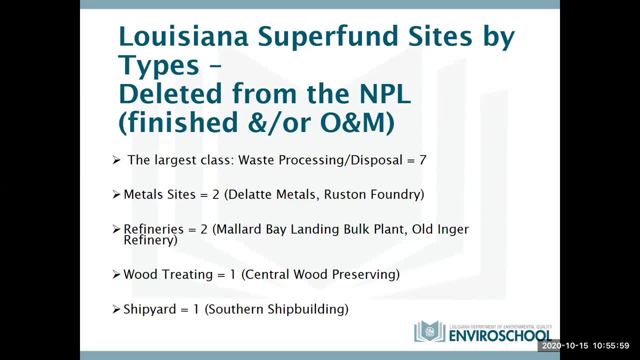 And so that's a great success story there- Our refineries. we had the Mallard Bay Landing Bulk Plant. That's another great success. We cleaned that up to unlimited use levels. It's safe for residential development If they want to. I don't think they will because it's at a landing on the intercoastal waterway, but you could if you want to. 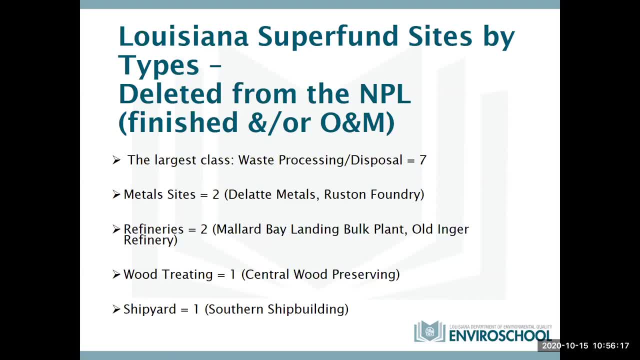 Then we have the Old Ingle Refinery, which was a state cleanup, and we are still in O&M on that one. We have to maintain fencing, all that Wood treating. we have Central Wood Preserving. that is finished, It's in O&M and the parish actually is conducting O&M there. 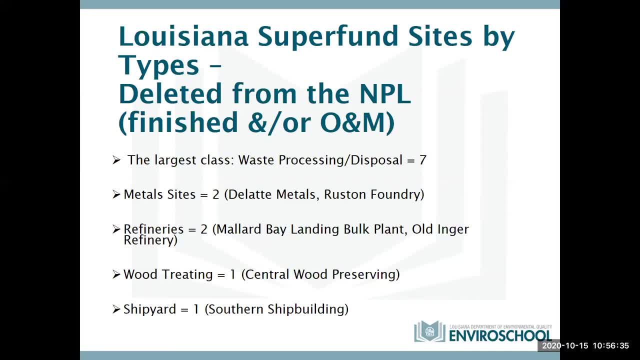 There's a capped area and a fence and they maintain that Shipyard- one Southern Shipbuilding. this has been redeveloped and it's in private ownership now. Port of Slidell Corporation runs that now and they maintain and operate the site. 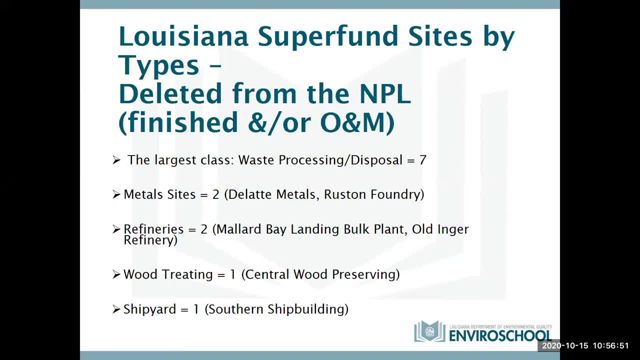 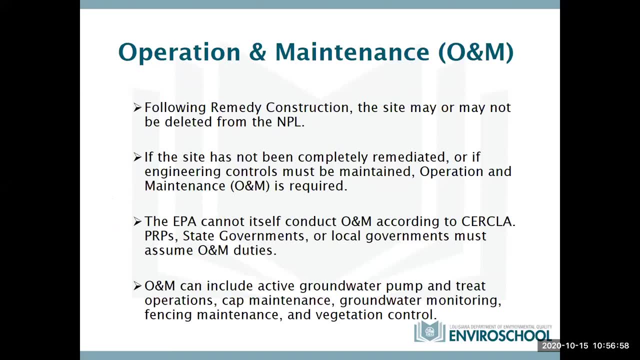 So those are deleted. So they're in O&M. All right, Tamika, All right. so let's talk about that concept of O&M, or operation maintenance. You know these Superfund sites, they're the worst of the worst. 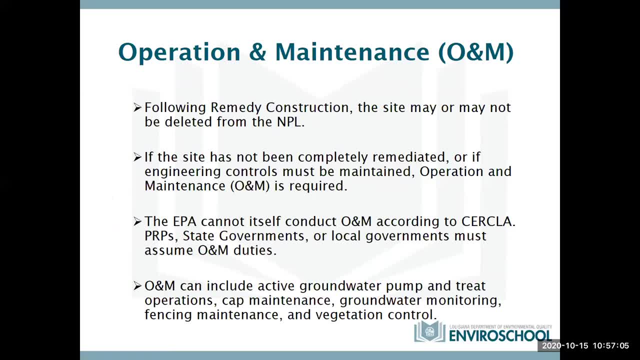 They have big problems. Some of them have big cleanup. Sometimes it's not technical. Sometimes it's not technically possible to completely clean up the site. You know we like to do that where we can. Sometimes it's not technically possible and sometimes it's not financially possible. 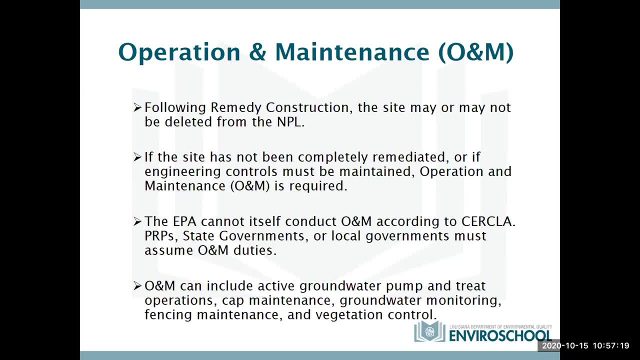 You know, Bayou Bonfuca cost $160 million to clean up the surface. It was incineration of a mile of bayou sediment- and they built an on-site incinerator- hazardous waste incinerator on-site- and operated it for a number of years. 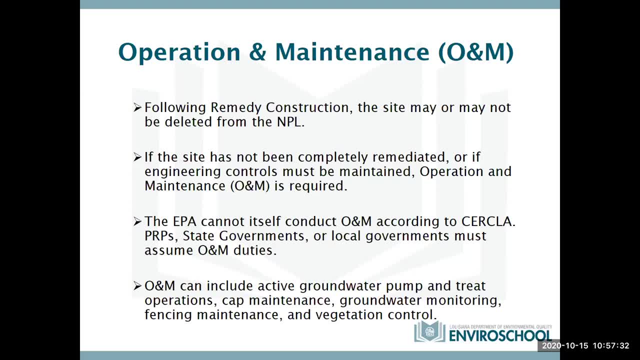 And we cleaned up the surface soil, We cleaned up the bayou sediment, restored Bayou Bonfuca to its- you know- ecological conditions, even lifted the fish advisory. now It's safe to fish there. So a lot of work was done. but subsurface soil and groundwater, that would have cost gosh knows how much more. 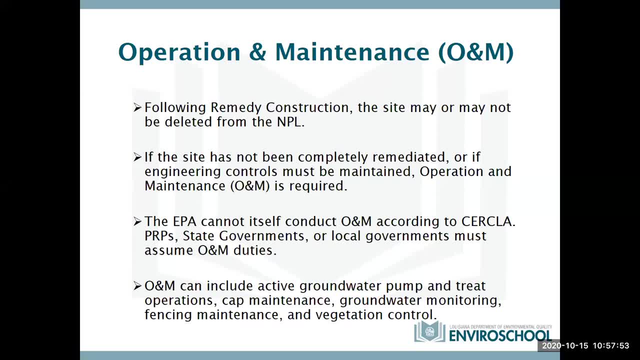 We have been pumping and treating that groundwater ever since the cleanup was completed in the 90s and we will be from now on. As far as I'm concerned, I don't know if we'll ever get there, but that's where we're at. 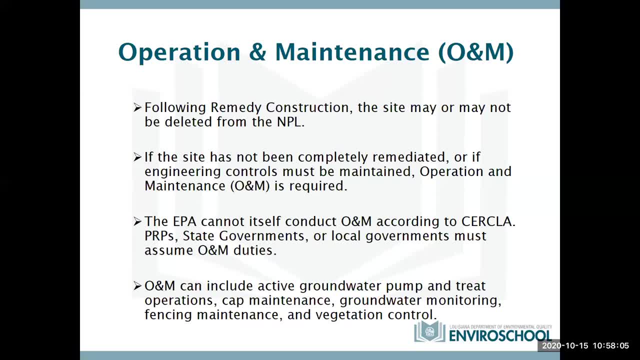 But following the remedy construction, the site may or may not be deleted from the NPL, And that's an interesting concept. Sometimes they're not, you know, sometimes they go into LTRA or long-term remedial action. Our American Creosote Winfield site is in long-term remedial action. 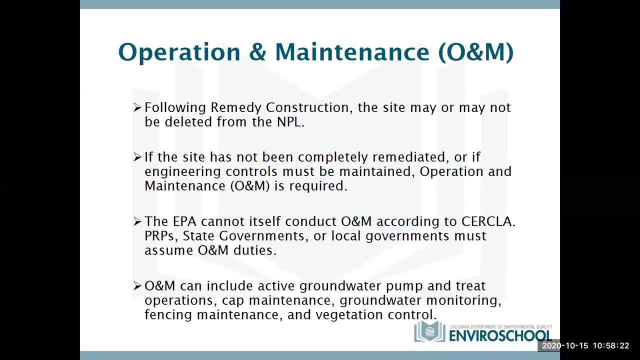 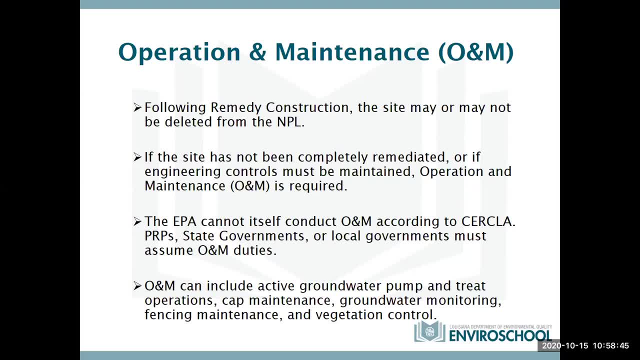 So that's an important part. We in the state pay $300 million pump and treat a year on that particular site. That's the one. we in the state pay 10%, So that's a good point. I haven't made that point before this. 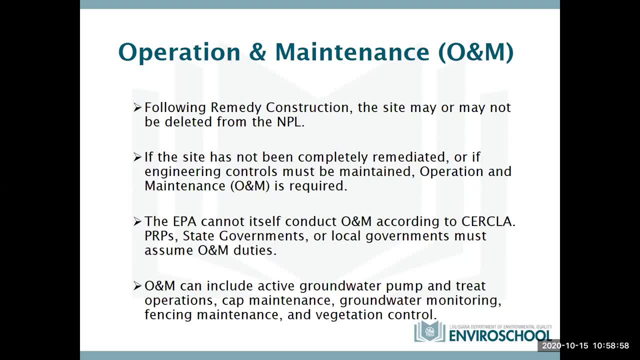 But before we get to O&M, when we do the remedy, EPA does all what's called pipeline costs. They do the PA, they do the SI, they do the RI. you know great, you know the PRPs pay. the taxpayers of the state of Louisiana and of the federal. 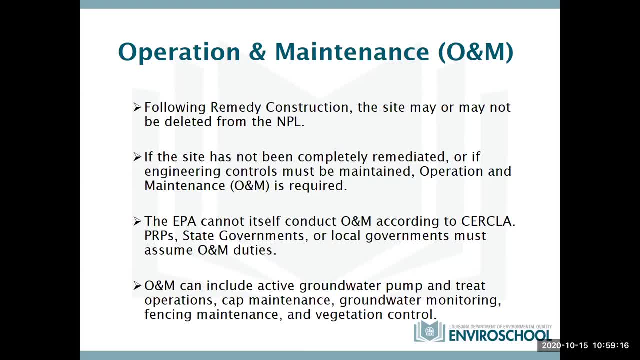 government. we have some overlap there. we we are not, you know, tapped for that. so that's great if there's PRPs, but if there's not, then EPA pays 90 percent of the cleanup costs from the remedial action to O&M. so the remedy itself: EPA pays 90 percent on the orphan sites and the state has to. 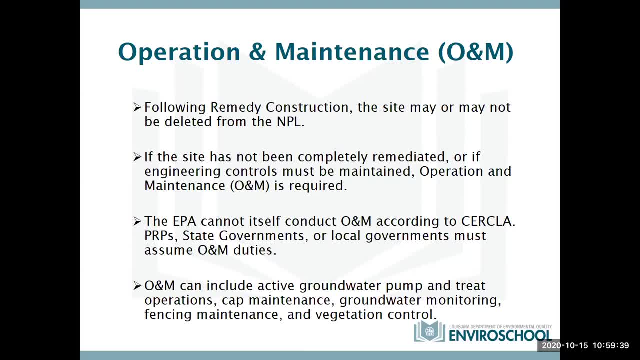 match 10 percent. so you know, on that Bayou Bonfouque, 160 million dollar incineration, the state had to come up with 16 million dollars, which you know, if you look at 10 percent is a pretty good deal, you know, but it's still 16 million dollars. go to the legislature and ask for 16. 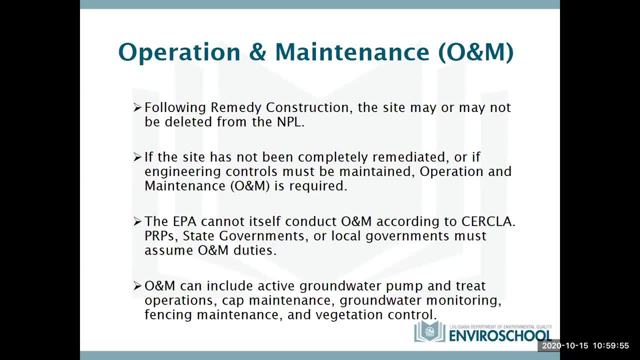 million dollars. that's a hard sell, but uh, anyway. so but this changes. when a site goes into operation and maintenance, okay, someone else has to pay for it. because the EPA cannot conduct O&M according to CERCLA, the PRPs, the state governments or local governments must. 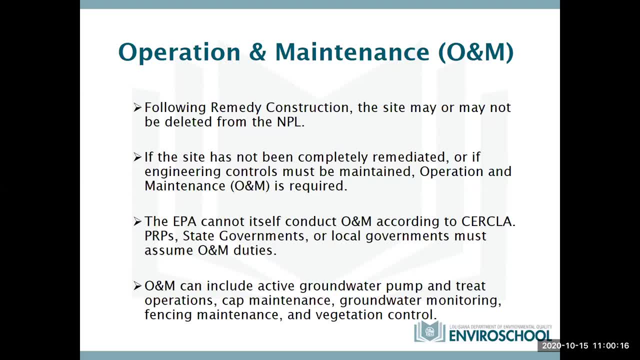 assume O&M duties. so if there is a long-term remedial action, that's a different thing. but whenever we delist a site, we take it off the NPL, then it goes into O&M and somebody else has to maintain that site. so if we do delete it then and there's O&M, then 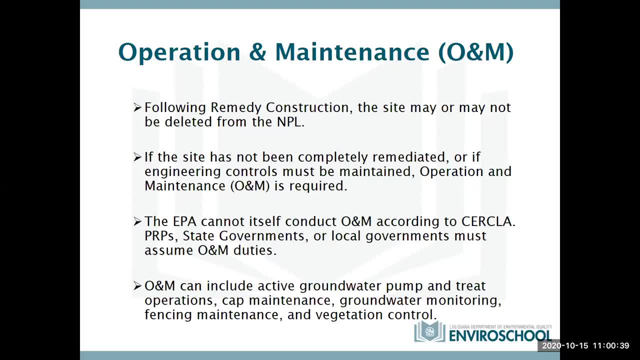 we have to go in that now. uh, if site's been completely remediated, you know great awesome, if we've completely cleaned up everything, it's unlimited use, then there's no O&M. but if it has not been completely remediated or we have some type of engineering controls like a cap or a, 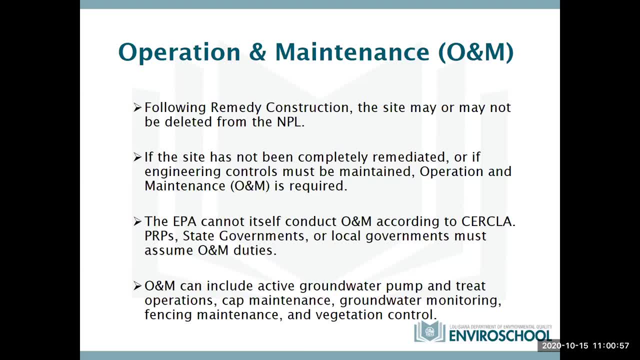 groundwater treatment system or whatever it may be, that O&M is required. and so- and I've mentioned that, we have some PRPs, we have private landowners, we have the state government, which you know, we have three, three or more sites that we're doing O&M. it just varies um three active O&M. 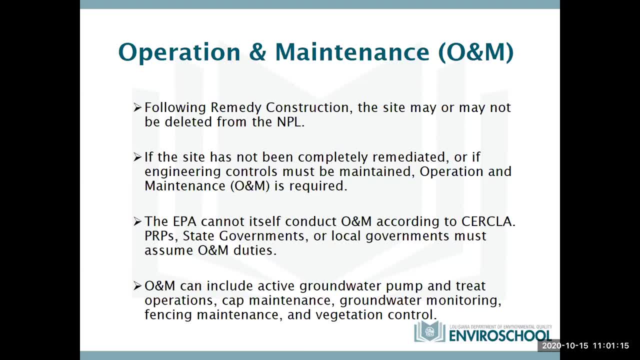 and some are passive O&M and then in some cases it's local governments, like I say. you know, East Feliciana Parish take care of central wood preserving. so um, now O&M can be anything from active groundwater pump treat. it could be other kinds of remediation systems. um could be cap. 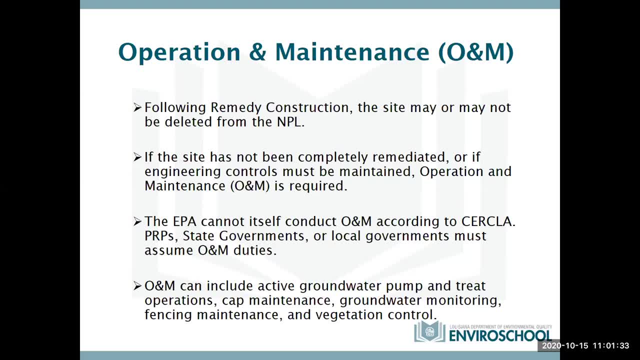 maintenance. maintaining that clay cap put over contaminated soil could be groundwater monitoring. maybe we're just monitoring it could be other kinds of remediation systems. um could be cap monitoring the groundwater every so often. uh, maybe we have to maintain some kind of fencing, maybe we have to do vegetation control. we have to mow that cap a couple times a year to make sure. 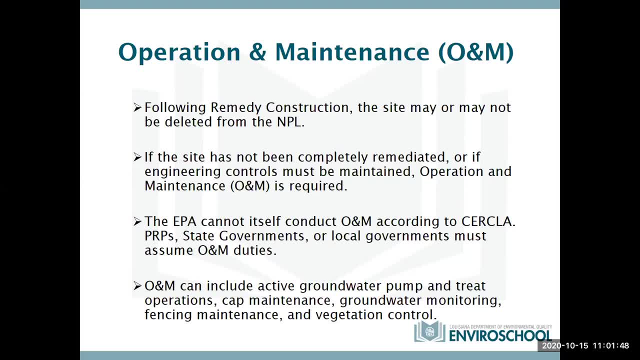 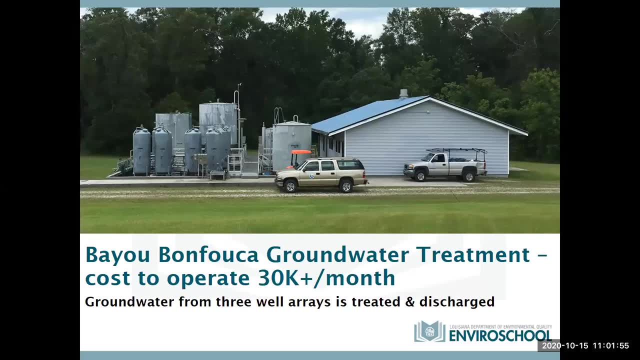 that it does not grow trees. that will compromise its integrity. so, all right, Tamika, great. now here is the Bayou Bonfuca groundwater treatment system. um, this is, uh, oh, this is a big thorn in my side. uh, this one is an active pump. treat at that Bayou Bonfuca super pump. 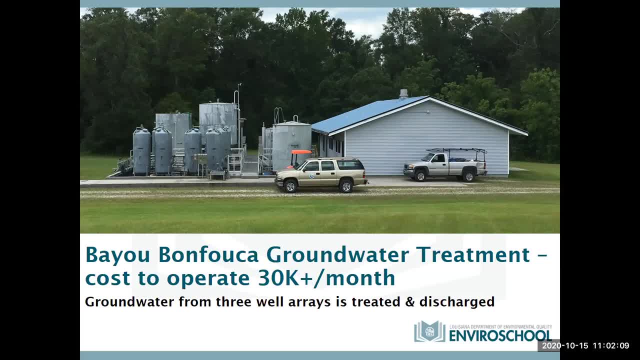 site. at the time I made up these slides, it was costing us approximately $30,000 a month for contractors to operate this for us, because that includes two full-time employees that are maintaining the facility operating the groundwater treatment. there's three well arrays, one's in a. 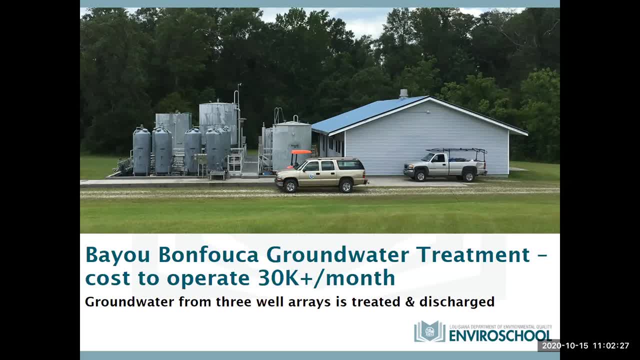 neighborhood across the bayou pumping creosote out of people's yards. uh, there's two of them. they're on site that's controlling the plume, keeping it from moving and trying to bring it back in and get it cleaned up, and we're going to be doing a lot of work on that, so I'm going to 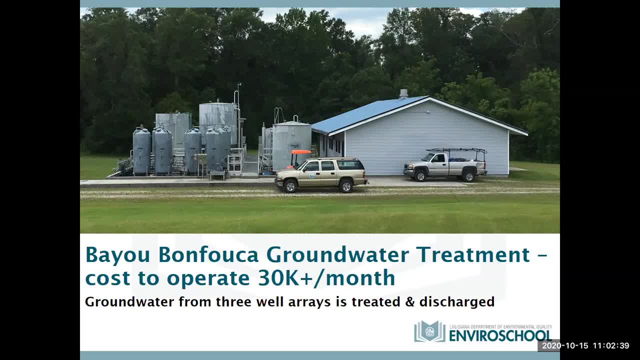 talk a little bit more about that in just a moment. and then the creosote is in this facility, you see, in front of you, the creosote is filtered out through a combination of oil, water separators, sand filters, and finally, by the resulting water, is polished through carbon filtration. and then 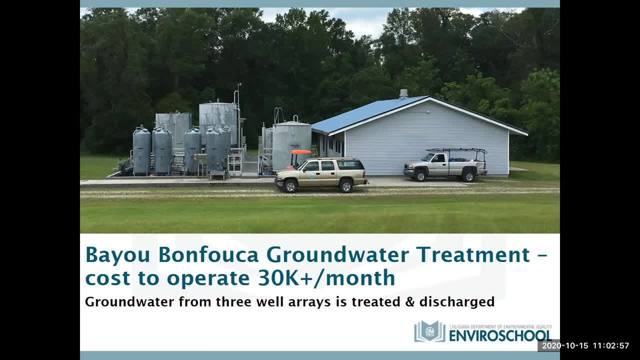 is discharged back to the bayou under a water discharge permit like limitation. so it's cleaned up to the what groundwater is cleaned up to a point where we can discharge it back to the bayou, and then we're going to be doing a lot of work on that, and then we're going to be doing a lot of work on that. 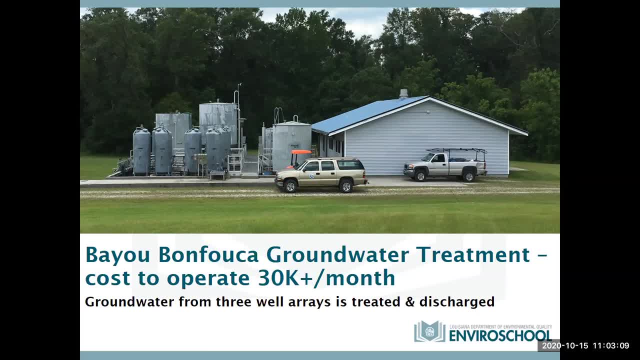 and uh, it's. it's quite the thing. it was a state of the art in the 1990s when it was built, and I think it was 2002. they handed the state of Louisiana the keys and said, okay, it's OEM now, and now you're. 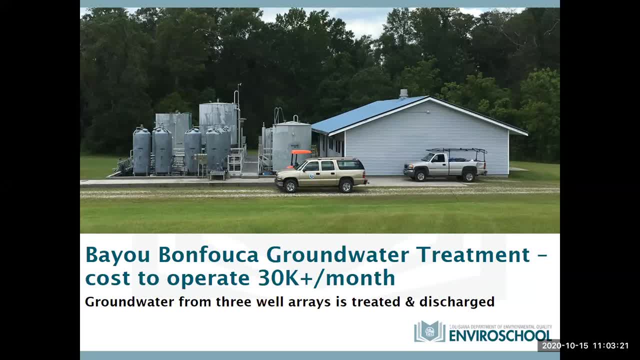 responsible, and so we will be responsible for this particular site until we reach the cleanup standards, which are the maximum contaminant levels for groundwater. EPA cleans up groundwater until it's drinkable, so that's that's the cleanup standard we have to apply to this site, and I don't know that we'll ever reach it, uh, but we're. 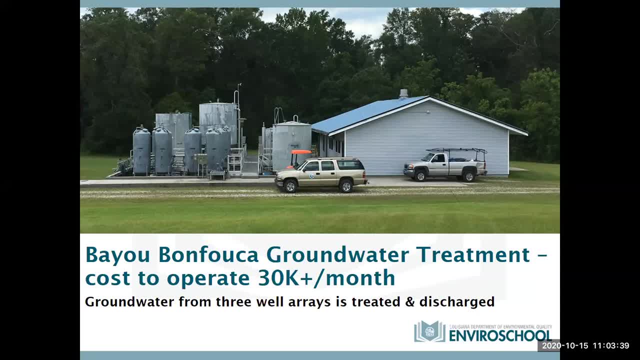 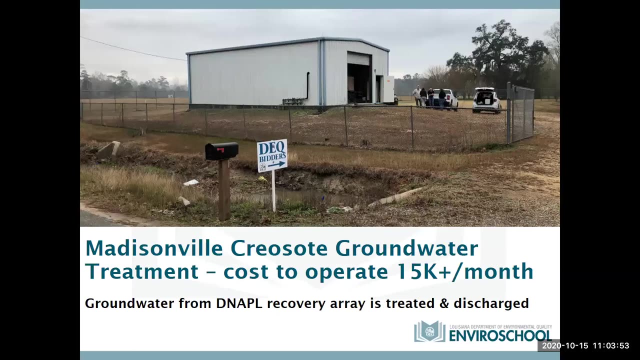 we're bound to do so. we may consider trying to change the rod or something to look at some other options down the road, but at this point that's what we pay. so all right, next slide. here's another active pump and treat that the state of Louisiana has a uh obligation to, uh well, I don't know if it's. 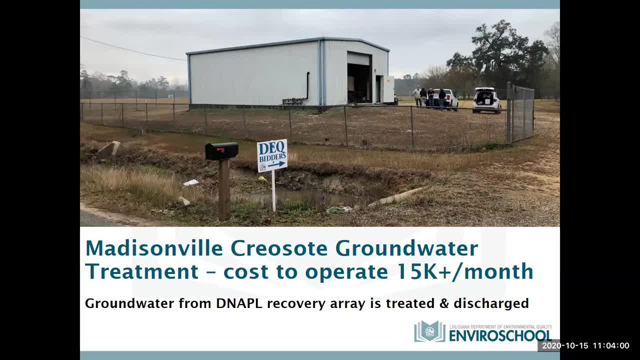 really pump and treat. it's more of a passive denaple recovery system. there's sort of a herringbone french drain system under the Madisonville creosote uh superfund site. um, this was an earth site where thermal distortion was used to clean up surface, but the subsurface 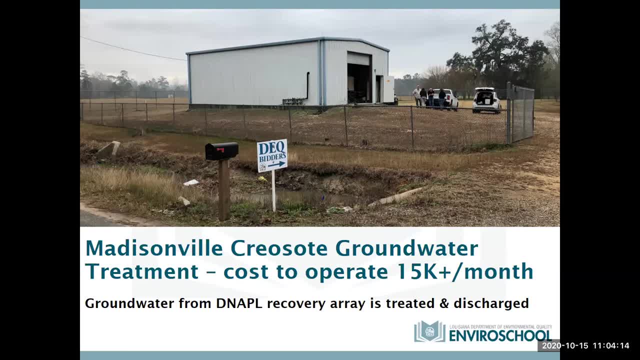 has some uh lenses have creosote and contaminated groundwater. so the groundwater is collected in denaple recovery array and then it's pumped into this nice metal building that you see in front of you and then, um, it is treated and then discharged into this ditch by the road that you see uh. 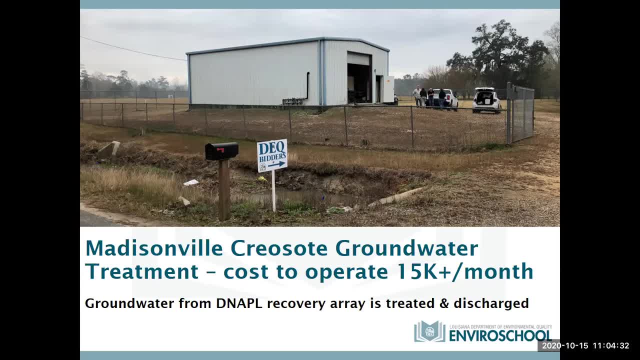 everything looks dead out there because this was taken in January and, uh, I don't know if you remember the name of this one, but it's a pretty old tree. it's a giant live oak tree. it's a historic tree that's actually on the register of historic live oak, so that's kind of a everybody likes to. 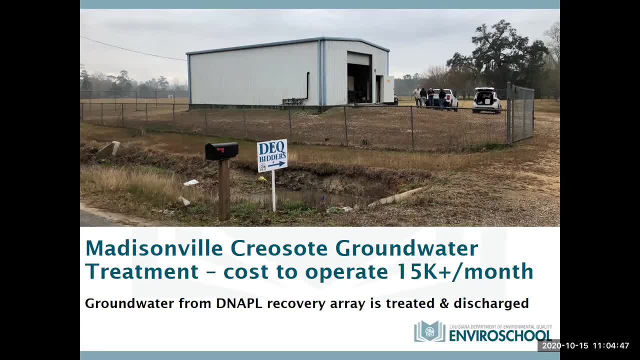 you know, enjoy that while they're there. it's quite the the large and old tree. so this particular site, uh, you see in front of you the sign by the mailbox. it says DEQ bidders. we bid this uh contract to operate the site out every three years, uh, to try to get the best value for the um. the um, you know. 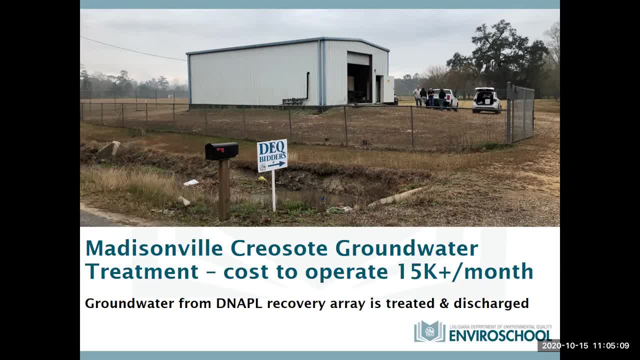 and, uh, consequently, uh, the taxpayers. and so, at this point, uh, it was 15k a month when, uh, this slide was made. we've had a second, another bid since then and, I'm glad to say, it went down several thousand dollars a month. so we're getting a better deal now. we had more competition on the. 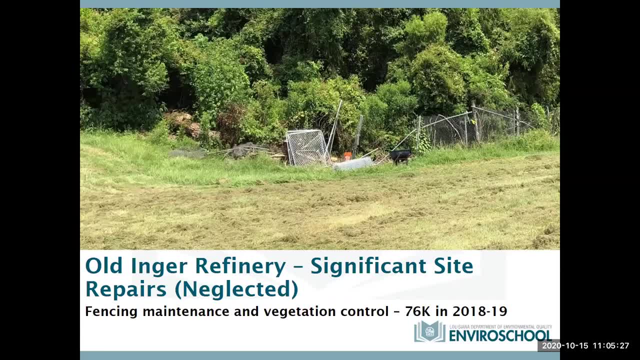 bidding. so that's great, all right to me. now this is the old inger refinery um. this particular site is another type of O&M. this one had, um a capped area and it vegetation needed to be controlled on that capped area. you can see that it's been mowed in the foreground um and the. then it was supposed to be fenced to prevent access. 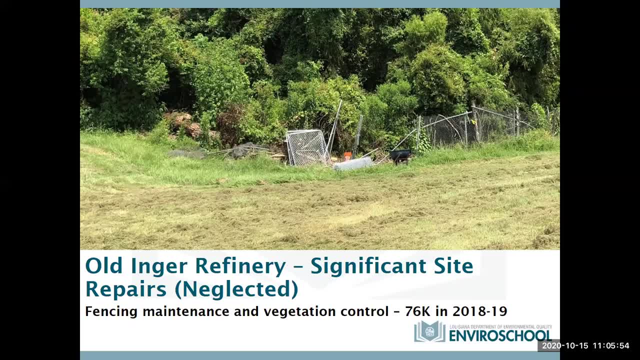 and that's all part of the O&M that's supposed to be done. the unfortunate thing is uh that, you know, during our various budget issues that we had, uh some years ago, uh the you know the fencing was not doing so well and during that time of neglect we had hurricanes like Katrina and Gustav. that uh. 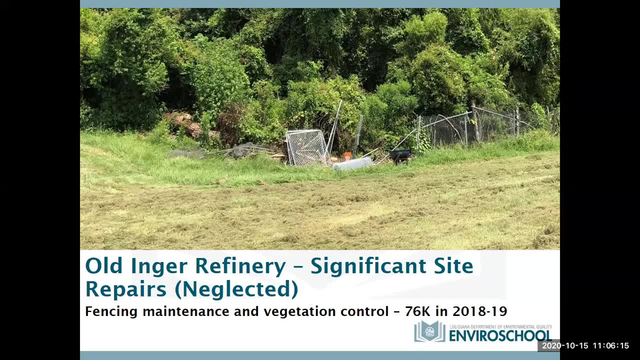 knocked over some of those big trees you see outside the site. uh, this is over, uh, near the Batchelor on the Mississippi River. so you get some really big trees and some of those trees. you see some wood in the picture. they fell on the fence and damaged it and took it down, so that was the 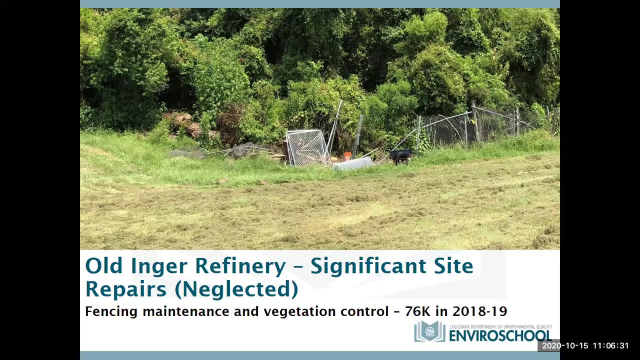 fencing condition, as you can see it there's poor, and so we paid in 2018-2019, about $76,000.00 to repair fencing. so, uh, we kind of got a bad review from EPA on a five-year review on the site because we were not keeping up our end of the O&M, and so we're trying to uh fix that up, I think, at 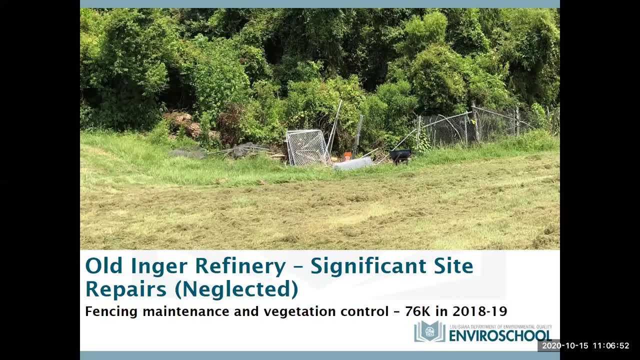 this point on: uh, we just had an inspection and Delta didn't knock down any more fence, so we're good and we we have repaired it all. it is in all good shape now. now we just have to keep it that way, so we're going to try to keep it up. all right, all right, so now let's. 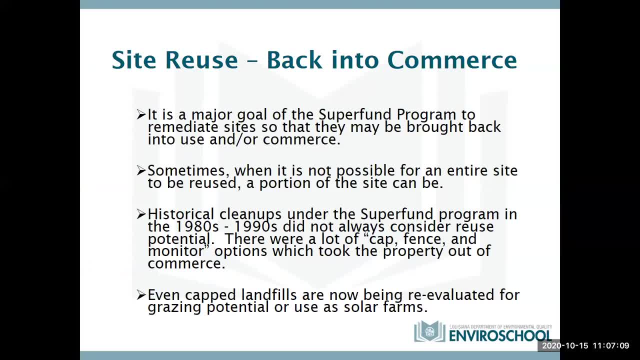 talk about that last step. you know those green hills and EPA's diagram: site reuse. we want to bring the sites back into commerce where we can. it is really a major goal of Superfund program to remediate sites so that they can be brought back into use or in commerce they can be used again. 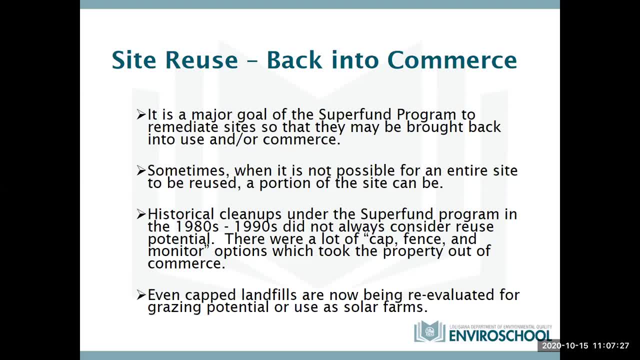 so this is one of the things EPA strives to do wherever possible. sometimes it's possible for a portion of the site to be reused and while the other portion of the site is not reused because it's still undergoing some remediation, we had that Bayou Bonfoucault Superfund site. a portion of the site was cleaned up to the extent where it could be. 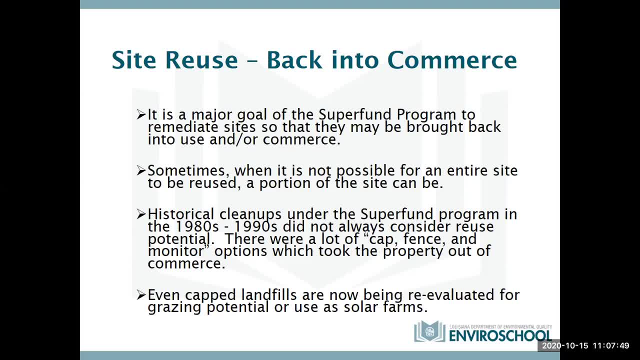 used as Slidell's Heritage Park and we'll look at some pictures of that in a little bit. other examples we'll look at include downtown Boulder, now historically under the Superfund program. back in the 80s to the 90s they didn't really always consider that reuse potential. they didn't. 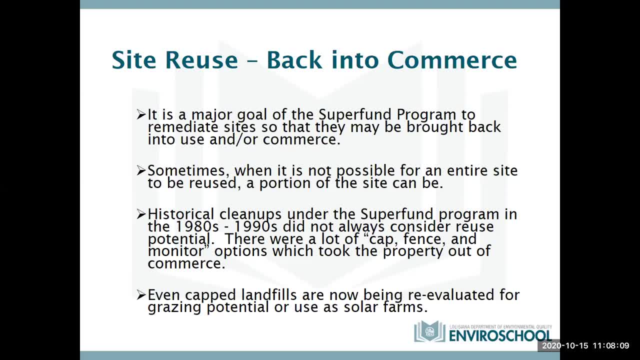 look at that, bringing it back into commerce. you know, I think the brownfield initiative and the voluntary remediation program. we started trying to clean up things so that people could reuse them again. instead of developing new land to be another industrial site, let's use the industrial sites we already have. so there were some cleanups that involved cap fencing and 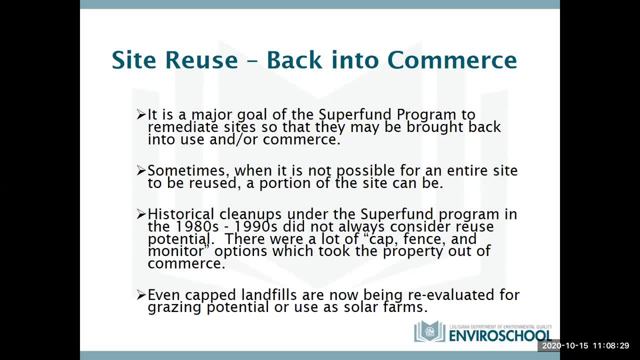 monitors. you know, we'd put a big cap on it. sometimes we'd build a landfill on the site to address the waste. we put a fence around it, we put some monitoring on it, we put some monitoring wells and we say, look, we cleaned it up, we remediated it and we did. but a lot of times 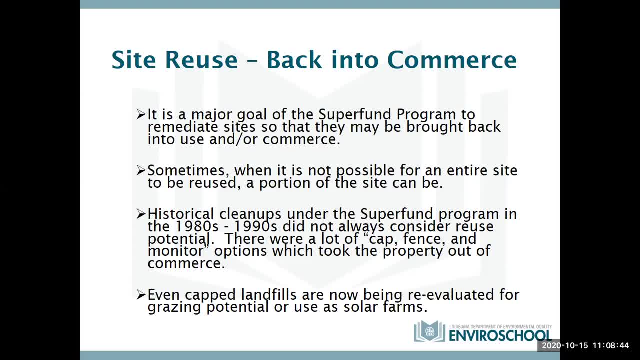 you know we stopped exposure. you know we reduced the risk, but did we make it possible for that site to be reused? well, not always. you know we got a number of those that, uh, you know that's what we still have. we've got a landfill that's capped and got to be mowed a couple times a year. got 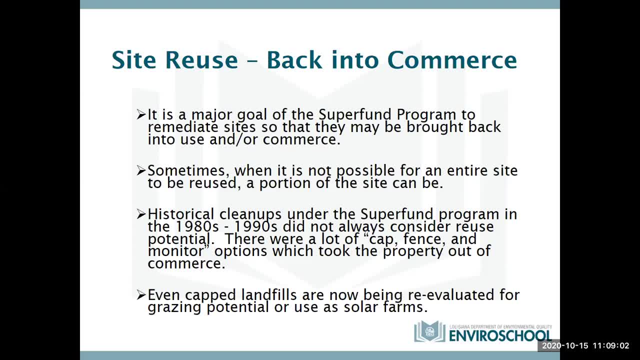 to be monitored, and nobody really wants to use it for anything, so not too good. those took the property out of commerce. sometimes that was the only feasible way to do it. sometimes that was the most cost effective way to do it, but it didn't help us with the reuse. um now i will say, though, that capped landfills are 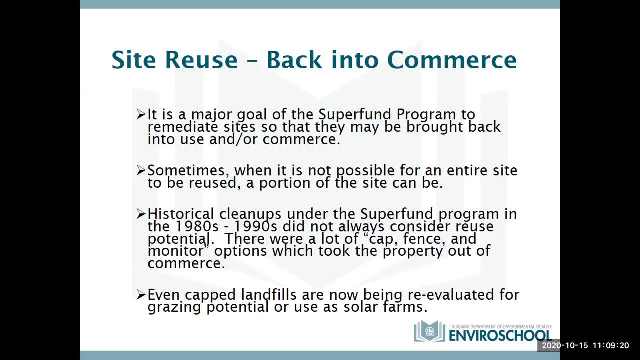 sometimes being re-evaluated for other uses, whether that's grazing potential for animals, you know, uh, get you some sheep or cows or something um, or as solar farms. uh, you know, putting solar panels on big uh frames that stand up above the ground. so if landfill settles or moves, 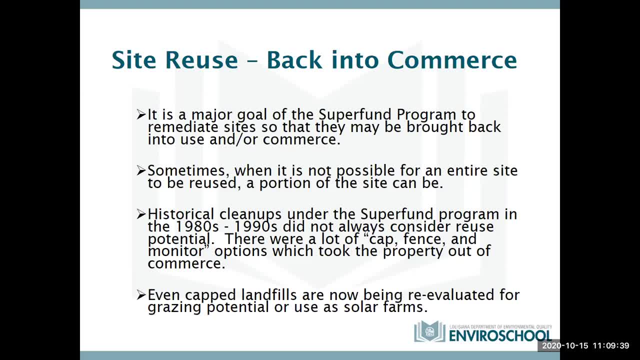 you know it doesn't matter, and underneath it you can still graze your sheep. another big thing on these landfills and cap sites is what we call pollinator meadows. you plant them with, uh, perennial plants that are good for a wildlife and, uh, you know, insects that pollinate our crops as. 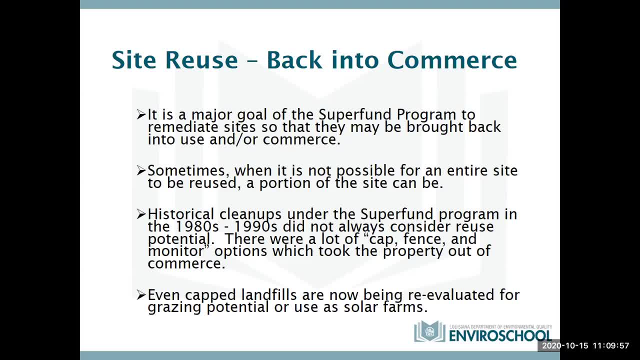 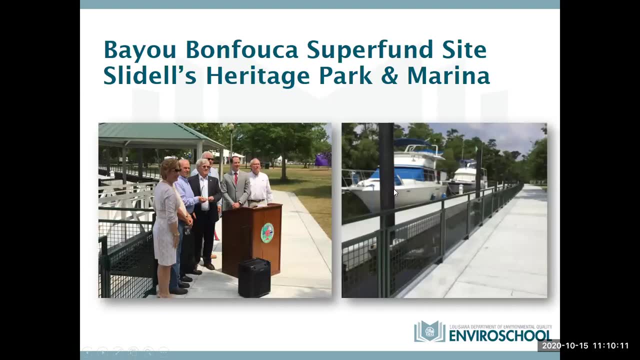 well, as you know, native plants and you try to grow these things up to, you have basically sort of a native prairie, um, growing on the landfill and this is great because, uh, i just recently uh sat in on a nationwide pollinator and then we got a pollinator that hit that first one. that was a. 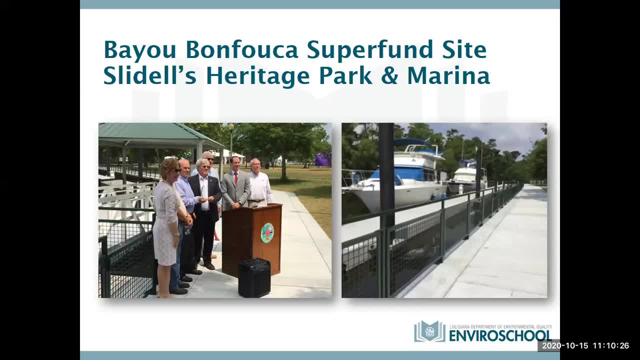 population-based pollinator. so that's for sure. good, um, um, all right. finally, uh, after all this, we're not going to run out of time. it's probably not people's pleasure to get into the den of the lab, uh, to get into the lab of a le monitoring lab where we're going to be doing some NPF. 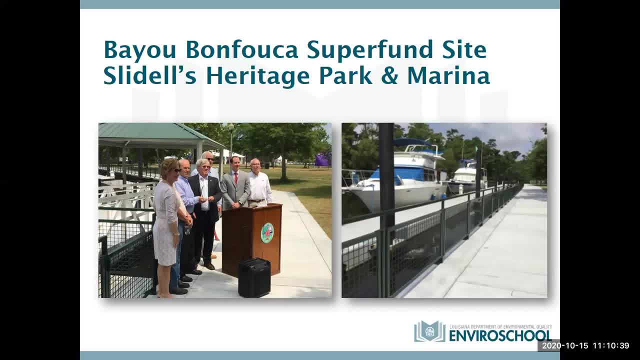 testing and other things. um, you want to get in there and get a little bit more information so you can. It's a clear one. you can't see it but the mayor of mayor at the time of Slidell was holding it. But they redeveloped the portion of the Bayou Bonfoucault site to be a park. that's one of the most heavily used areas in downtown Slidell. 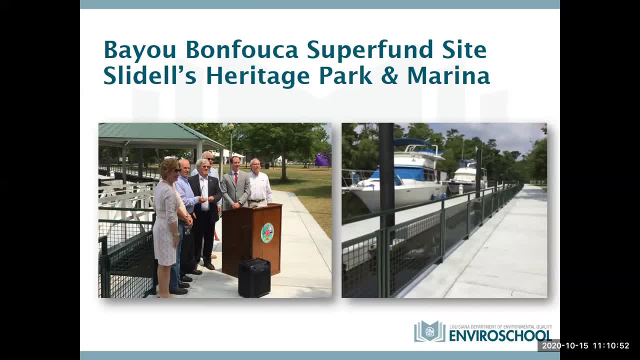 People are always walking there, they have concerts, they have picnics And they also have this great marina that was recently developed. The city got some grant money and they built this wonderful marina facility so that people can bring their boats in from Lake Pontchartrain. 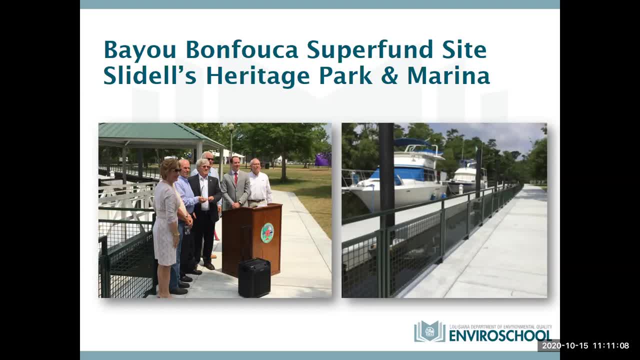 park, at the park, enjoy the park. go to fireworks displays that they have there are concerts, and walk into Old Town, Slidell and you know, go to restaurants and go to craft shops and so forth and enjoy the facilities and businesses. 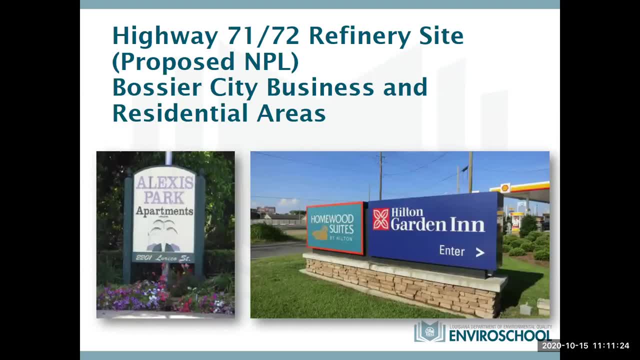 Okay, Next I want to talk a little bit about the Highway 172 refinery site, which is that proposed NPL site, And I don't know if it's so much redevelopment as it was development, Because when we found the site it was pretty much already developed. 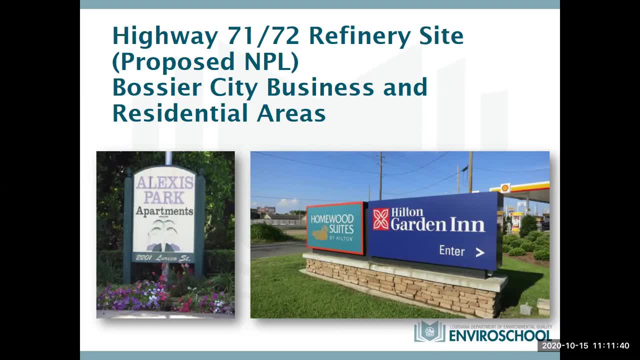 I'll point out. on the left is the Lexus Park Apartments sign, which the Lexus Park Apartments is where the site came to light in the early 1990s. I was familiar with this when it occurred. The Lexus Park Apartments were built on an area of the site that had contaminated groundwater- had hydrocarbons floating on the groundwater. 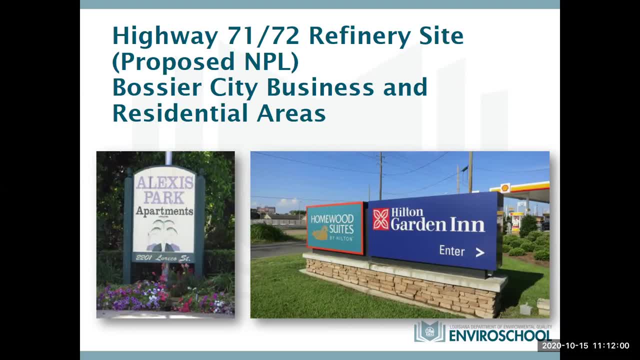 And what happened is the apartment building began to act as a vapor trap for that subsurface vapor, And that vapor trap built up, you know, methane in the walls of the apartments to the point where a fire marshal or you know, went in there and put a combustible gas indicator in the wall of one of the apartments in the downstairs area. 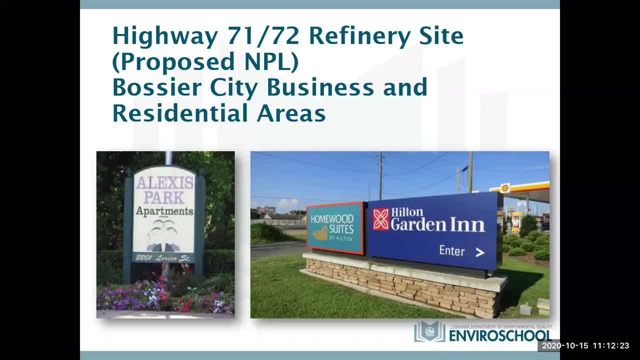 And they got above the lower LEL. That meant, you know, had he been smoking at the time, that he could have blown the whole place to smithereens. So that was how we discovered the site, And then it became NPL. 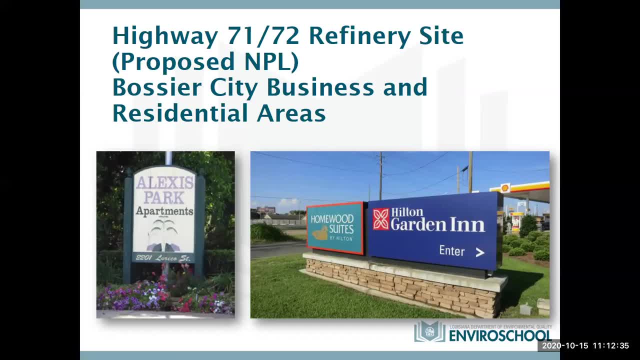 And it's been like I say we're almost, We're almost done with this site, We're very close And some of the things there, of course the Lexus Park Apartments, they've been able to. They moved A by Adam for a while. 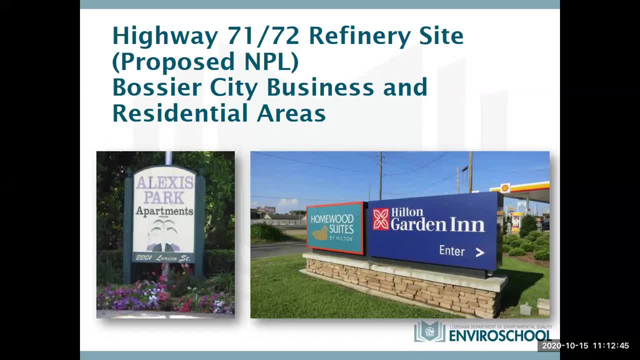 And the lower floors were then uninhabitable. Then, after the cleanup progressed and the situation improved, then people could move back into them And they're fully- you know, fully- occupied at this time. So I guess they've been developed and redeveloped.